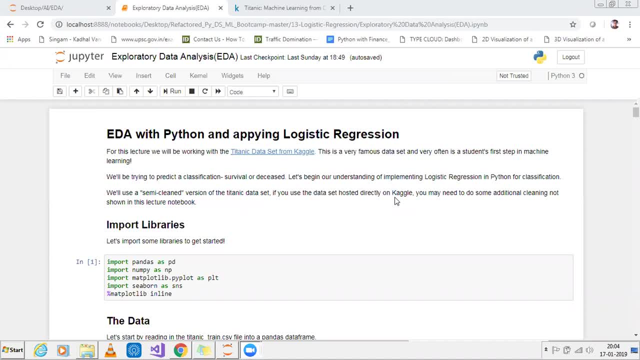 of your time span goes on analyzing your data and actually exploring the data, so it is basically called as exploratory data analysis. That basically means that if you have a data set, you have to be a detective where you need to find out more and more information from that. 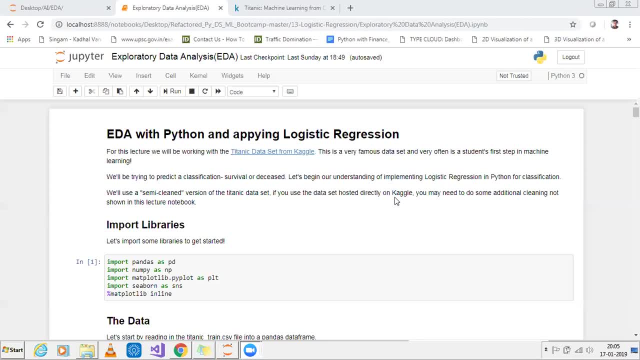 particular data. So this topic is basically: who is actually interested to know more about data pre-processing and to apply different kind of logics, and over here we'll be using libraries like pandas and numpy. very simple function in pandas. we'll be seeing over here and we'll try. 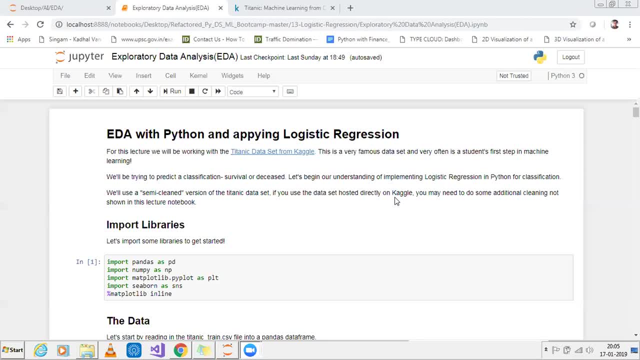 to do the exploratory data analysis Before starting this particular lecture. guys, this session, please subscribe the channel if you have not subscribed, because I do come up with very interesting contents and I try to upload a video each and every day. So, to begin with, over here, the data set that I'll be using is something: 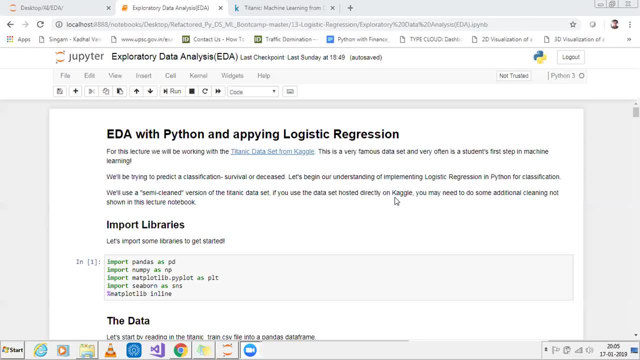 called as titanic data set, and I hope everybody's familiar with titanic data set. if you are not, you can download it from Kaggle, otherwise I'll be trying to. I'll put this particular notebook file along with the data set in the github, which will be provided in the description box. so to begin with, 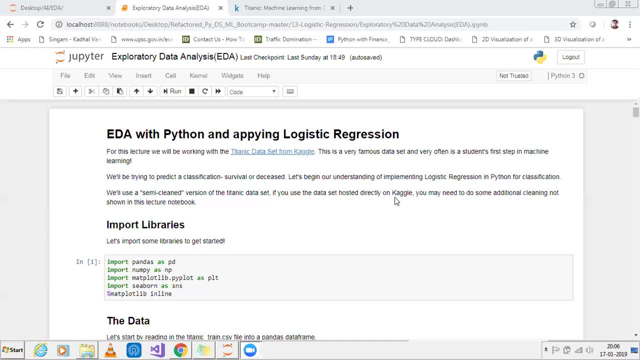 When I am doing the analysis. so what is the main? what, what, what does the data set say? tightening data set? so first we'll discuss about the data set and then, when we are doing a lot of pre-processing steps, we'll try to see that. what are the pre-processing steps that we usually do? 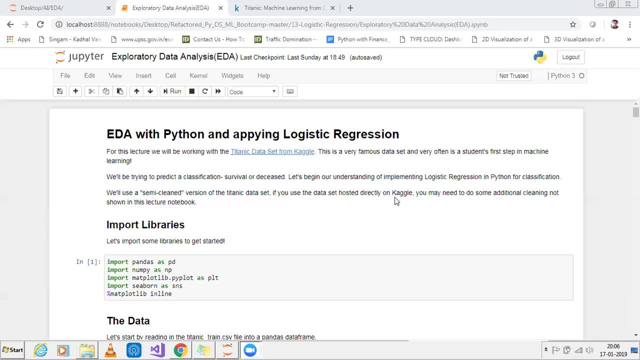 on a particular data set before we give that particular input to our model so that our model will be able to do the prediction. It is very important to know that if we don't do this analysis properly, definitely our model will not give a very good accuracy. 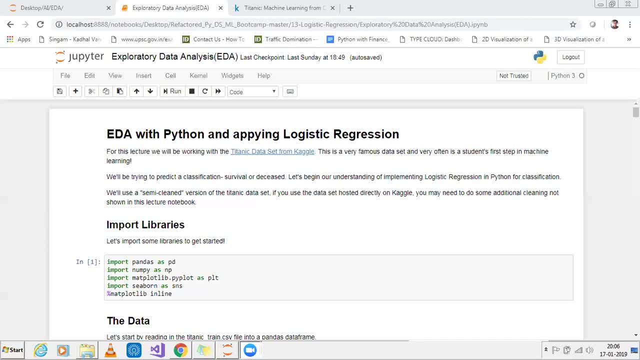 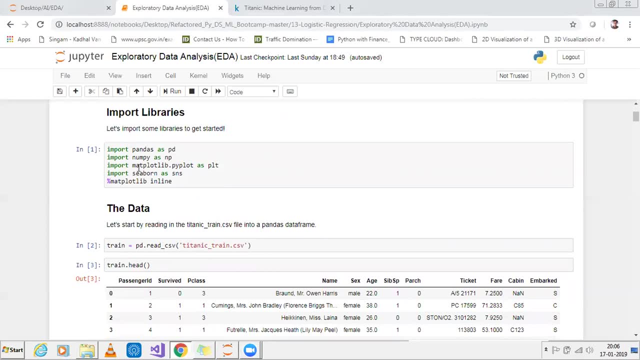 So let us go ahead and start seeing this particular data set and let us see that what of data pre-processing steps will come up with. Initially, I'll be uploading all the libraries which are required, like Pandas, NumPy, Matplotlib, Seaborn, and I'm using this Matplotlib inline so that I'll be able to see my graphs within. 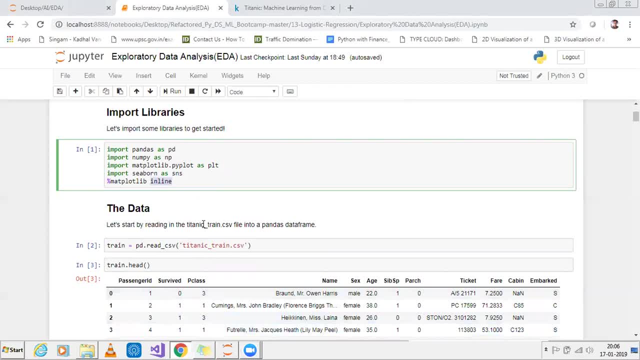 this particular Jupyter Notebook. I think one of the most important thing is that I'm not using a spider IDE over here. Instead, I'm using Jupyter Notebook. The reason is that I need to show you visualization graphs which will be created by using Seaborn. 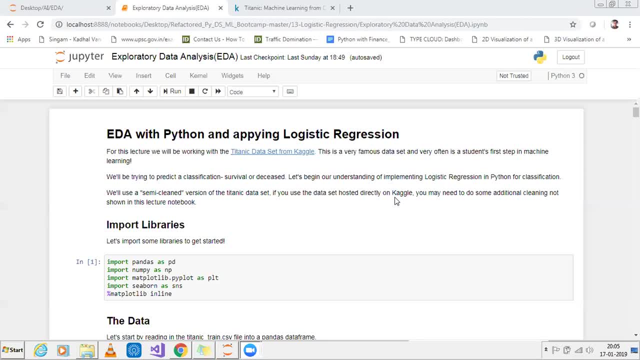 called as titanic data set, and I hope everybody's familiar with titanic data set. if you are not, you can download it from Kaggle, otherwise I'll be trying to. I'll put this particular notebook file along with the data set in the github, which will be provided in the description box. So to begin with, when I am doing the analysis. so 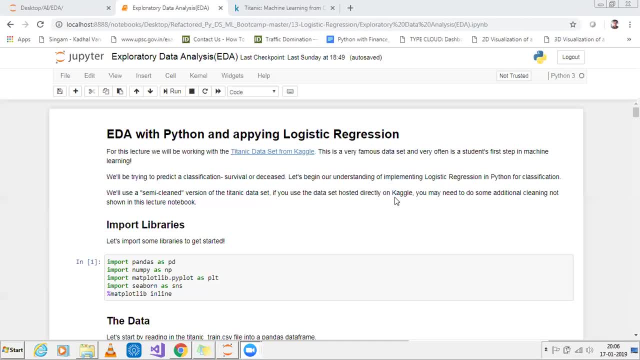 what is the main? uh, what, what, what does the data set say? titanic data sets. first we'll discuss about the data set and then, when we are doing a lot of pre-processing steps, we'll try to see that what are the pre-processing steps that we usually do on a particular data set before we give. 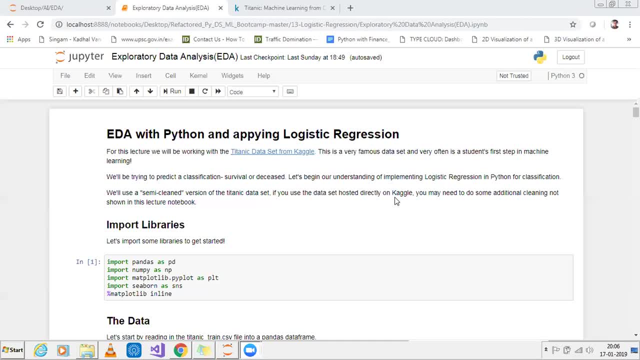 that particular input to our model so that our model will be able to do the prediction. It is very important to know that if we don't do this data analysis properly, definitely our model will not give a very good accuracy. So let us go ahead and start seeing this particular data set and let us see that. what of 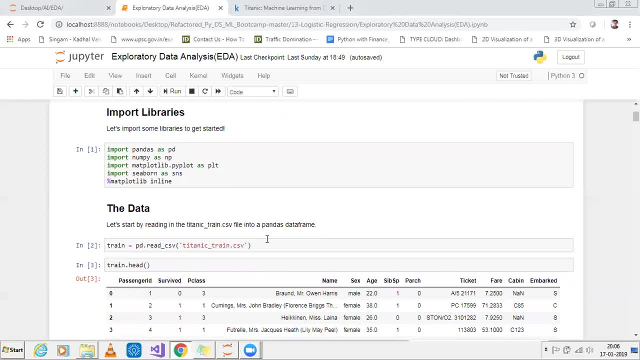 data pre-processing steps will come up with. Initially, I'll be uploading all the libraries which are required, like pandas, numpy, matplotlib, seaborn, and I'm using this matplotlib inline so that I'll be able to see my graphs within this particular Jupyter notebook. I think one of the 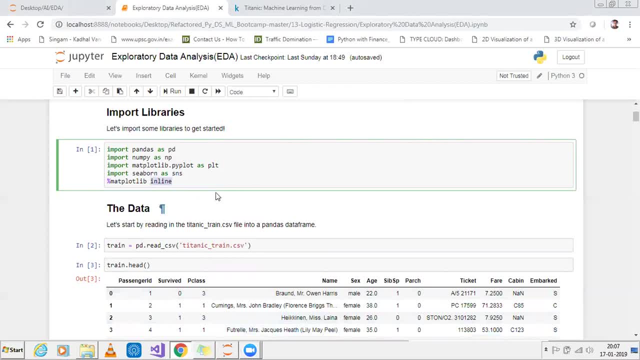 more. most important thing is that I'm not using a IDE over here. instead, I'm using Jupyter notebook. The reason is that I need to show you visualization graphs which will be created by using seaborn. So that is the reason why I'm trying to implement. 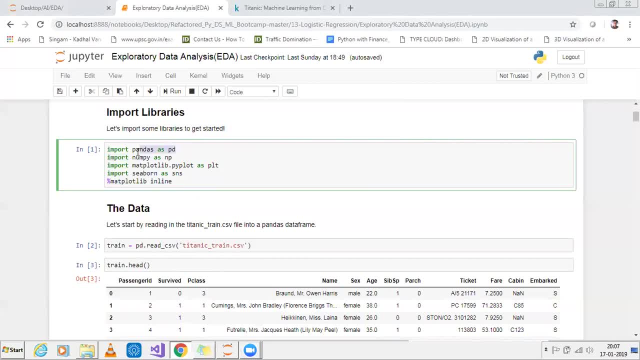 this in Jupyter notebook, So I hope everybody knows what pandas library does. it helps you to read the data set and most of the data pre-processing steps will be done by the inbuilt function that is present inside pandas. Then numpy is basically used to work with arrays. 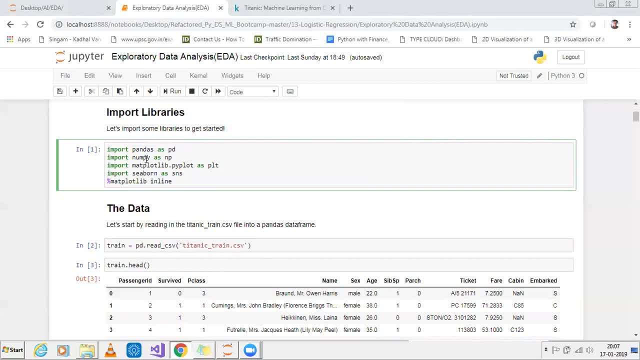 it may be a multi-dimensional arrays or a single dimensional array- matplotlib. it will be used for visualization, seaborn will also be used for visualization, and seaborn will also consist of various statistical concepts, statistical functions, which will help you to visualize the data properly. So, to begin with, I'm going to 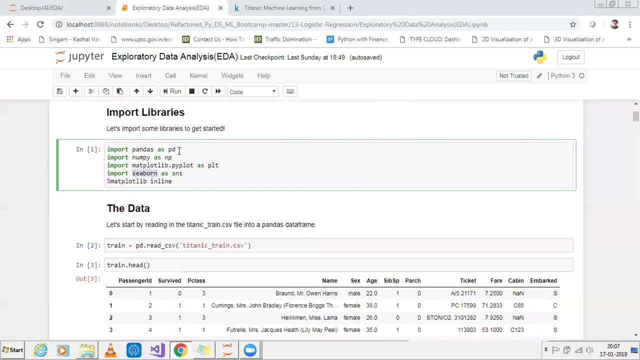 So that is the reason why I'm trying to implement this in Jupyter Notebook, So I hope everybody knows what Pandas library does. It helps you to read the data set, and most of the data pre-processing steps will be done by the inbuilt function that is present inside Pandas. 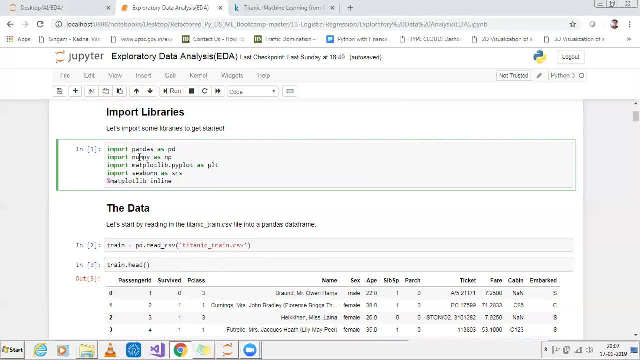 Then NumPy is basically used to work with arrays. So I'm going to show you how to do that. So I'm going to show you how to do that. So I'm going to show you how to do that. It may be a multi-dimensional array or a single-dimensional array. 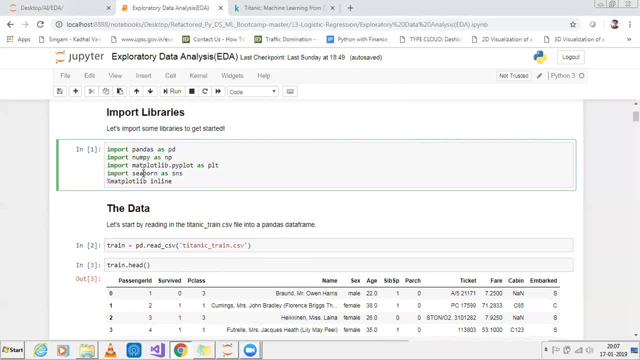 Matplotlib. it will be used for visualization, Seaborn will also be used for visualization, And Seaborn will also consist of various statistical concepts, statistical functions, which will help you to visualize the data properly. So, to begin with, I have downloaded the data set and the data set looks something like: 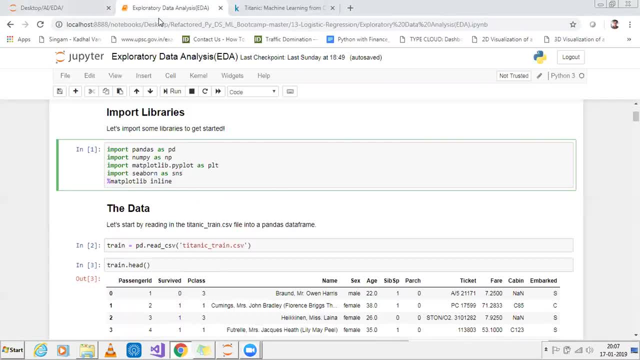 this titanic-traincsv, So I'll try to read the data set by using Pandas. So I'll write pdread-csv and I'm going to. Now let me just discuss about some of the columns that are present inside this. 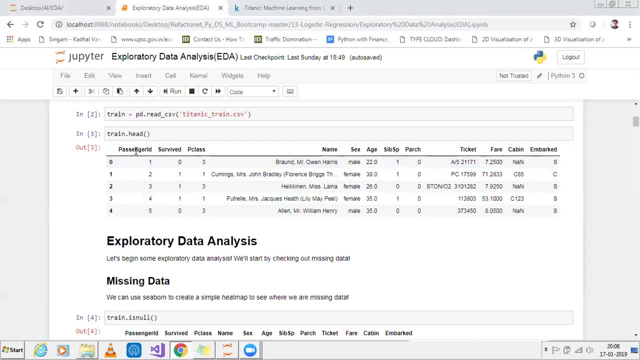 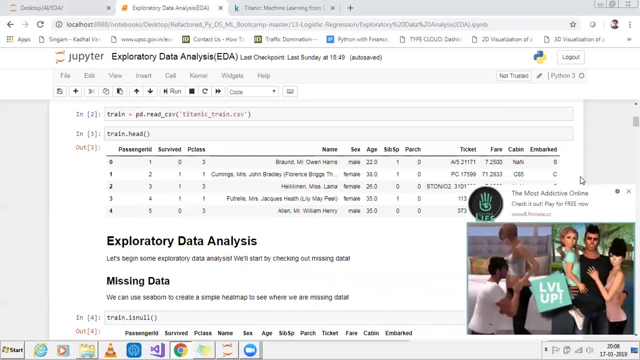 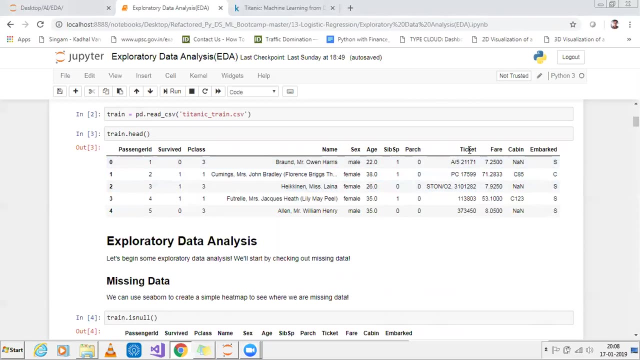 So when I see the head part of this particular data set, I have different information like passenger ID, survivor, passenger class, name, sex, age. This sib is basically called a sibling spouse- yeah, And this is PR is basically called as parent-child. and ticket fare, cabin and embark. 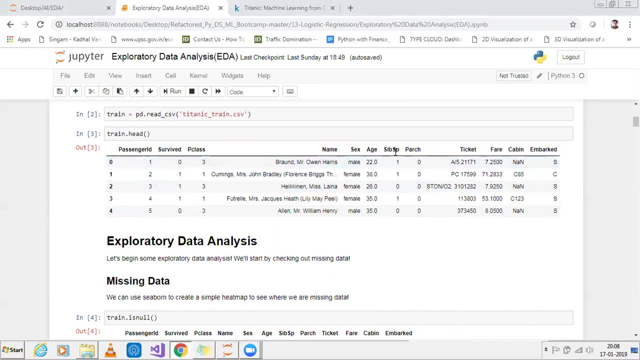 Let me just go and explain you about this particular column because it looks confusing. This is basically called a parent, child and ticket fare, cabin and embark. Let me just go and explain you about this particular column because it looks confusing. This is basically the count of spouse and the sex total count of the spouse and siblings. 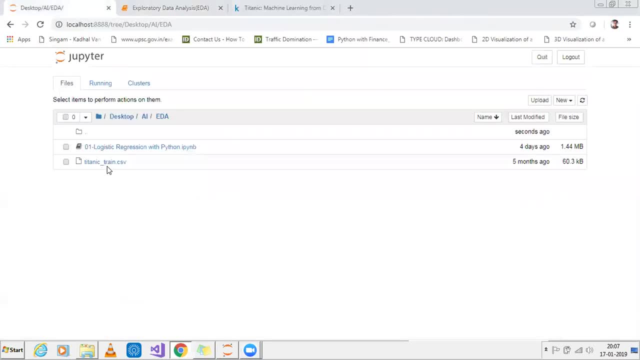 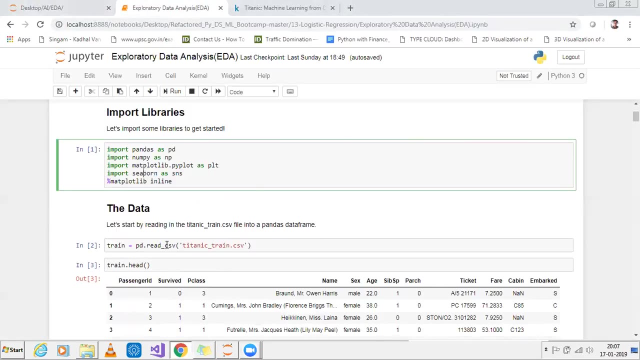 I have downloaded the data set and the data set looks something like this: titanic underscore train dot csv. so I'll try to read the data set by using pandas. so I'll write pd dot read underscore csv and I'm going to read the titanic underscore train dot csv. Now let me just discuss about some. 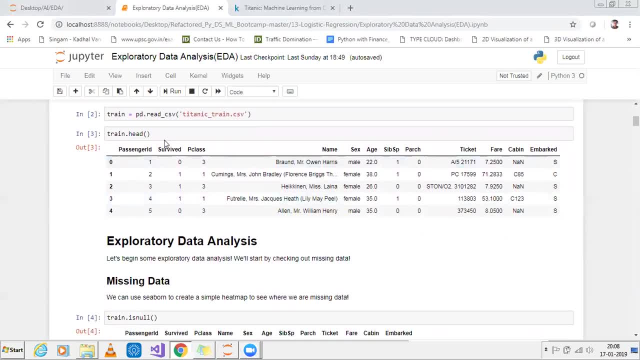 of the columns that are present inside this. so when I just see the head part of this particular data set, I have different information like passenger id, survived passenger class, name, sex age. this sib is basically called a sibling spouse. yeah, and this is p arc is basically called as: 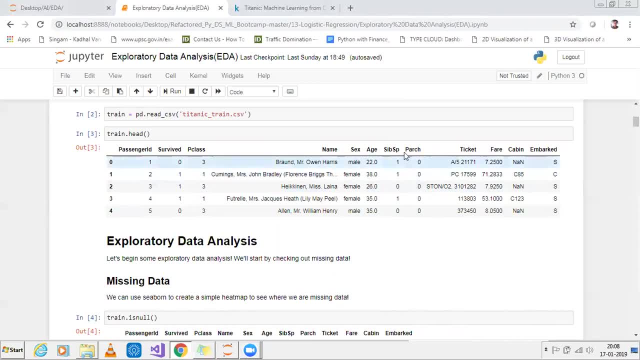 parent, child and ticket fare. cabin and embark. let me just go and explain you about this particular column because it looks confusing. this is basically the count of spouse and the total count. this is the total count of the children and the parents and this is basically the ticket information. 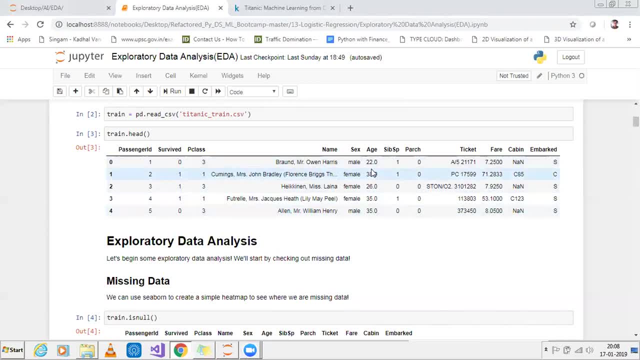 so this is the basic information about this data set, and the main aim of this data set is that we need to predict, based on this information that we have, whether the passenger has survived or not. so that is the main problem statement behind it. I hope everybody is familiar with titanic movies. 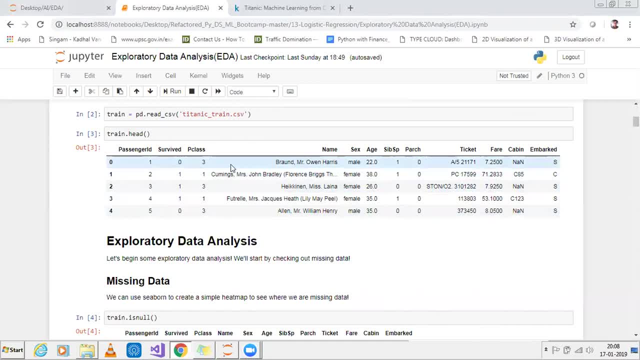 right over there. we have this particular information. now we need to predict whether the passenger has survived or not. so I'll just try to show you how to predict whether the passenger has survived or not. so to begin with your data pre-processing technique. first of all, you need to find out how many nan 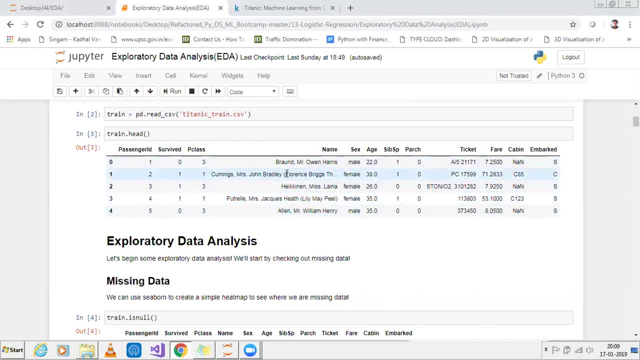 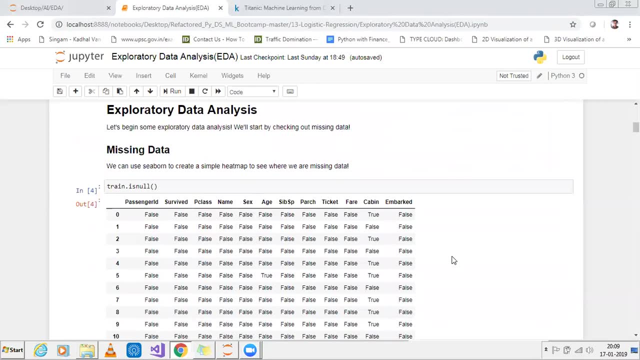 values are present. nan values basically means that how many null values do I have in this particular data set? so the first thing is that I'll try to find out what is the missing data in this particular data set. so, in order to find it, you just what you do. is that so my train? 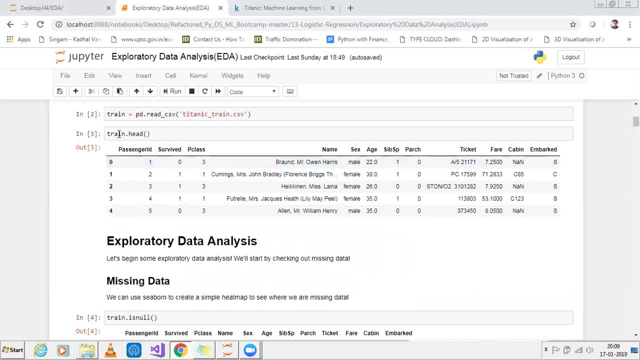 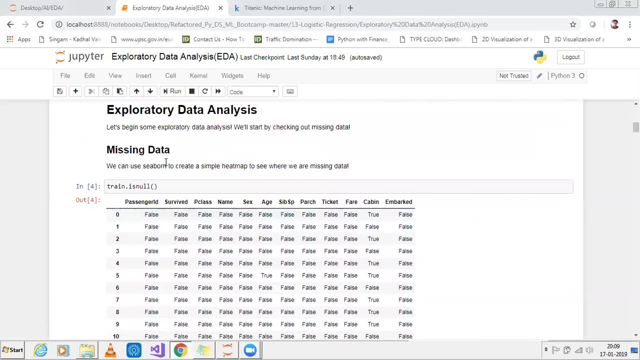 my data set name is basically train. you can see over here this is my train data set, right? so what I'm going to do is that I'm going to first of all check how many missing data sets I have, so that I'll be using an inbuilt function which is present in pandas: bet hosting. 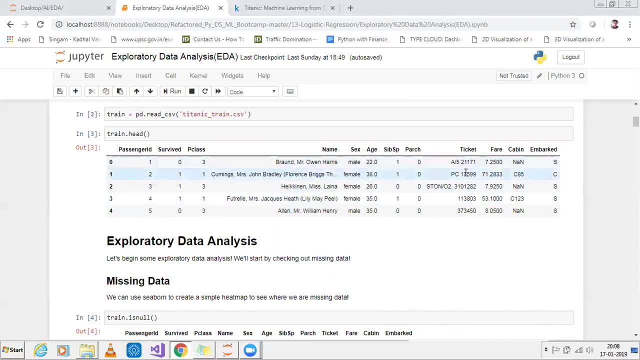 This is the total count of the children and the parents and this is basically the ticket information. So this is the basic information about this data set, and the main aim of this data set is that we need to predict, based on this information that we have, whether the passenger has survived. 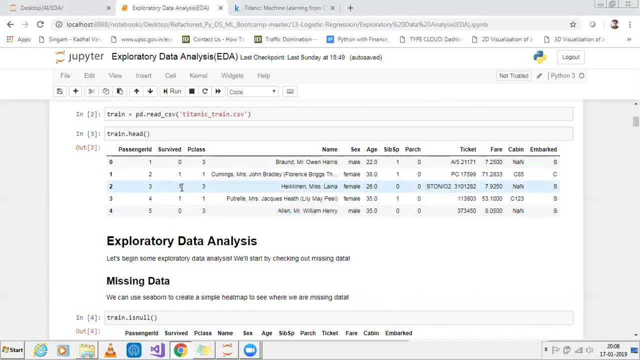 or not. So that is the main problem statement behind it. I hope everybody is familiar with titanic movies right Over there. we have this particular information. Now we need to predict. We need to predict whether the passenger has survived or not. 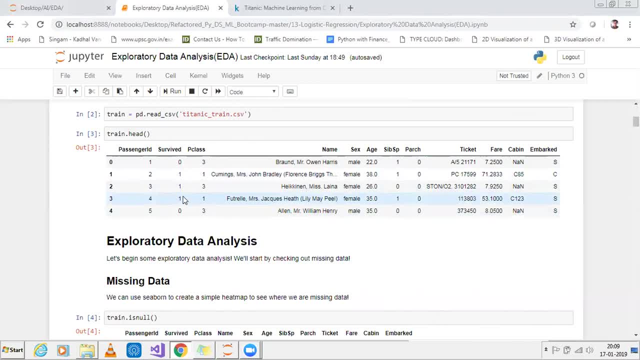 So always to begin with your data preprocessing technique, first of all you need to find out how many NAND values are present. NAND values basically means that how many null values do I have in this particular data set? So the first thing is that I'll try to find out what is the missing data in this particular 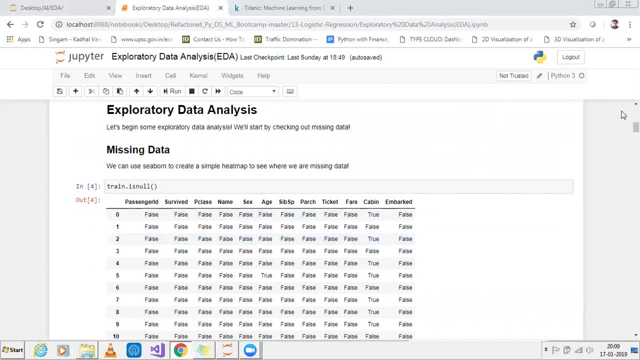 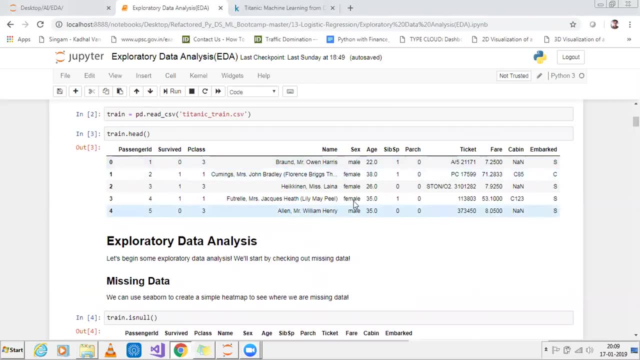 data set. So, in order to find it, you just what you do is that? so my train, my data set name, is basically train. You can see over here. this is my train data set, right? So what I'm going to do is that I'm going to first of all check how many missing data. 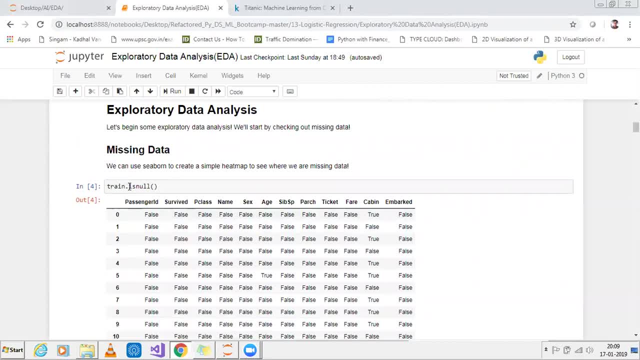 is there. So for that I will be using an inbuilt function which is present in Pandas- sorry- within a data frame that is called trainisNull. So isNull helps you to find out whether each and every value in each and every row is either. 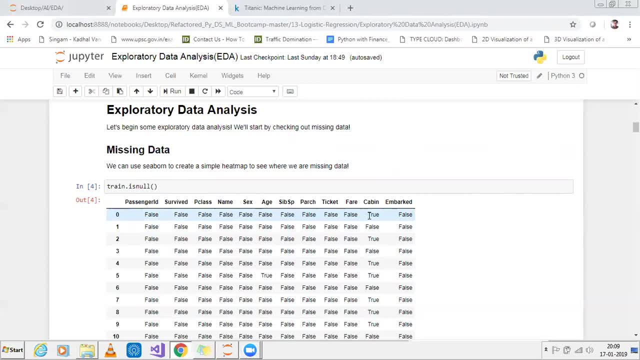 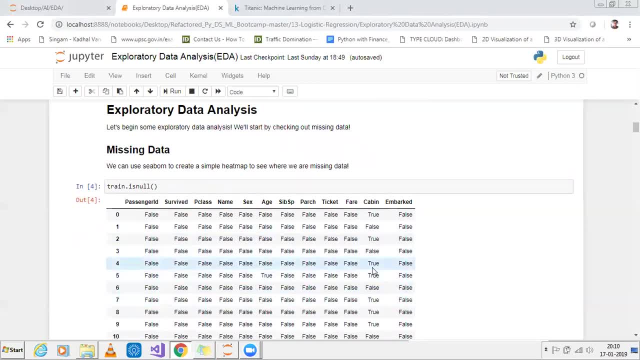 So, similarly, there are many columns, many rows, which will be giving you true and false right. But is this a good way of seeing or finding the null values, right? It becomes difficult because if I have a million data sets, you know. 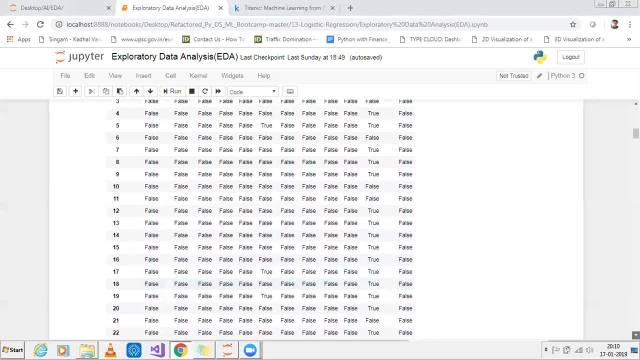 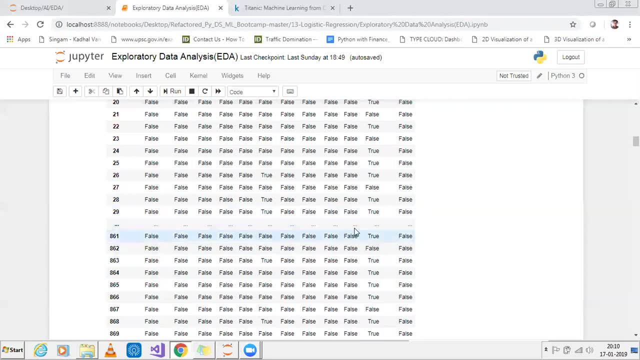 or just consider a thousand data sets. I have to scroll down all and try to see. And Jupyter Notebooks also does not give the whole information. It skips some of the rows away. You can see this. So in order to do that, I'll be using a visualization concept. 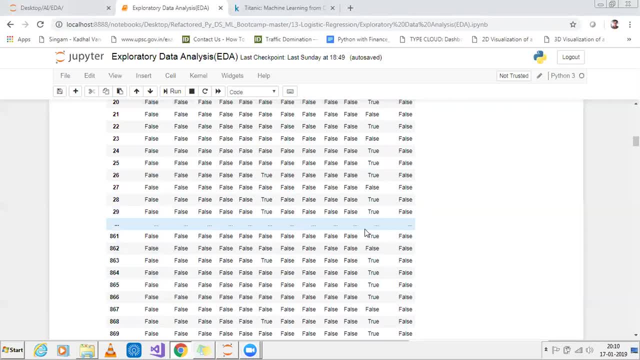 which is introduced in Seaborn, which is through an inbuilt function which I'll prove to explain to you in a while. With that, we'll be able to see that how many null values are there and how many null values are not there. 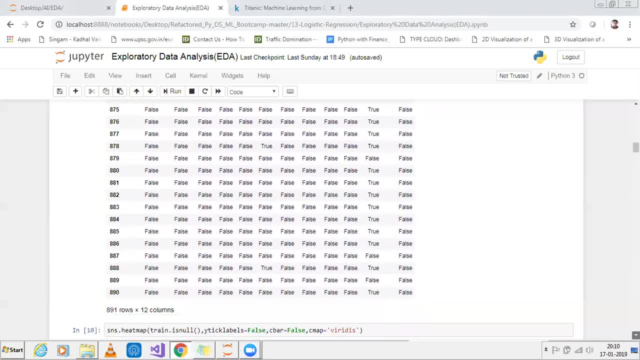 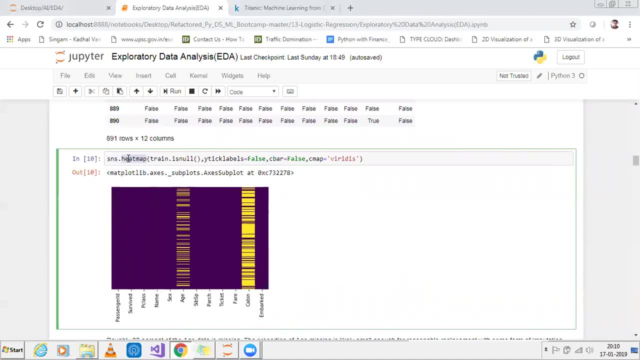 So to do it I'll be using a Seaborn library. So Seaborn I have actually imported as SNF. So there is a heat map concept. This heat map actually helps you to see that whatever condition that you're putting over here, 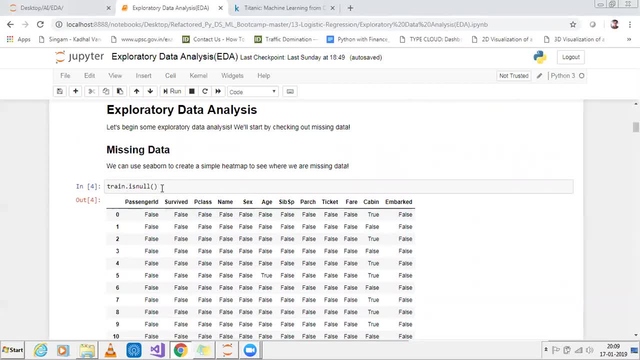 within a dataprint that is called a trainis null, so is null- helps you to find out whether each and every value in each and every rows is either true or false. if it is true, that basically means that value is null. so you can see over here in the first record I have this cabin value as true. so if I go and see in the top or in my head section, then see that. my cabin value is true and my truck is matching that value, but this one has got trigonometric information over here. but this one also has trigonometric information over here and now. that won't be important to this, because there are a lot of allows that, even though I see a lot of values. 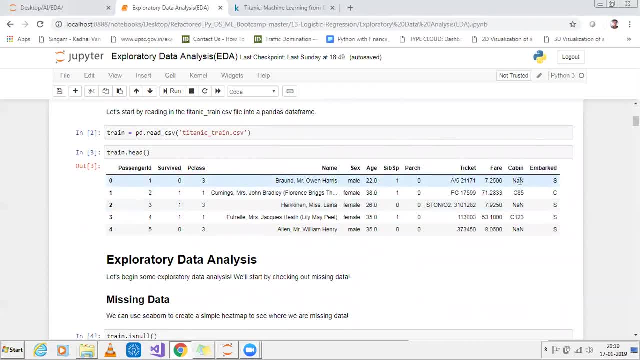 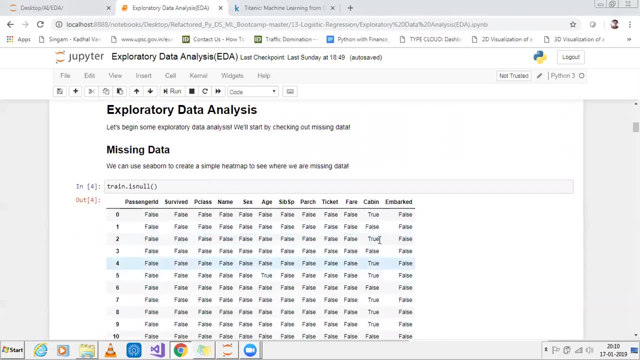 So that's because we just want to get that check. as you can see over here, like, for example, we have got all right, or whatever section, you can see that my cabin is having the nan value in the first record, so that is the reason why it is giving you a value called a true code. so, similarly, there are many columns, uh many. 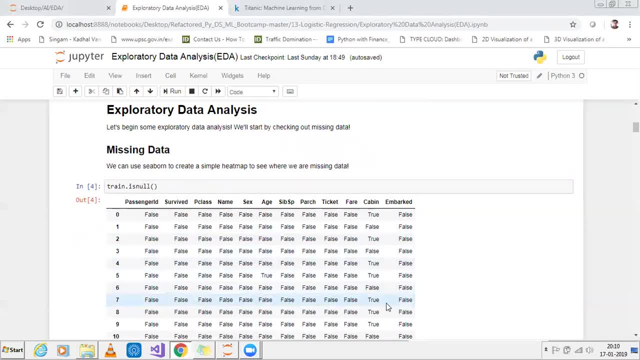 rows, which will be giving you true and false, right. but is this a good way of seeing or finding the null values, right? it becomes difficult because if i have million data set, you know, or just consider thousand data set, i have to scroll down all and try to see. and jupyter notebooks also does not. 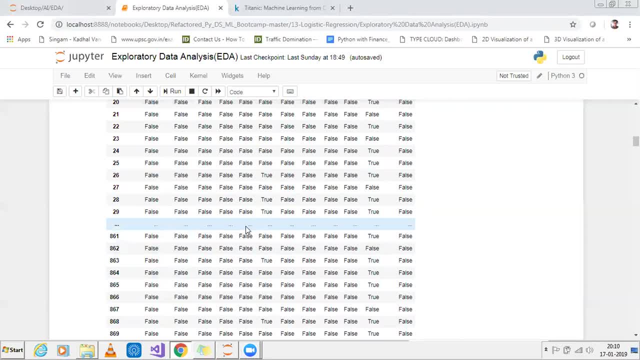 give the whole information. it skips some of the rows over. here you can see this. so in order to do that, i'll be using a visualization concept which is introduced in c-bar, which is through n-grid function, which i'll prove to explain you in a while. with that, we'll be able to see that how. 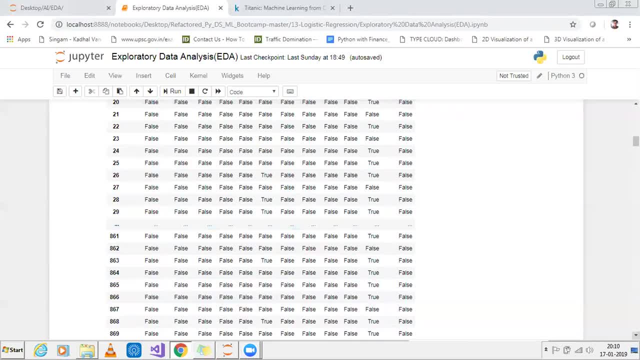 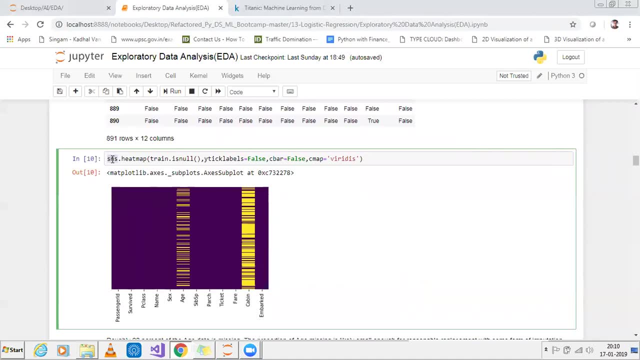 many null values are there and how many null values are not there. so to to do it, i'll be using a c-bar library. so c-bar i have actually imported as sns. so there is a heat map concept. this heat map actually helps me to see that whatever condition that you are putting over here and whichever is true, that will be. 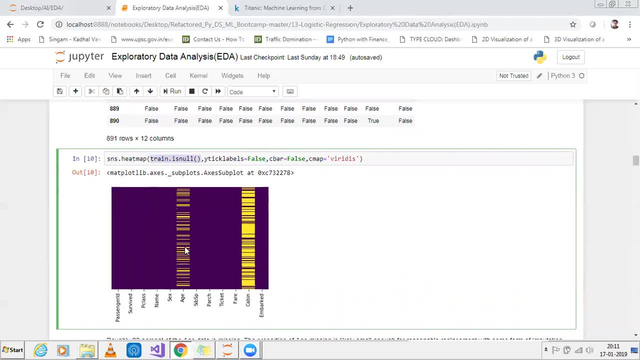 actually, you know, displayed in this, in another, you know, in another color, or it will be visualized in such a way that that will be differentiated from, differentiated from that particular condition. so if i write train dot is null, so it is going to check this condition in this particular heat map. 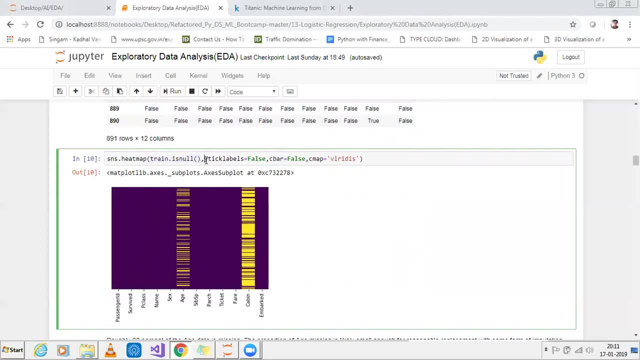 here are some of parameters that i want to show, such as white tick labels. okay, now, when i say white tick labels as false, so i have two axes, one is x-axis and one is y-axis. so when i take x-axis, since my x-tick label 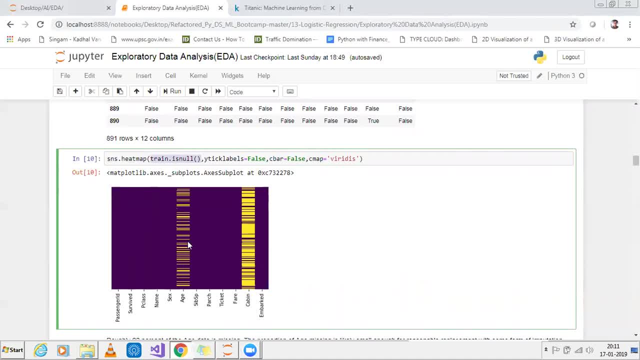 and whichever is true, that will be actually, you know, displayed in another color or it will be visualized in such a way that that will be differentiated from that particular condition. So if I write trainsnl, so it is going to check this condition in this particular heat map. 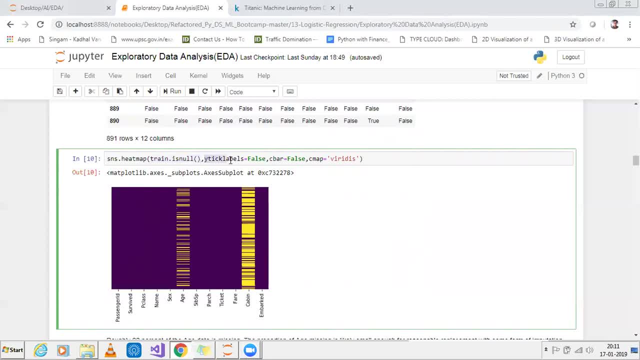 Here are some of the parameters that I want to show, such as y-tick labels. Okay, Now, when I say y-tick labels as false, so I have two axes, One is x-axis and one is y-axis. So when I take x-axis, 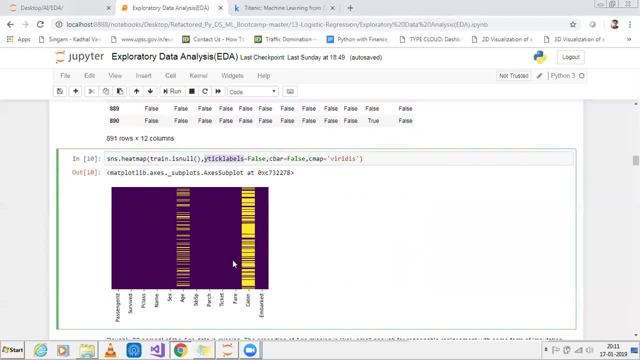 x-tick label. x-ticks label is not false, right? So I can see all my x values over here, which is my column name. So this is all my column name. passenger ID: survived, key class name, sex age. 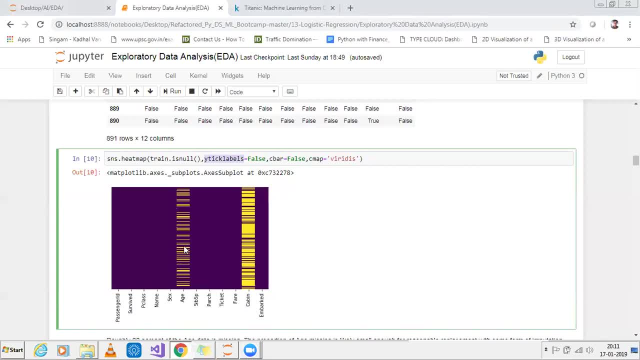 sibling spouse, parent, child, ticket pair, cabin and embark. But I try to put y-tick labels as false. Y-tick label basically means that this is my record information, So it will be record zero. record one, record two, record three based on the index number. 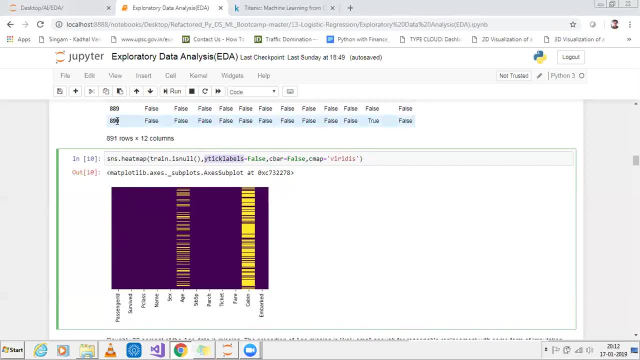 So I can see over here, I have total two, So this is basically 891 posts. So this is basically 891 records. So what we can do is that, if I, if I, if I have a parameter which is called an x-tickable. 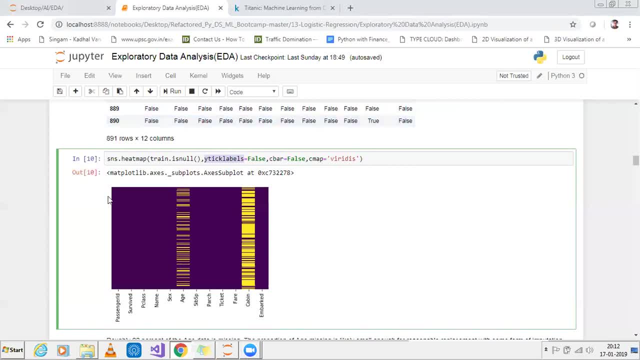 x-tick label is equal to true. If I set it, all my indexes will come over here. but I'm not that much interested over here. I just want to see that in which all columns I have nan values. Then there are some more styling which is called a cbar and cbar also I'm minting in test false. 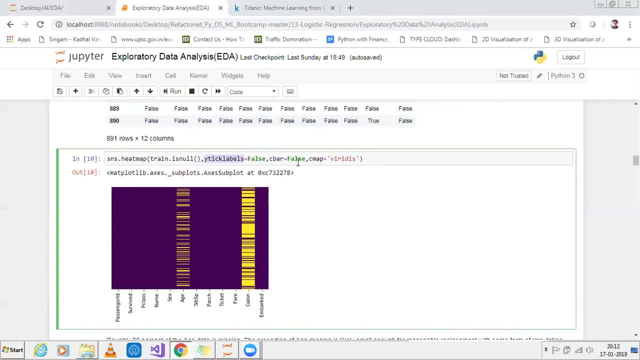 And there is some styling called a cmap. So this is not important. You can just keep this- two parameters- And you can just display this heat map. Now, in this heat map there is no specific thing, that all the null values is shown in yellow color. 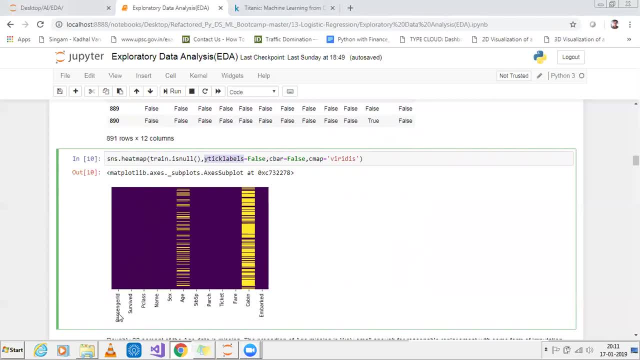 x-ticks label is not false, right? so i can see all my x values over here, which is my column name. so this is all my column name. passenger id: survived, key class name, sex, age, sibling, spouse, parent, child, ticket pair, cabin and embark. but i try to put white tick labels as false white tick label basically. 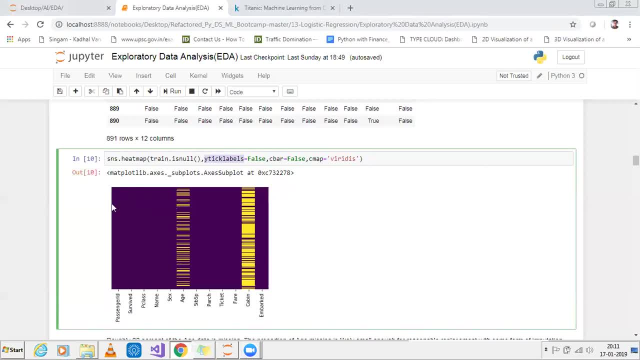 means that this is my recording function, so it will be record zero: record one, record two. report three: based on the index number. so i can see over here i have total two, two, ninety one, eight ninety one posts. so this is basically eight ninety one reports. so what we can do is that, if i, if i, if i, 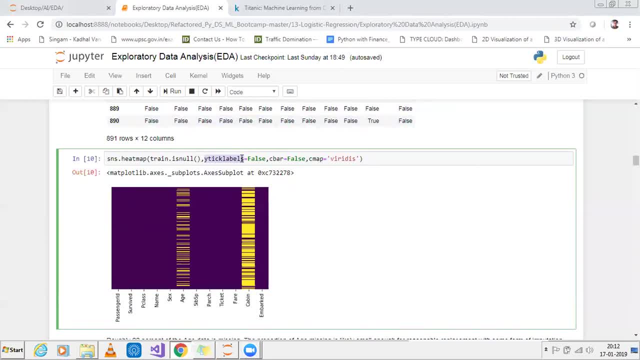 have a parameter which is called as x tickable. x tick label is equal to true. if i set it, all my indexes will come over here. but i am not that much interested over here. i just want to see that in which all columns i have man value. 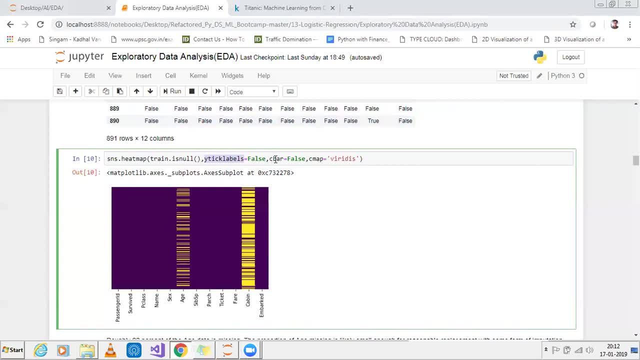 then they are some more styling which is called a C bar, and C bar also I'm inting in test files, and there is some styling called a C map where it is. so this is not important, you can just keep this two parameters also, and you can. 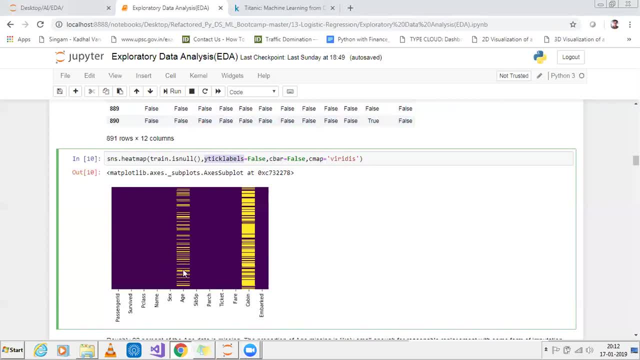 just display this heat map now. in this heat map there is no specific thing, that all the null values is shown in yellow color, and this styling has come from the C map that I have used, which is called as we read it now because of this particular style. you can see that we are having yellow colors over here for the 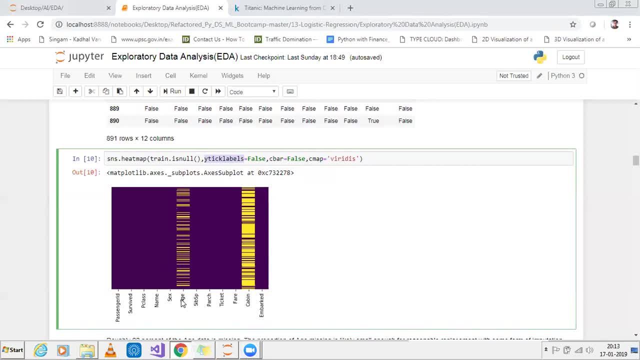 nan values. so most of the nan values are present in H cabin. so most of the nan values are actually present. now, this will actually give you more information: that which all column is having more nan and now, in order to handle it, we will see that what all techniques will be used. okay, now let us. 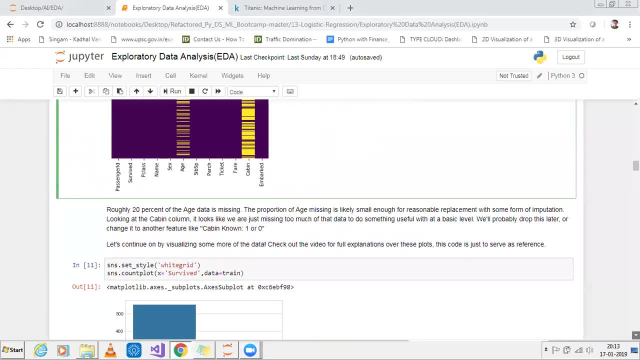 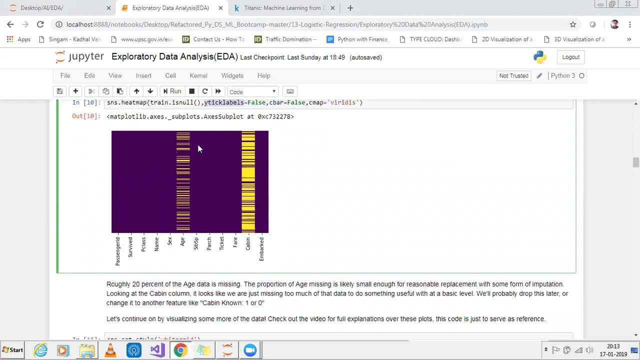 go and see that, how we can actually handle this nan values. okay, so what I'm going to do is, first of all, I'm going to visualize this data properly. I'm going to visualize, I try to get more and more information from this data and then I'll try to replace this nan value with something else, which is: 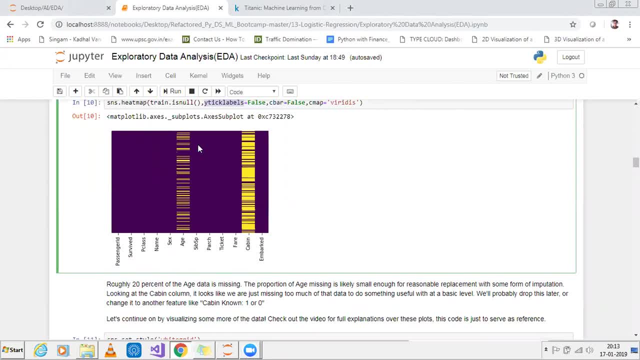 very much suitable. and again I'm going to use some of the statistics concepts and based on that statistics concept, I'm again going to visualize by using C bar, so from here we can make some observation- that roughly 20% of our age data is missing. okay, just randomly, if you just see the proportion of the 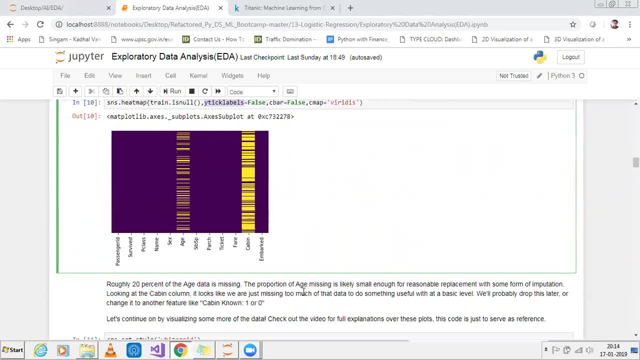 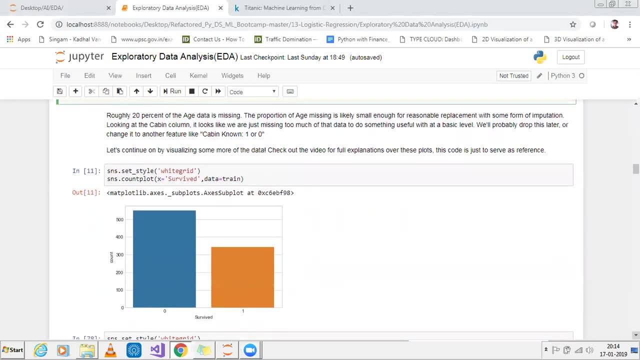 proportion of age missing is likely small enough for reasonable replacement. so you can read this, all the kind of observation. okay, now let's see how. what all information can I do? now again, I will be using C bar. I'll be setting a style called as white grid. white grid basically says you that over here in the 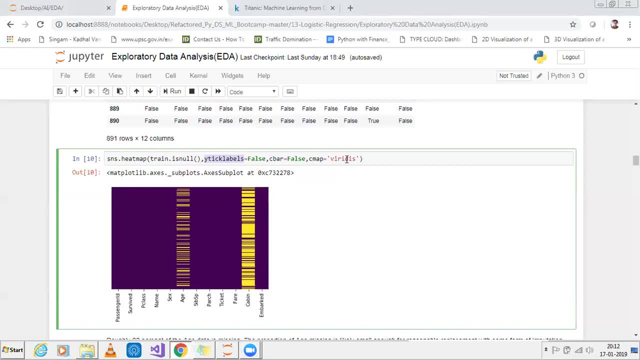 And this styling has come from the cmap that I've used, which is called as viridian. Now, because of this particular style, you can see that we are having yellow colors over here for the nan values, So most of the nan values are present in H cabin. 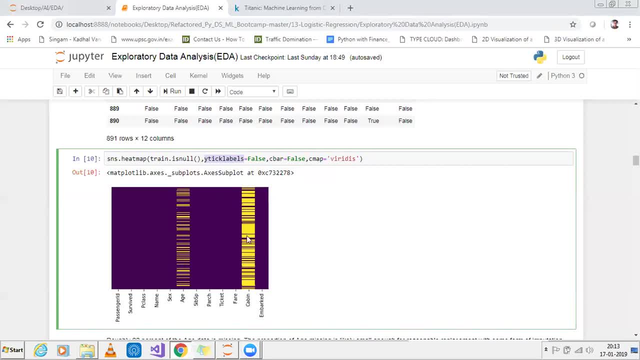 So most of the nan values are present in H cabin. So most of the nan values are present in H cabin. These are actually correct problems. And now, in order to handle it, we'll see that what our techniques will be used. And now, in order to handle it, we'll see that what our techniques will be used. 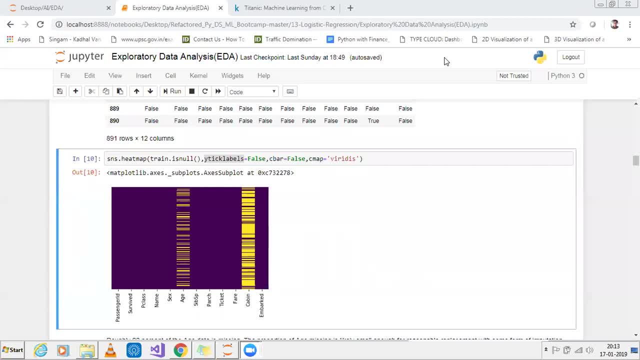 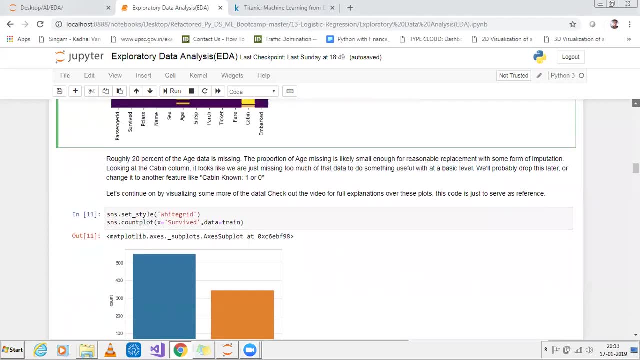 OK, Now let us go and see that, how we can actually handle this nan values. So what I'm going to do is, first of all, I'm going to visualize this data properly. I'm going to visualize, I try to get more and more information from this data. 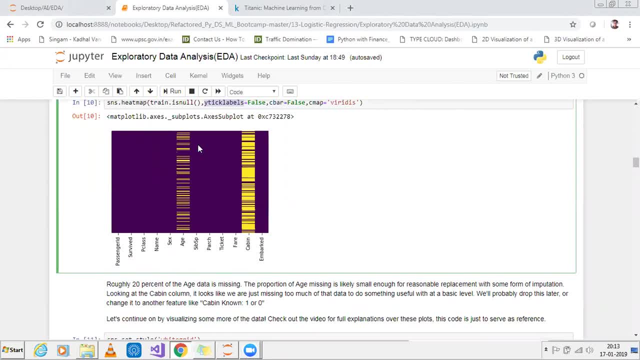 And then I try to replace this nan values with something else, this nam value with something else which is very much suitable. and again i'm going to use some of the statistics concepts and based on that statistics concept, i'm again going to visualize by using c. 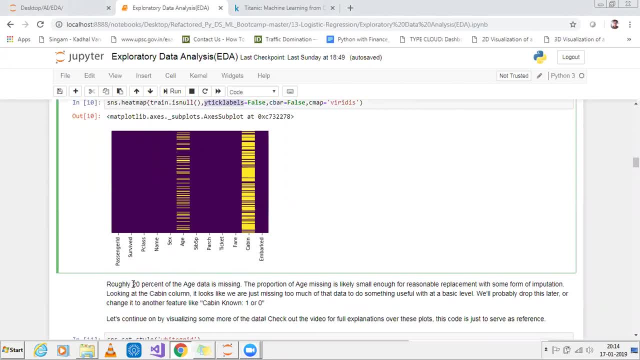 bar. so from here we can make some observation that roughly 20 percent of our age data is missing. okay, just uh, randomly, if you just see, the proportion of the proportion of age missing is likely small enough for reasonable replacement. so you can read this, all the kind of observation. 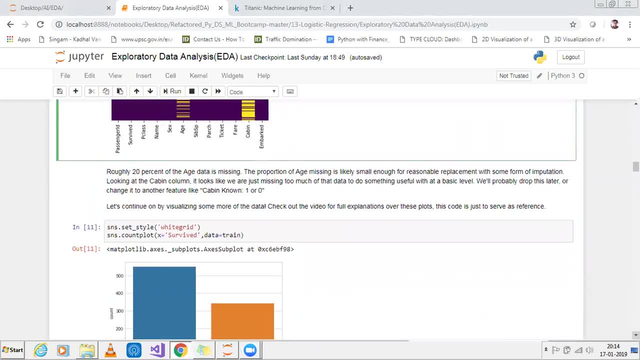 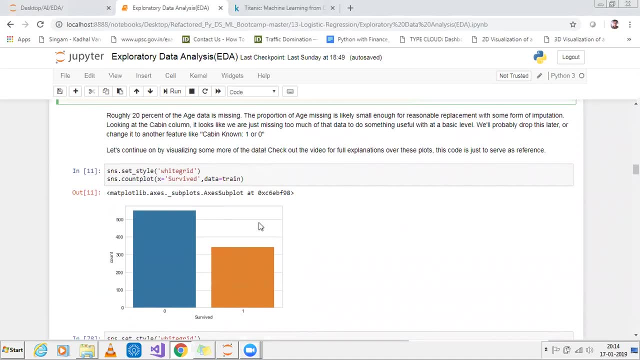 okay, now let's see how. what all information can i do? now again, i will be using c bond. i'll be setting a style called as white grid. white grid basically says you that over here in the back end you can see that there is something like a white boxes right in white. now i'll i'll try to make a. 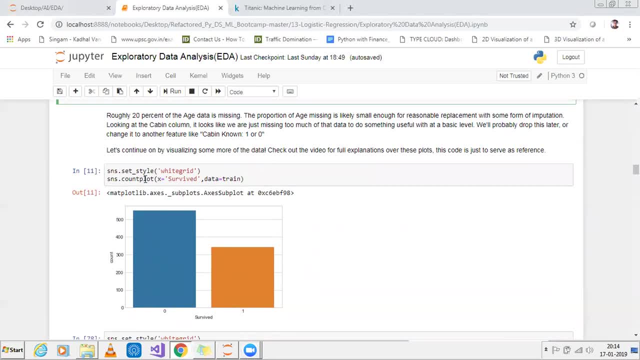 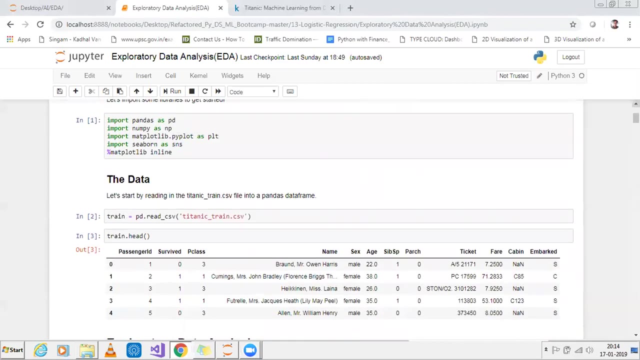 counter plot. so this is basically a counter plot and based on the survive column, i'm going to find out how many. so suppose, if my survive value is zero, you can see over there if i go up, if i go up and see my data set right: survived zero basically means that the person did. 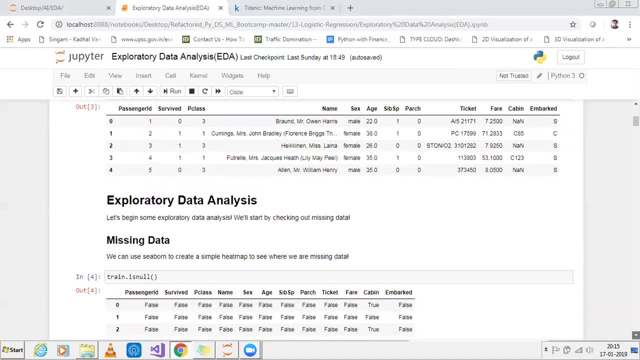 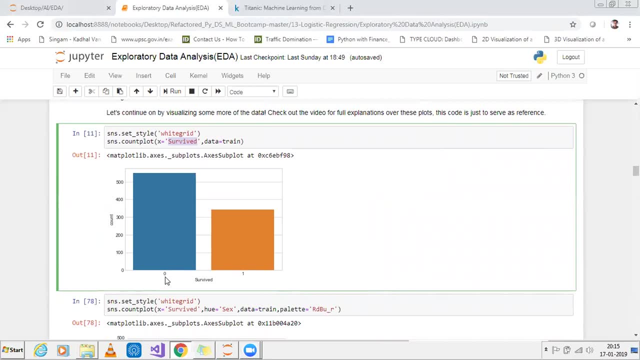 not survive, whereas survive one basically means that the person survived. so what i'm going to do is that, based on this survive column, i'm going to plot a counter plot. so whenever i see, survive is equal to zero. so here the counter plot actually helps you to see that. what is the count of the? 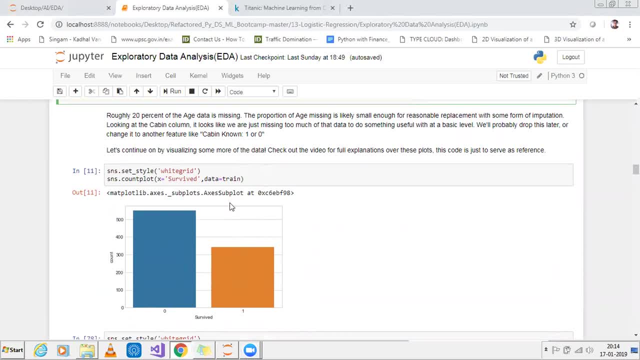 back end you can see that something like a white boxes. right now I'll try to make a counter plot. so this is basically a counter plot and based on the survive column, I'm I'm going to find out how many. so suppose, if my survive value is zero, you can see over. 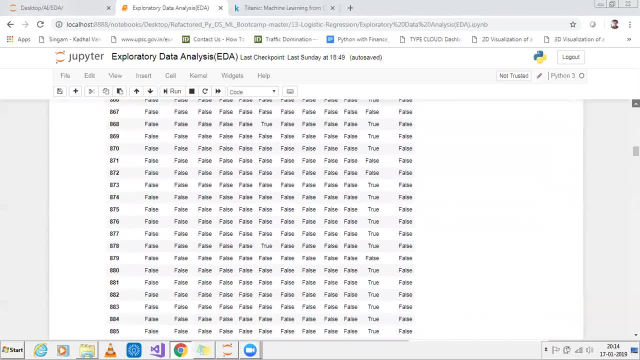 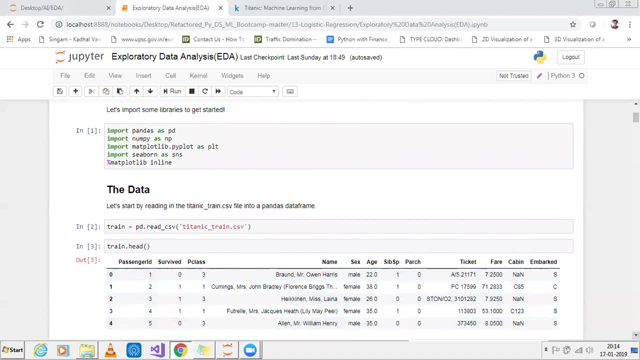 there, if I go up, if I go up and see my data set right, Survived zero basically means that the person did not survive, Whereas survive one basically means that the person survived. So what I'm going to do is that, based on this survive column, I'm going to plot a counter. 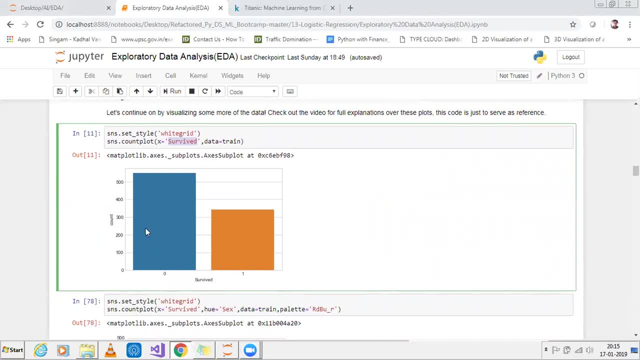 plot. So whenever I see survive is equal to zero. So here the counter plot actually helps you to see that what is the count of the person who did not survive from that 891 reports, whereas what is the count for the person who has actually survived? 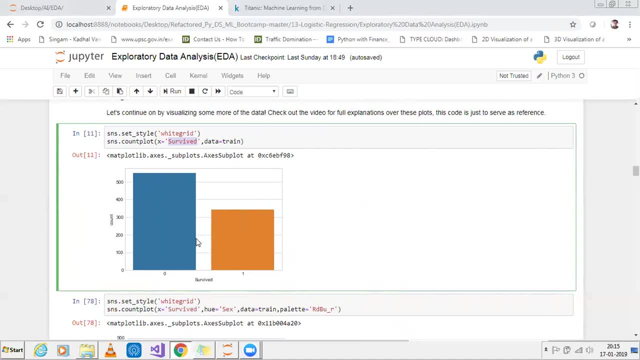 Now you can see that most of the people- more than 550 people- has not survived this particular Titanic accident right, Whereas there were some people around, more than 300, those people actually survived. So this is some information I'm trying to gather from the data set. 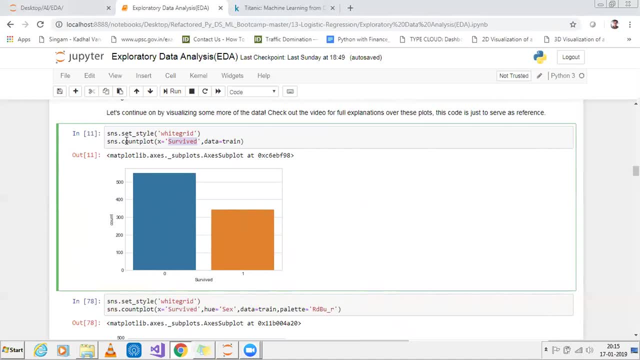 And here I'm using the C1, very important library guys, which will actually use a lot of statistics concepts within it And it will try to show you in a visualized way. Now, fine, I can see, we have survived zero and one. 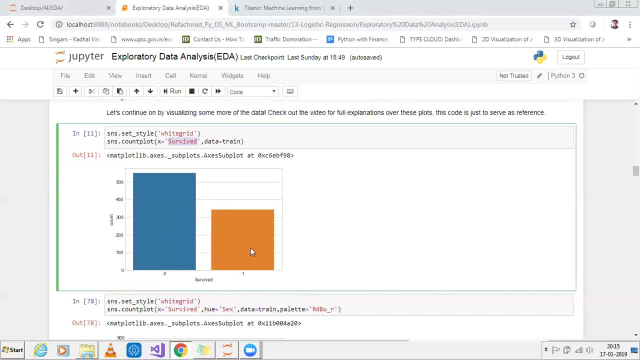 Many people have not survived and many people have less people have survived. Now, based on the survival rate. can I just differentiate this with a sex like male and female? How many people, how many males survived? How many females survived? So let us go and use the same C1 technique. 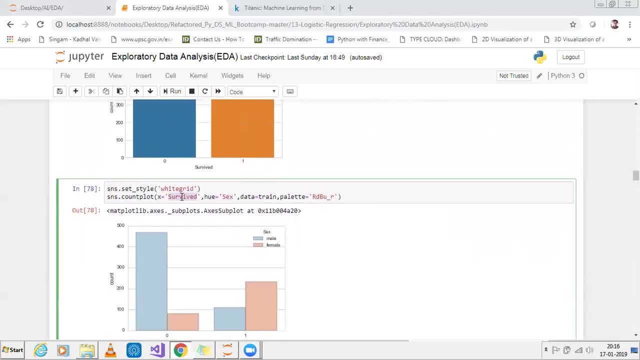 Now I'm going to use the counter plot Here. my X axis is actually having the survive column, but there is one more parameter, which is called a hue Hue. This hue will be, you know, divided based on the survive column, based on sex column. 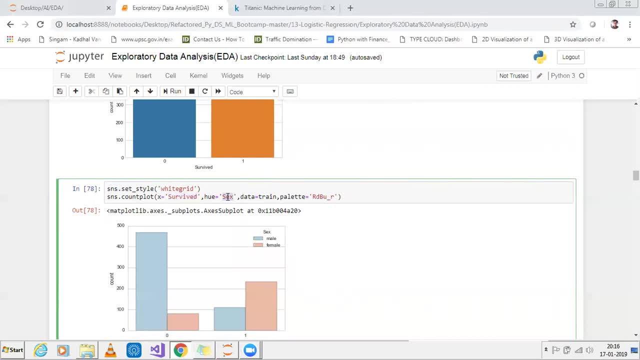 So sex, I have basically two: One is a male and female. Okay, I'm going to use the data that is, my trained data set, And this palette is just used to give your, uh, some some good colorful visualization, So I'm using this. 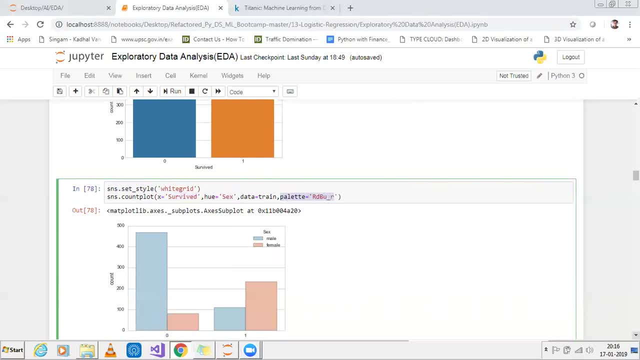 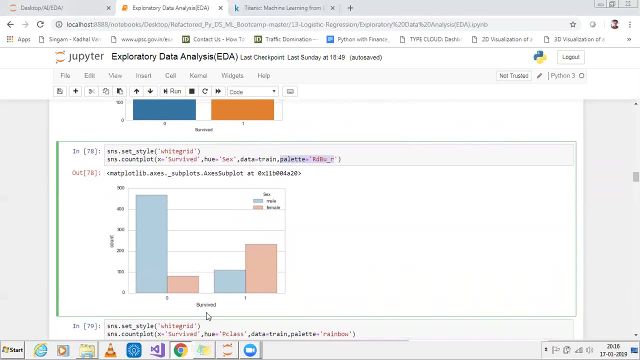 If you don't use this, it is more than enough, It is, it is finite. I basically say it is fine. Okay, Now you can see that when I use this hue parameter, which is a sex column over here Now, in this survive. 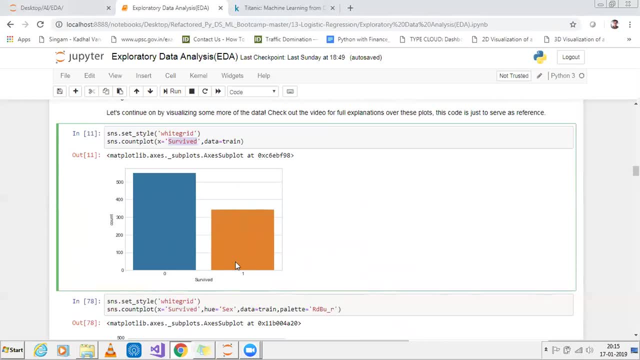 person who did not survive from that in 91 records, whereas what is the count for the person who has actually survived? now you can see that most of the people, more than 550 people, has not survived this particular titanic accident right, whereas there were some people around, more than 300. those people 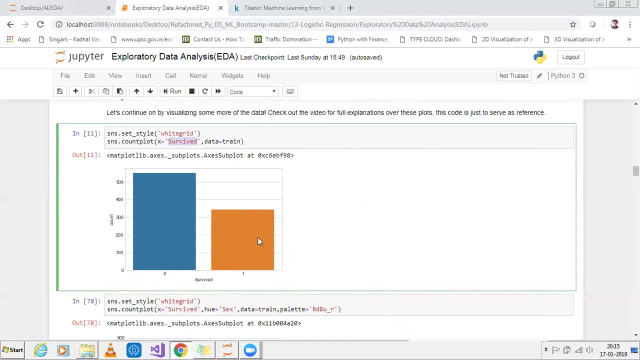 are actually survived. so this is some information i'm trying to gather from the data set, and here i'm using the c bond- very important library guys- which will actually use a lot of statistics concepts within it and it will try to show you in a visualized way. now, fine, i can see we have. 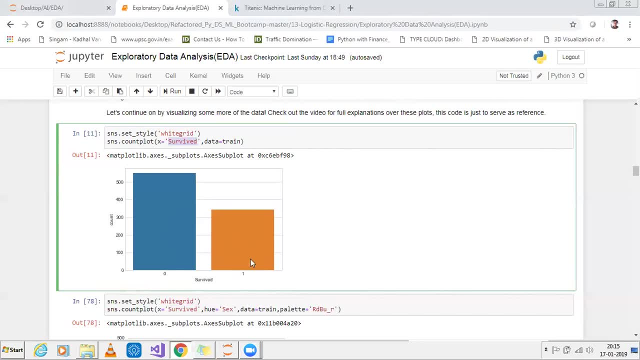 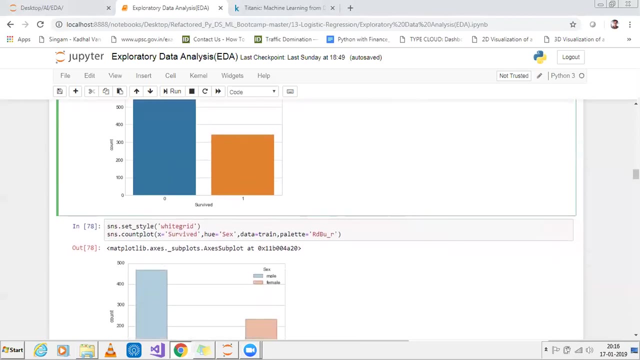 survived zero and one. many people have not survived and many people have less people have survived. now, based on the survival rate, can i just differentiate this with uh, a sex like male and female. how many people, how many males survive, how many females survive? so let us go and use the same c bond technique. now i'm going to use the counter plot. 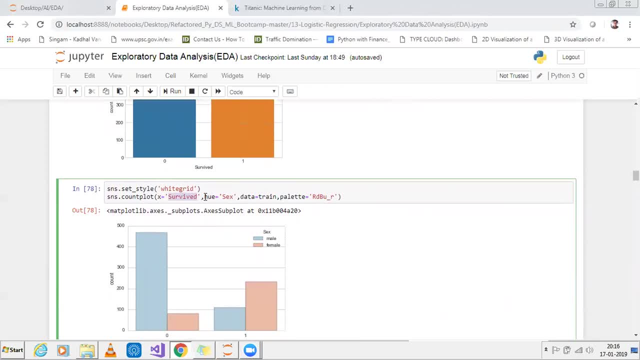 here, my x-axis is actually having the survive column, but there is one more parameter which is called as u hui. this hui will be, you know, divided based on the survive column, based on sex column. so sex- i have basically two- is uh, male and female. okay, i'm going to use the data, that is, my train data set and this palette. 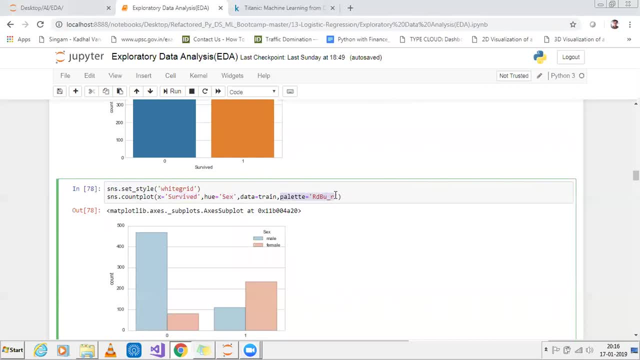 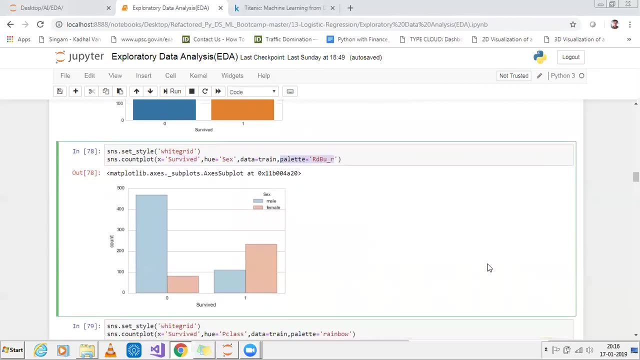 is just used to give your, uh, some some good colorful visualization, so i'm using this. if you don't use this, it is more than enough, it is, it is finite. i basically say it is fine. okay, now you can see that when i use the hui parameter, which is a sex column over here now in this survive i have. 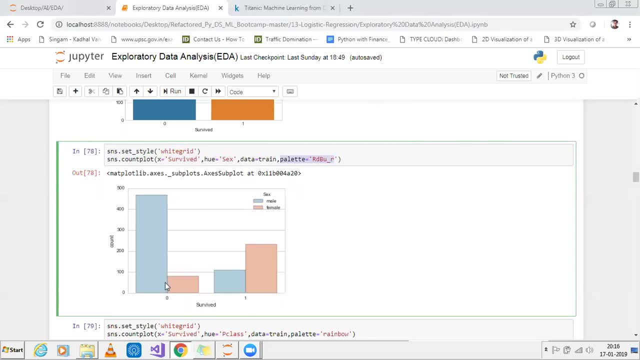 zero and one. right now, in this zero and one, i got divided into two. now what does this? you know what this blue line blue color say? it says about male sex, right, and the pink line pink color actually says about female. now, from this you know if the person has not survived. most of the people are. 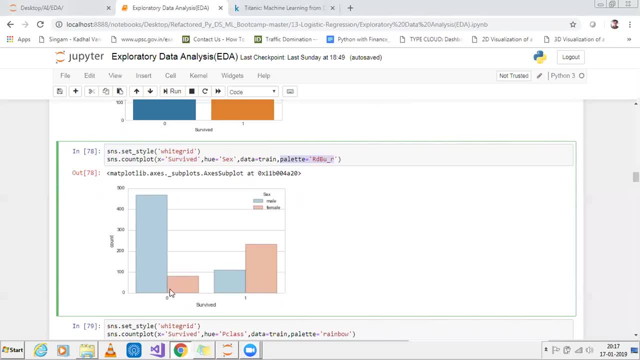 actually male. you can see that more than 450 people are male, whereas around more, around less than hundred people are females. right, so most of the male have not survived, you know, when the value was actually zero, whereas less women, you know less women died. basically, when i just say the 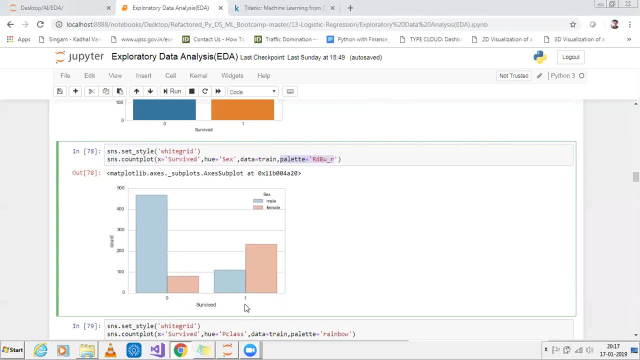 see this distribution now. similarly, in the case of survived value as one, you can see that my male is again less. it is somewhere more than 100, more than 100. uh, male only survived in this, considering- i'm considering only this 891 data set. won't get confused with them. then again, you can see this. 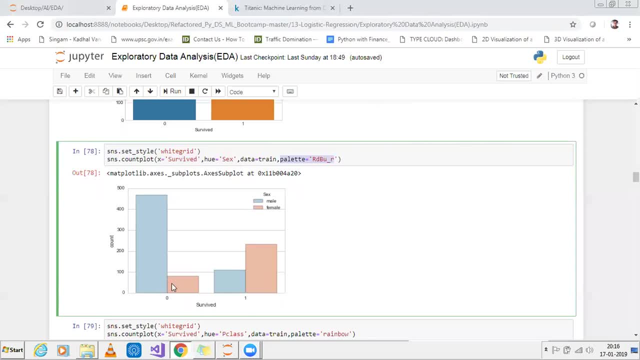 I have zero and one. Right now, in this zero and one, I got divided into two. Now what does this? you know? what does this blue line- blue color- say? It says about male sex, right, And the pink line- pink color- actually says about female. 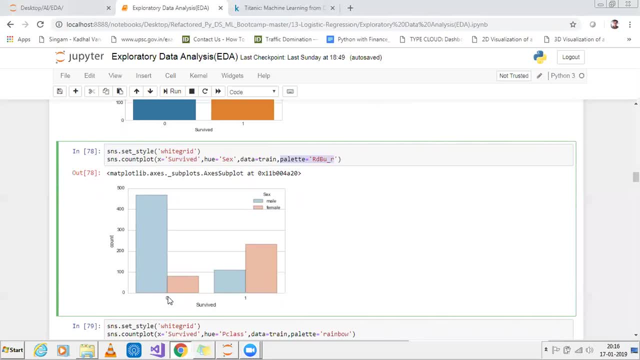 Now from this you know if the person has not survived. most of the people are actually male. You can see that more than four, 50 people are male, Whereas around more, around less than a hundred people are female right. So most of the male have not survived. 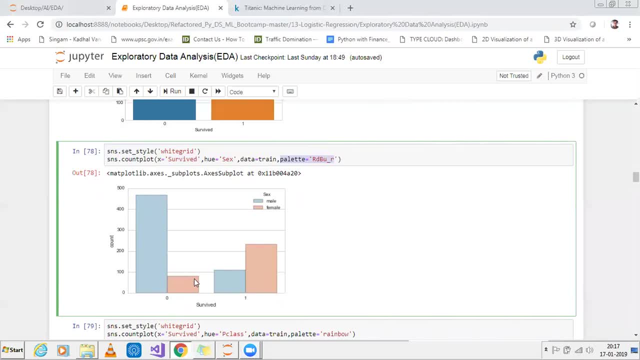 You know when the value was actually zero, whereas less women- you know less women died. basically, when I just say the zero value and when I see this distribution now, similarly in the case of survived value as one, you can see that my male is again less it is. 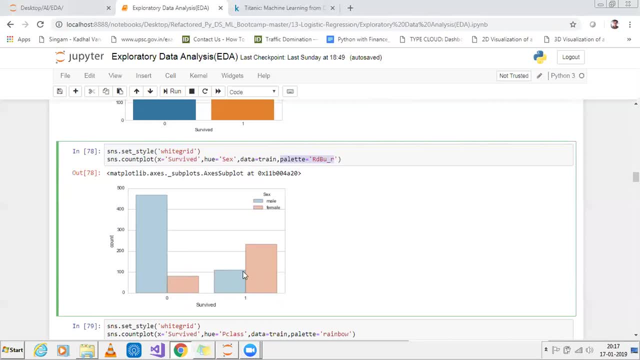 somewhere more than a hundred, more than a hundred, uh, male only survived in this, considering- I'm considering only this- 891 data set. Won't get confused with them. Then again, you can see this over here: The female value is more than 200. 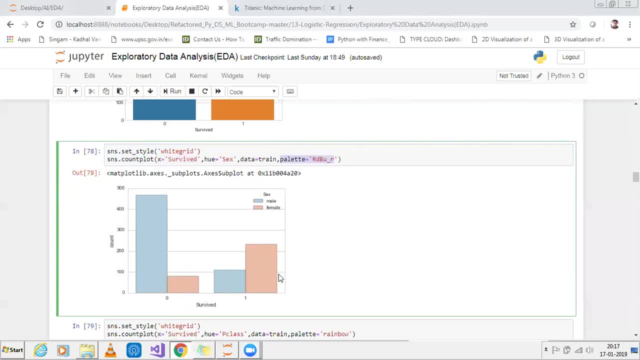 That means that more than 200 people, Uh, women- survive- Okay, Female. So this is more of the information that I'm again gathering from the data set and this is helping me to know more about the data. And what do you think that in Titanic, as we saw the movie, I hope everybody remembers- 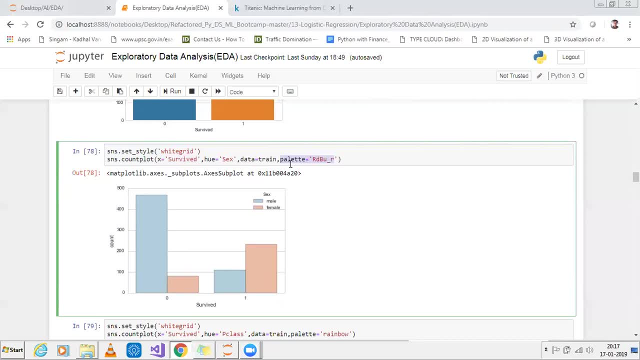 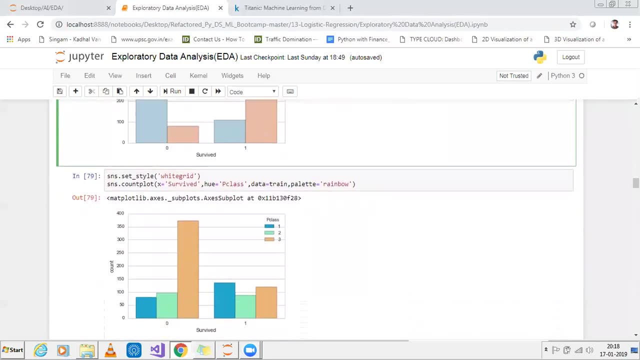 that when the accident happened, they tried to save the woman and the child, right? And then, uh, the chance was actually given to them. Now, let us go ahead and see it. Now, what I'm going to do is that based on survival? um, I'm also going to check with 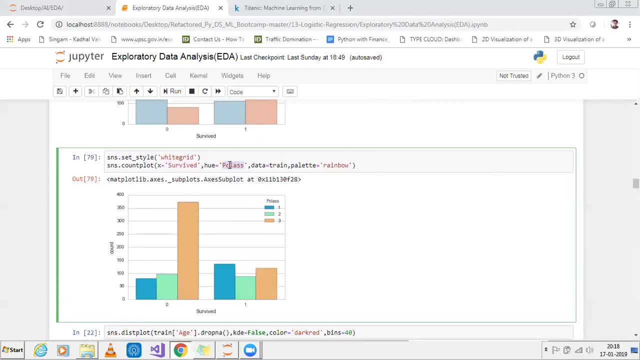 the help of passenger class. Now, usually what is happening in? uh, if you, if you have seen, I think, movie right, Rich people paid some money to the field and they were actually, you know, they were able to survive. 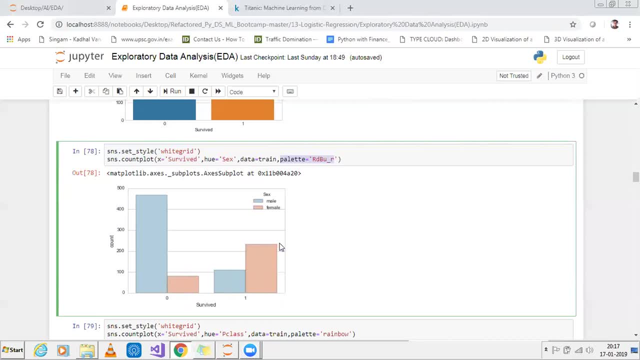 over here the female value is more than 200. that basically means that more than 200 people- uh women- survive, okay, female support. so this is more information that i'm again gathering from the data set, and this is helping me to know more about the data. and what do you think that in titanic, as 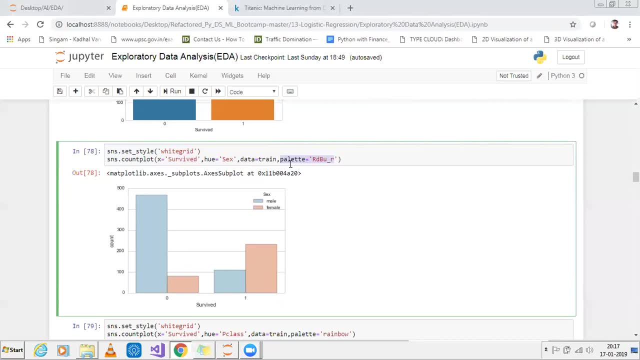 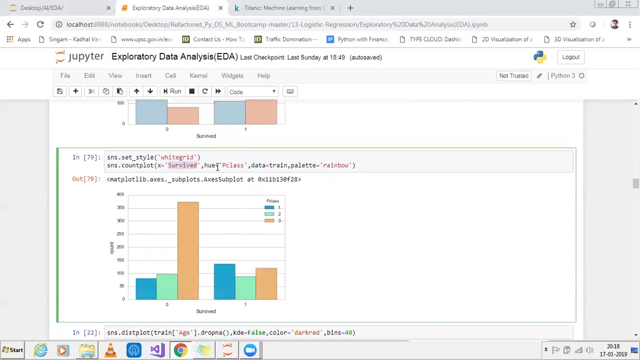 we saw the movie. i hope everybody remembers that when the accident happened, they tried to save the woman and the child right, and then, uh, the chance was actually given to them. now let us go ahead and see it now. what i'm going to do? is that based on survival? uh, i'm also going to check with the 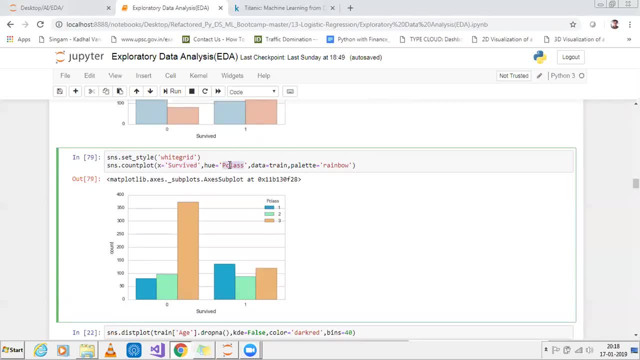 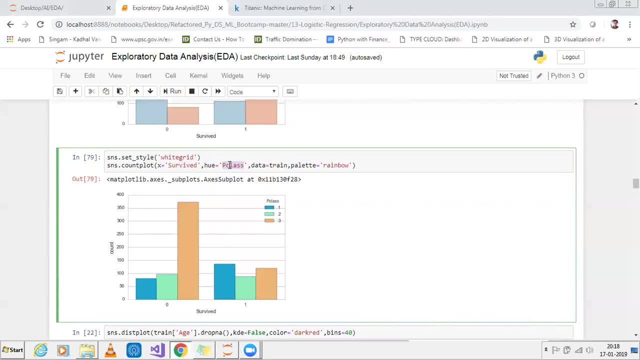 people paid some money to the sailors and they were actually. you know. they were able to survive. they were able to quickly exit the boat. right now, let us see, based on this survival and passenger class, is there any relation and is there anything that we can find out, like who has survived or not? so passenger class, again, it is an ordinal data. you. 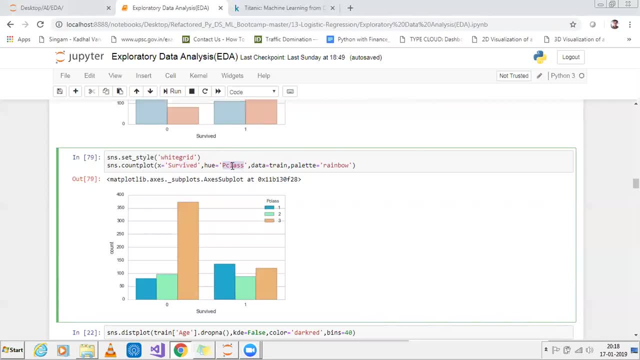 know. that basically means that if the passenger class is one, totally in this, there are three passenger classes, that is, one, two, three. okay, passenger class of one is basically a richer person, whereas Passenger class of two is actually, you know, it is just like second class. 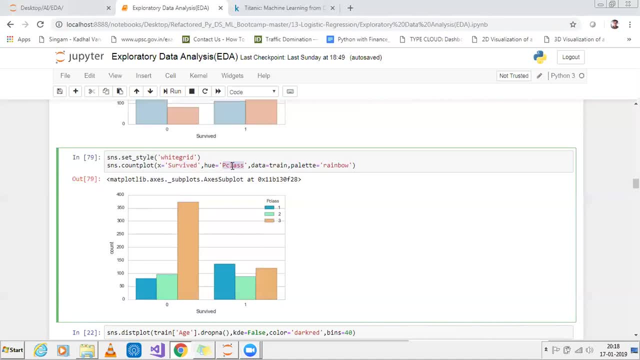 And passenger class of three is the final class. If you remember the movie Titanic, then I think the hero that is Leonardo DiCaprio actually was present in the third class passengers right. So based on that, we try to find out how many people survived. 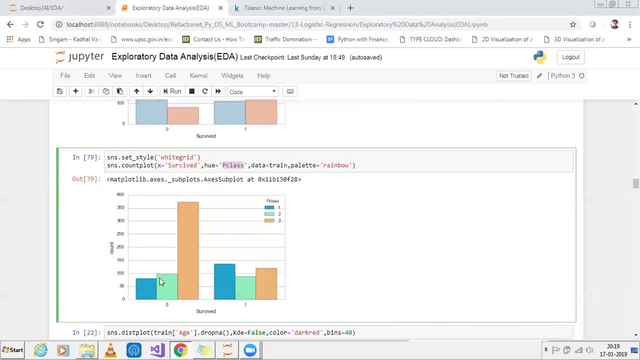 Now see this: the passenger class. over here, blue color is actually indicated for the passenger class. The passenger class two is basically indicated with this. This is just like a light green color, whereas brown color is basically for passenger three. Now the next thing is that, from this particular data visualization, 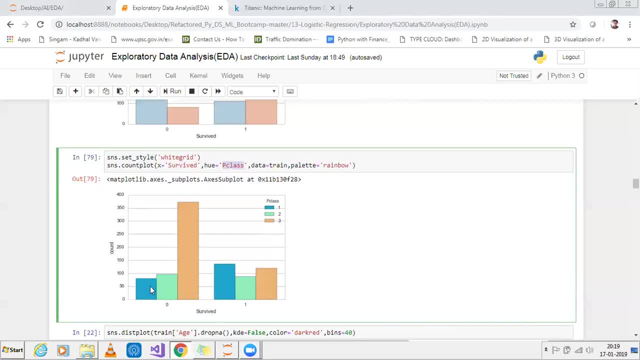 we can see that passenger class of one there were very less number of people who died, Whereas in case of passenger two, there were more people, But with passenger three, there were many people who had actually died right Now. similarly, in case of the person who had survived, you can see that from passenger class one. 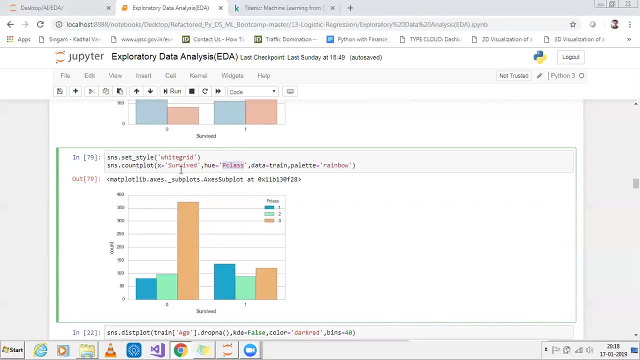 They were able to quickly exit the boat. Right now, let us see, based on the survival and passenger class, is there any relation And is there anything that we can find out, like, uh, who has survived or not? So passenger class, again, it is an ordinal data, you know. that basically means that. 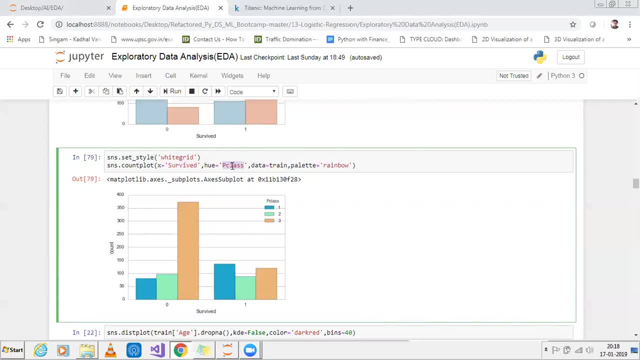 if the passenger class is one, totally in this there are three passengers, That is, one, two, three. Okay, Passenger class of one is basically a richer person, Whereas passenger class of two is actually, you know, it is just like second class, and 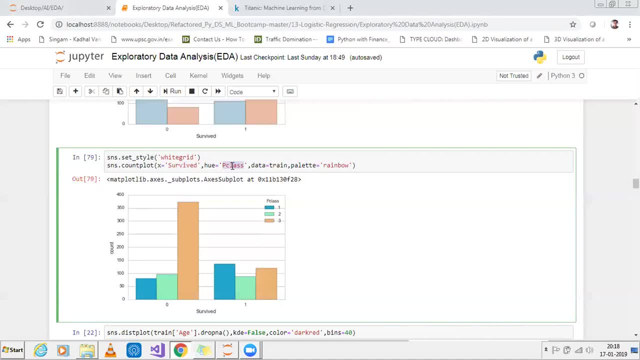 passenger class of three is the final class. Uh, if you remember the movie Titanic, then I think the hero that is Leonardo DiCaprio actually was present in the third class passengers Right. So based on that, we try to find out how many people survived. 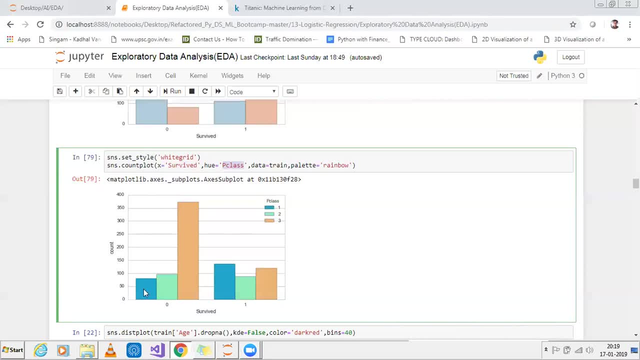 Now see this: the passenger class over here, blue color, is active. This is actually indicated for the passenger class. The passenger class two is basically indicated with this. Uh, this is just like a light green color, Whereas brown color is basically for passenger three. 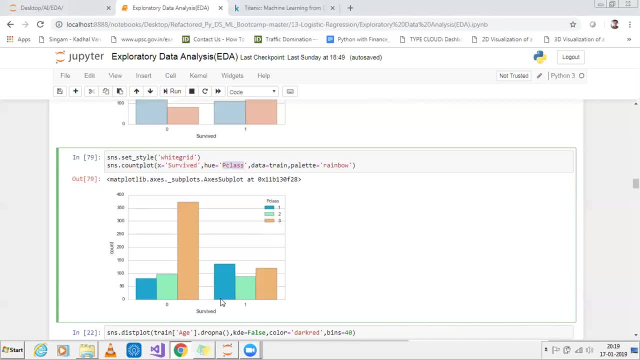 Now the next thing is that from this particular data visualization, we can see that passenger class of one there were very less number of people who died, Whereas in case of passenger two, there were more people, But with passenger three, there were many people who had actually died. 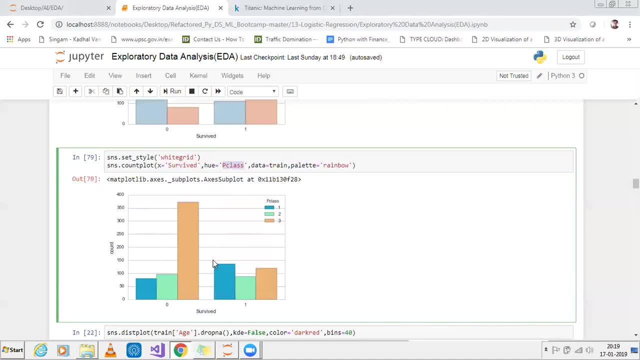 Right now. similarly, in case of the person who had survived, you can see the passenger class one. Many of them had survived, Whereas from passenger class two, they were like minimal only, Whereas passenger class three, there were very less number of people who had actually survived. 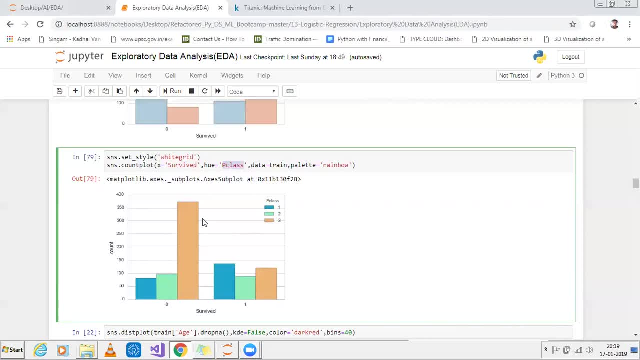 So again, we are trying to get more and more data. You're acting like a detective, right? You're trying to just see a data and you're just plotting some beautiful diagrams by using some statistic concepts, and libraries like Seabourn are getting more and more, more and more information. 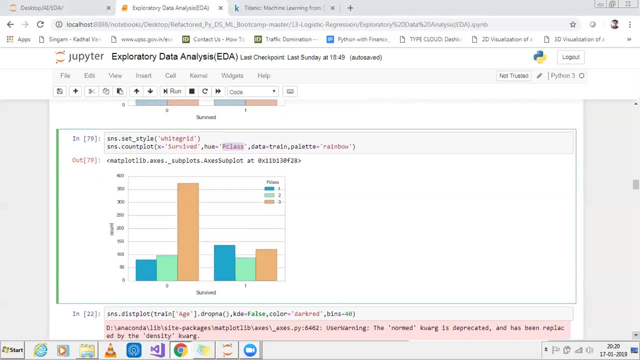 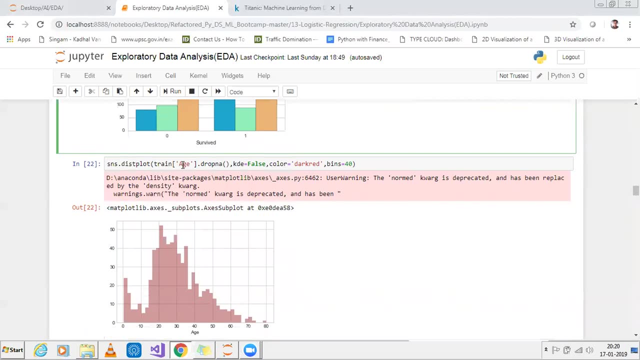 So let us just go ahead and try to explore more information from this. Now. what I'm going to do is that I'm going to see the distribution of the age. distribution of the age, whether the age follows a normal distribution or not. 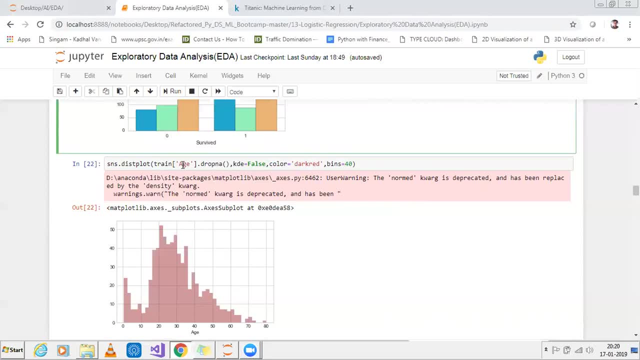 And this will actually help us to see that. what? what was the maximum number of people? I mean, what is the average age of most of the people that were in the boat? That is basically titanic. right Now I'm using a dist plot. 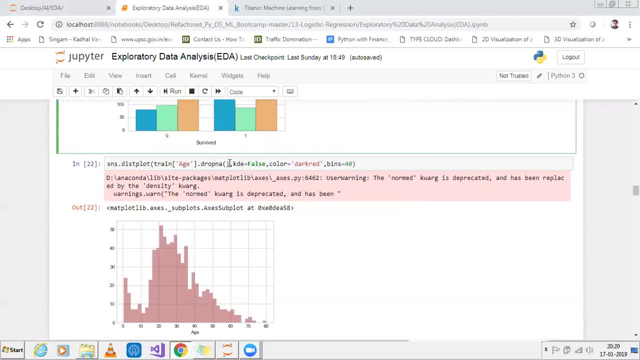 In this dist plot, I'm taking train age. First of all, I'm dropping the NA values because I saw that around 20% of values were NA in age. So first of all, I'm going to use the drop NA Here. KDE is equal to false. 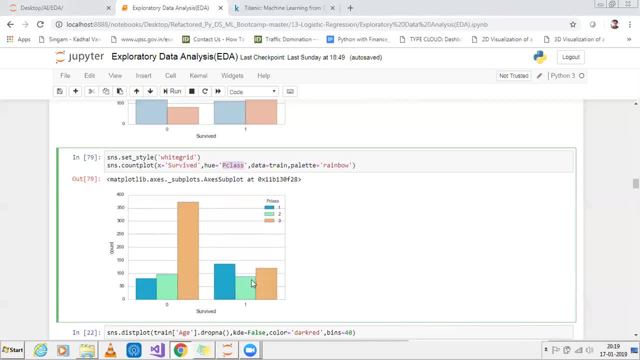 many of them had survived, Whereas from passenger class two they were like minimal only, whereas passenger class three there were very less number of people who had actually survived. So again, we are trying to get more and more data. You're acting like a detective, right. 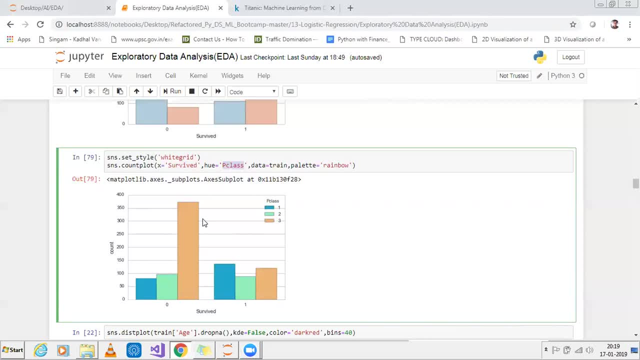 You're trying to just see a data and you're just plotting some beautiful diagrams by using some statistic concepts, And libraries like CBONI are getting more and more, more and more information, But so let us just go ahead and try to explore more information from this. 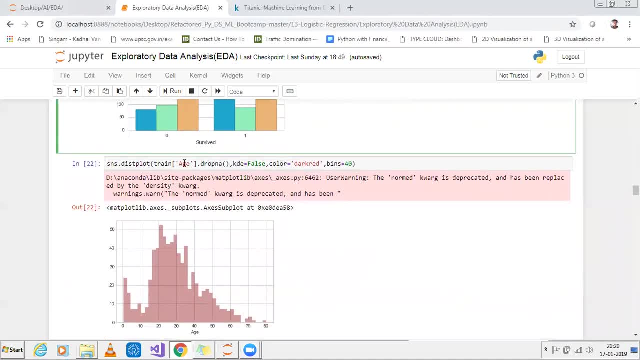 Now what I'm going to do is that I'm going to see the distribution of the age. okay, Distribution of the age, Whether the age follows a normal distribution or not. okay, And this will actually help us to see that. what was the maximum number of people of? 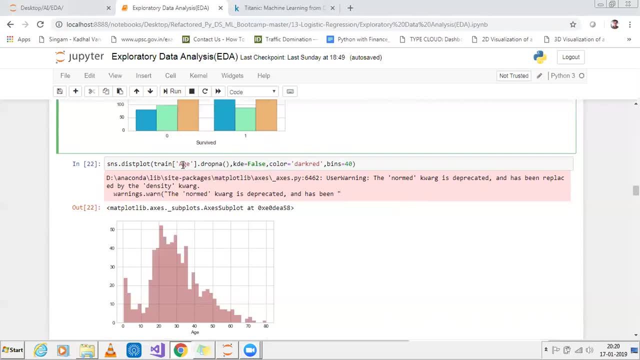 I mean, what is the average age of most of the people that were in the boat? That is basically titanic. right Now, I'm using a dist plot. In this dist plot, I'm taking train age. First of all, I'm dropping the NA values because I saw that around 20% of values were man in age. 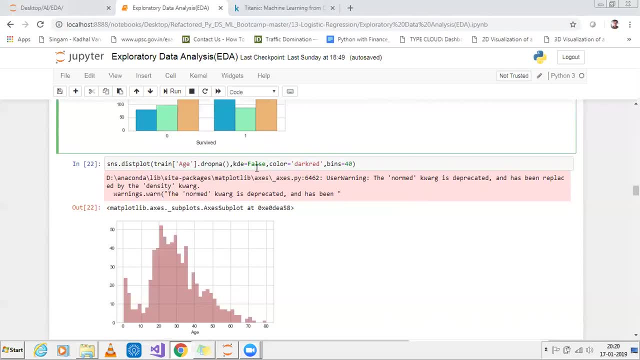 So first of all, I'm going to use the drop NA Here. KDE is equal to false. Why I'm setting is that I don't want to know the kernel density estimation. okay, Kernel density estimation is usually for creating a probability density function. 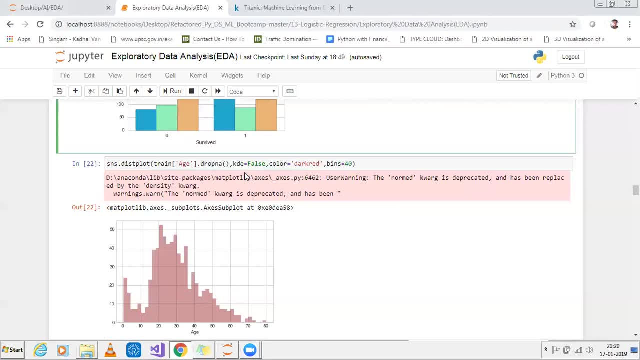 If you have, if you can go to statistics playlist of mine and you can see all these things, because I've already explained. I've explained the kernel density estimation, I've explained what is normal distribution or standard normal distribution, each and everything. Even I have explained log normal distribution. 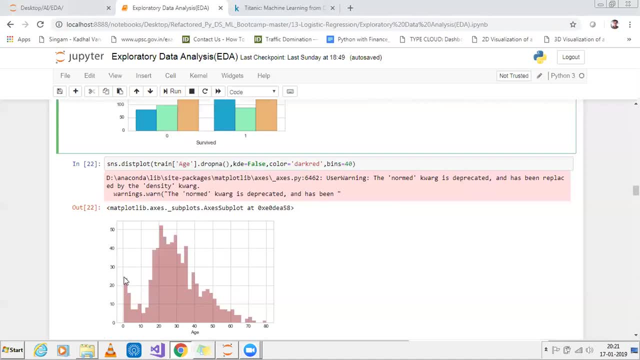 So you can go over there. So now, based on this particular distribution, you can see that this will this, this plot will actually give you a histogram and KDE is false. okay, Now, histogram basically means that what is the count of the people within this ranges of age? 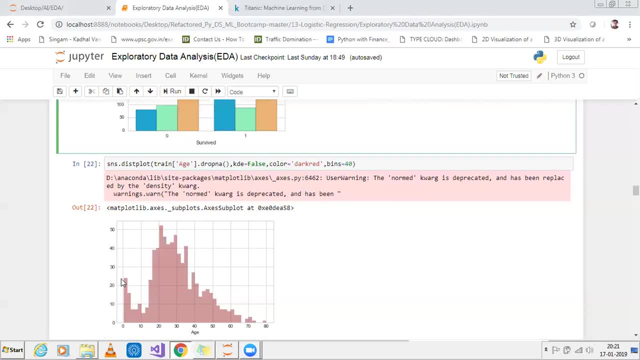 So if I just consider this zero to two, they were around more than you know 20, 20 people. So this was somewhere around 25.. If I consider the range between five to 10, they were around you know 10, 10 number of people. 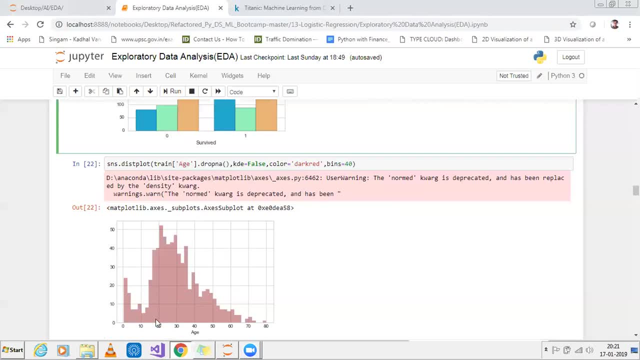 Similarly, you can see that the average age that was between 20 to 30, I think it is somewhere around, you know, 17 to 30 were maximum. You can see that maximum number of people who are in this particular age range, that is, between 17 to 30.. 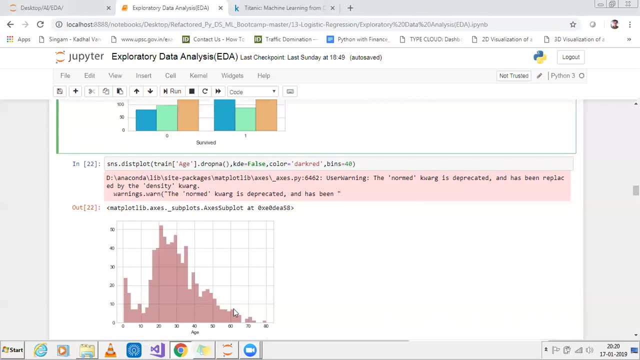 Why I'm setting is that I don't want to know the kernel density estimation. OK, kernel density estimation is usually for creating a probability density function, If you have, if you can go to statistics playlist of mine and you can see all these things because I've already explained. I've explained the kernel density estimation. 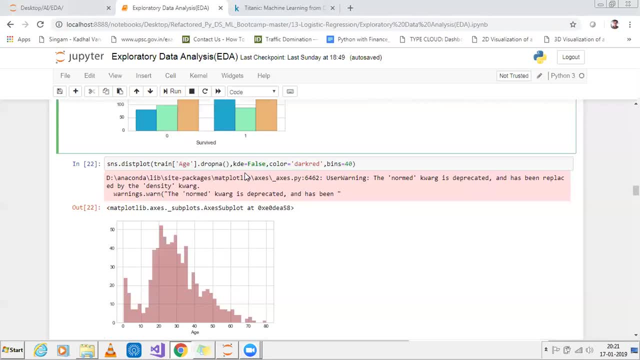 I've explained what is normal distribution, or standard normal distribution. each and everything, even log normal distribution. You can go over that. So now, based on this particular distribution, you can see that this will. this dist plot will actually give you a histogram and KDE is false. 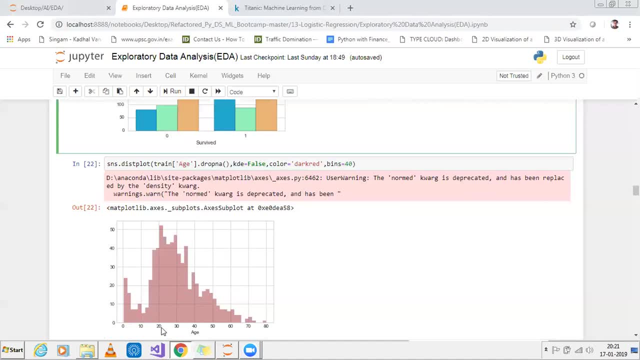 OK now. histogram basically means that what is the count of the people within these ranges of age? So if I just consider this, 0 to 2, they were around more than you know. 20,, 20 people. So this was somewhere around 25.. 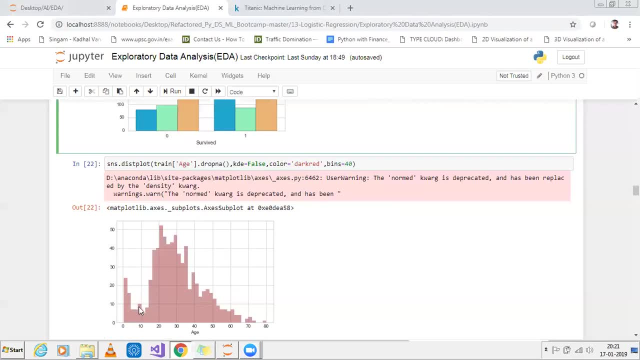 If I consider the range between 5 to 10, they were around you know 10, 10 number of people. Similarly, you can see that the average age that was between 20 to 30, I think it is somewhere around, you know 17 to 30- were maximum. 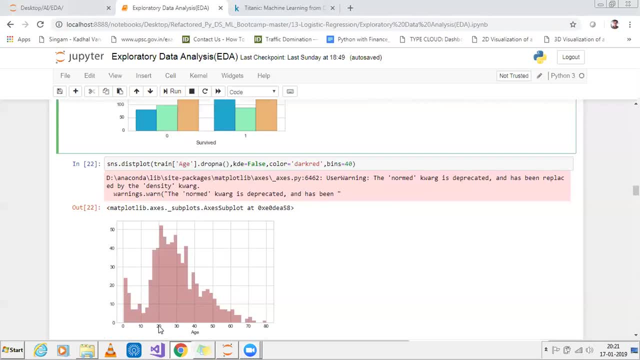 You can see that maximum number of people were in this particular age range, That is, between 17 to 30. And then still they were very less number of people who were at age like 70, 80, 60.. Yeah, So all this information is this. 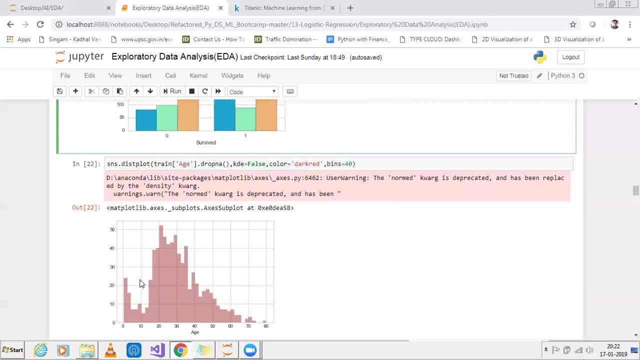 This plot actually helps you to get a histogram- OK, and you can remember it. helps you to find out the frequency of, basically the count of the people in this particular range of age. OK, because I've taken this age as my exact now. 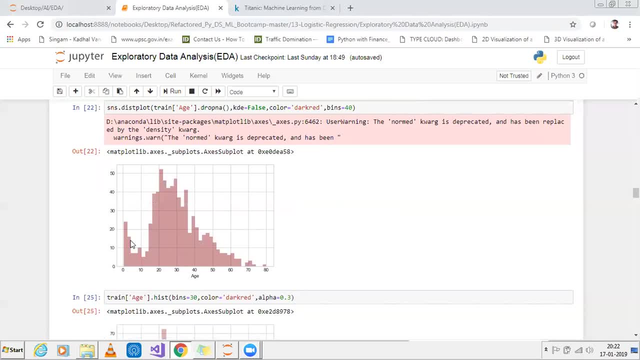 Now here you can basically see that this is also kind of normal distribution. It forms a bell curve, So this is just like a bell curve with some outliers. That is fine. Now you can also see that here I've used bins at 40.. 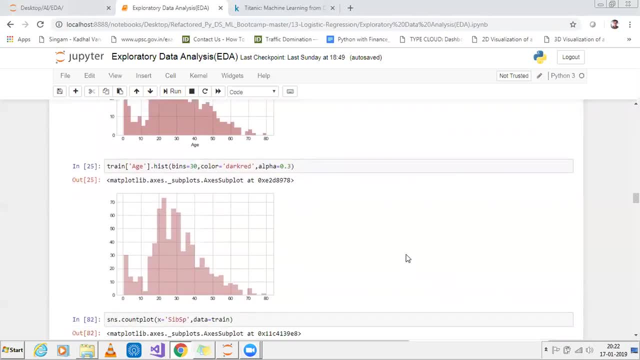 I can also reduce my bins to 30 and I can use matplotlib function like this: dot hist. OK, so in the data frame I have a dot hist function which will help you to see the distribution. So either way, You can. either you go by this plot or you can go by hist. 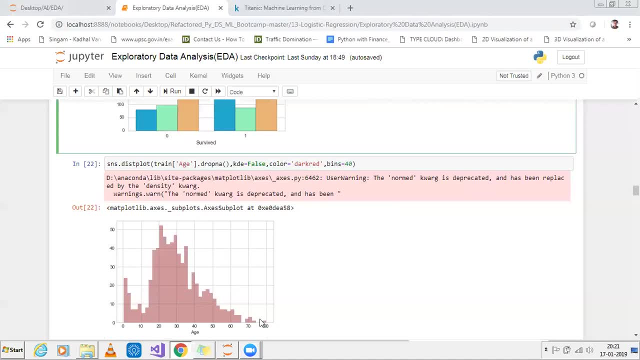 And then still they were very less number of people who are, uh, elder age, like 70,, 80,, 60. Yeah, So all this information is basically this: this plot actually helps you to get a histogram, Okay. 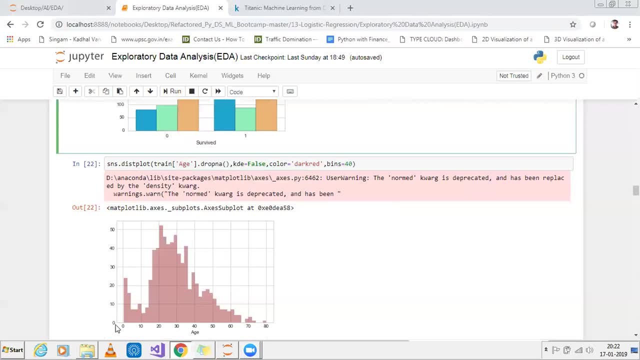 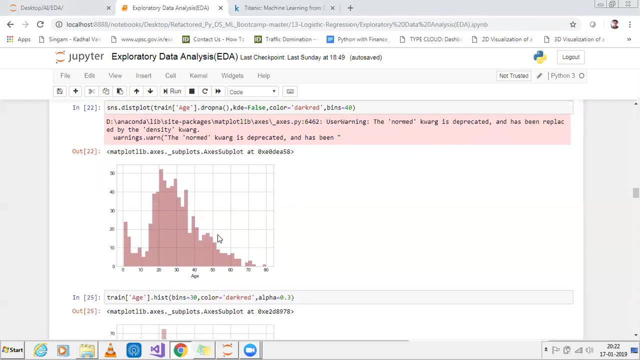 And histogram, remember, it helps you to find out the frequency of the uh, basically the count of the people in this particular ranges of age. Okay, So, because I've taken this age as my exact now, Now here you can basically see that this is also kind of normal distribution. you know, it forms a bell curve, but this is just like a bell curve with some outliers, but that is fine. 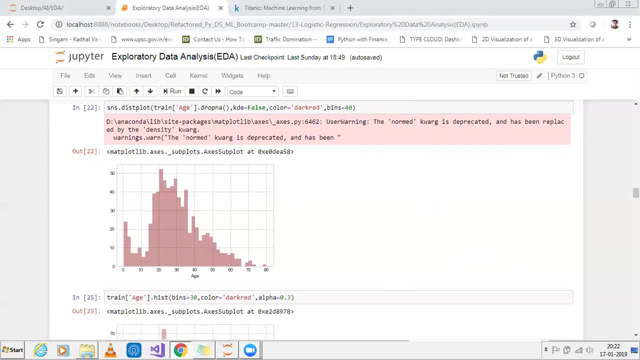 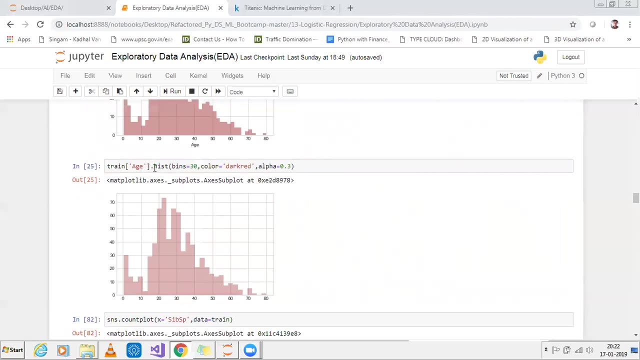 Now you can also see that here I've used bins at 40.. I can also reduce my bins to 30 and I can use matplotlib function like hist, dot hist. Okay, So in the data frame I have a dot- hist function which will help you to see the distribution. 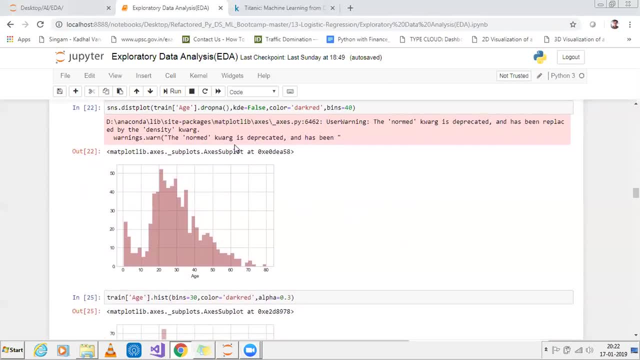 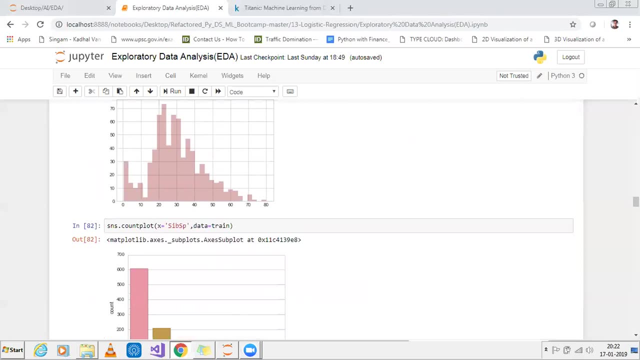 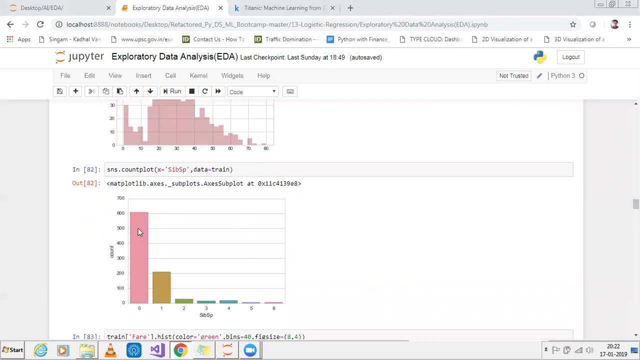 So either either way you can do, you can either use go by distplot or you can go by hist, So these two are in-built. now the next thing is that that I'm trying to find out is that I'm trying to find out the count plot of sibling plus spouse, you know. so here again, this will give me the frequency or the count of the people who either did not have any sibling or spouse who had one sibling, or spouse who had two siblings, or spouse who had three siblings or spouse. 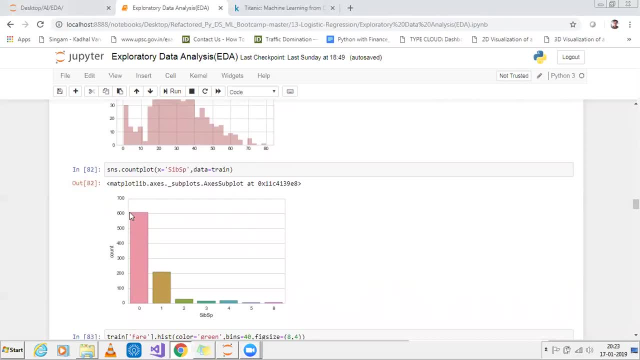 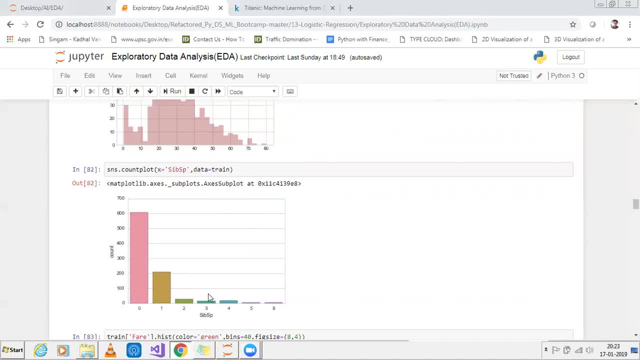 In this she is traveling with her spouse. In this two case it may be sibling and spouse, and three, it may be two siblings, one spouse, something like that. Okay, So this is the information. Again, this is: we are trying to get more and more information. 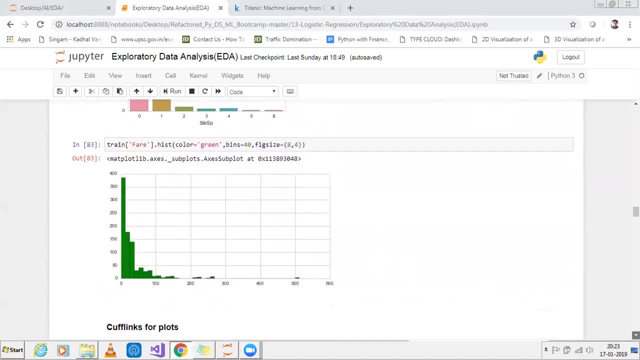 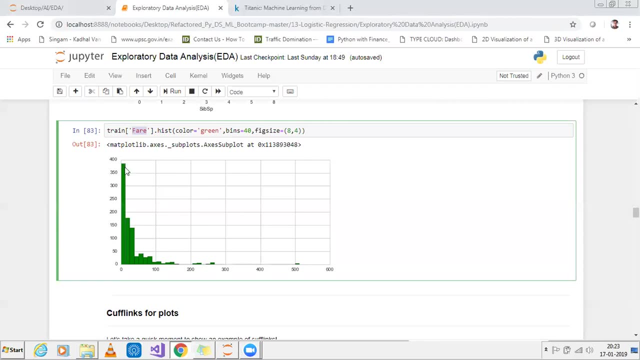 Similarly, what I'll do is that I'll try to get more and more information. I'll try to find out the train fair histogram also. If you just use dot test, you can see that what is the average fare of the people who have bought that tickets. 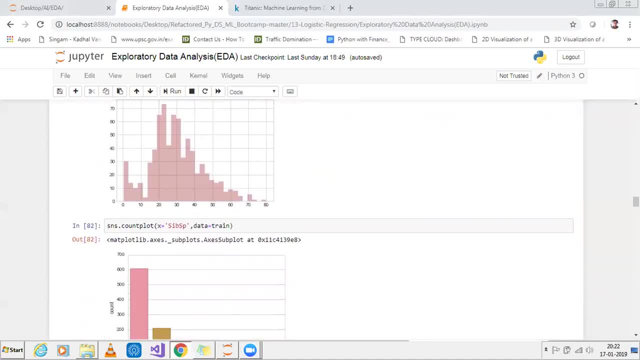 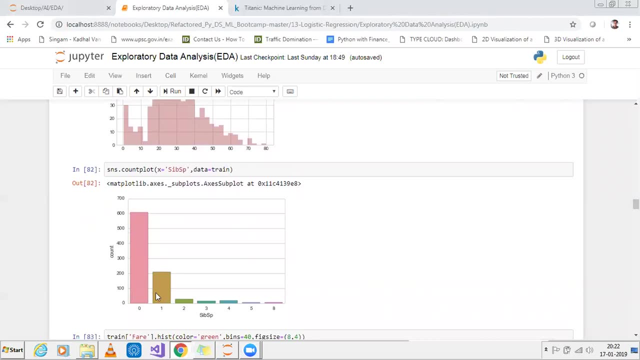 So these two are in between. Now, the next thing is that that I'm trying to find out is that I'm trying to find out the count plot of sibling plus spouse, you know. So here again, this will give me the frequency or the count. 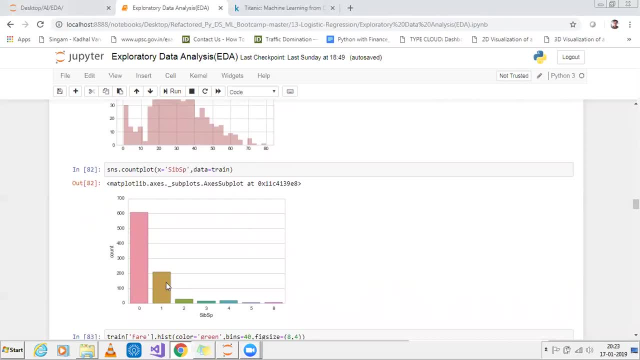 of the people who either did not had any sibling, or spouse who had one sibling, or spouse who had two siblings, or spouse who had three siblings or spouse, And you can see that maximum people did not have any sibling and they were around 600 people, whereas who had this one is basically with respect to spouse, because 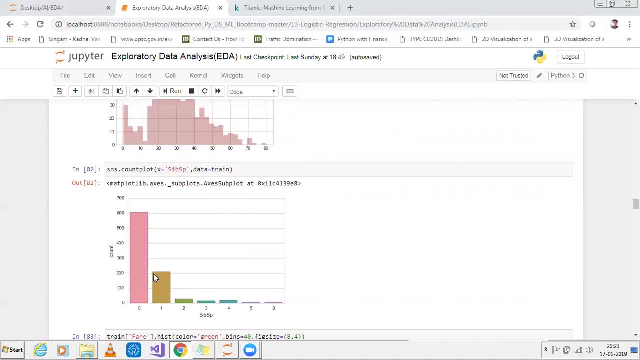 no one will travel without spouse, like with only children. So this one basically says that the person was traveling with the spouse. In these two cases it may be sibling and spouse, and three, maybe two siblings, one spouse, something like that. 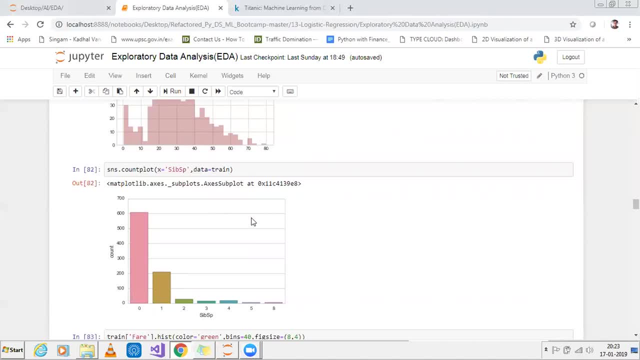 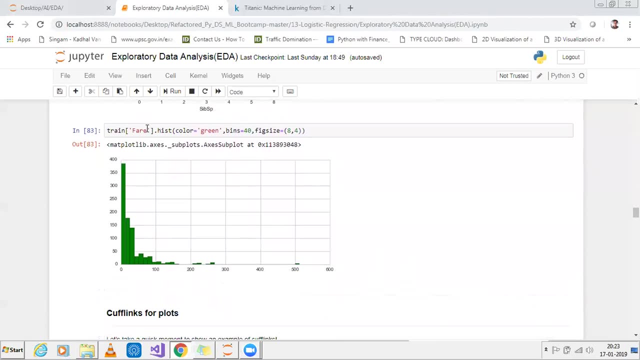 OK, so this is the information again. This is: we are trying to get more and more information. Similarly, what I do is that I'll try to find out the train or fair histogram. If you just use dot hist, you can see that. what is the average? 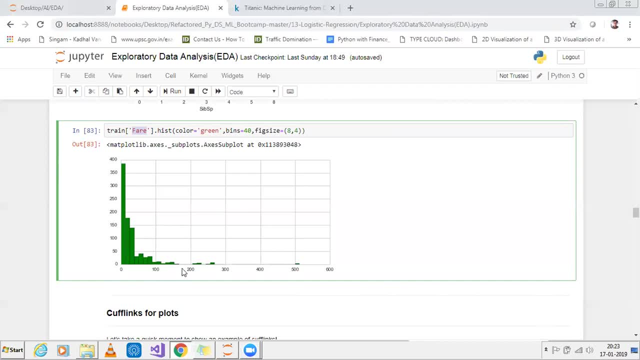 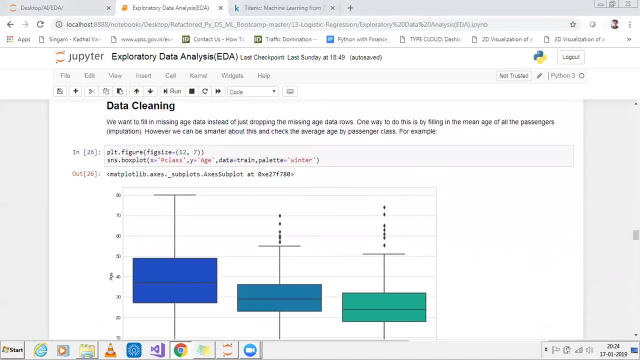 pair of the people who have bought the tickets, and how did they buy? OK, now, when I go down the first step, as I told you that I'm going to remove the null values, Now see what? how do I remove the null values? 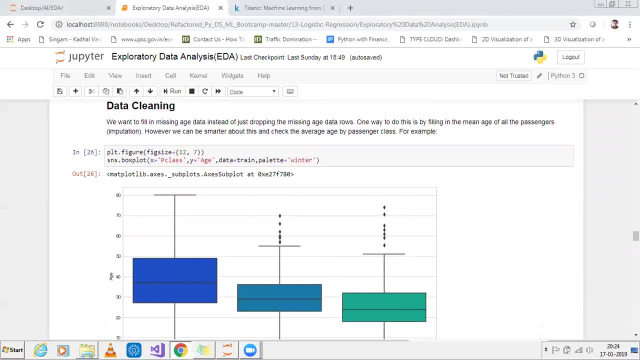 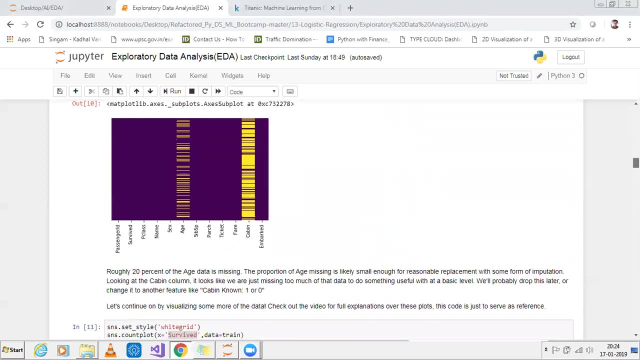 Null values of first of all. First of all I'll go with the age column and then you saw that I'll be going to my next column. over here We can see that we thought columns basically had null values. One is age and one is cabin. 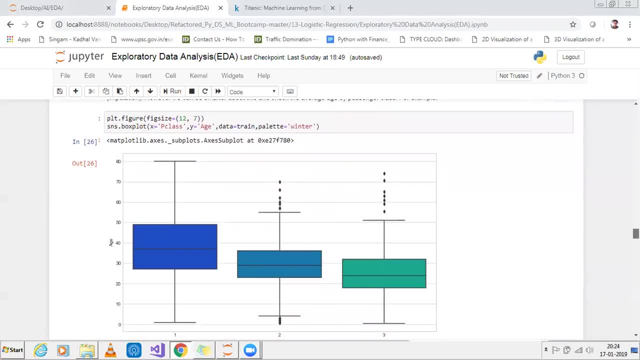 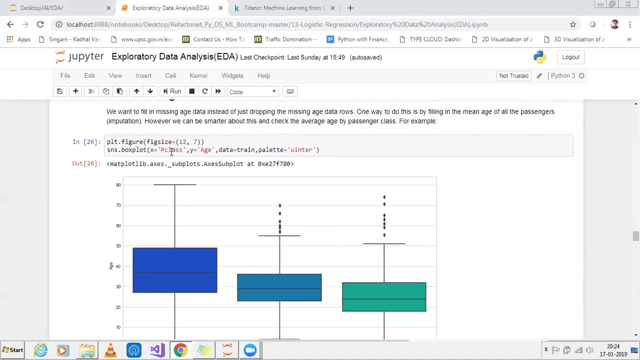 So now age and cabin. First of all, we'll try to remove the age column. But before removing the age column, OK, I did some analysis and I found out that there was some relation with respect to the passenger class and age. OK, with respect to the passenger class, 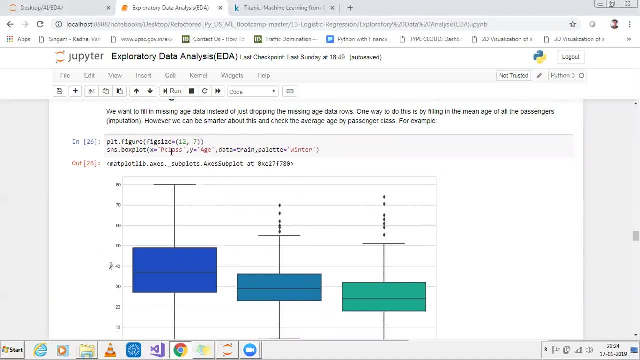 I try to find out what is the average age of the people, Whereas supposedly the passenger class is one, And what is the average age of this? So for that we will be using something called a box plot. OK, in the box plot in the X axis, I'll give passengers. 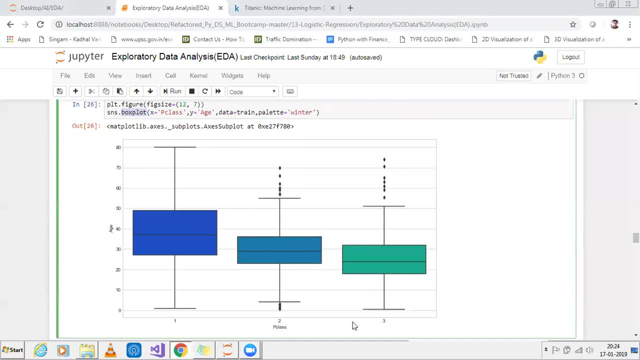 Now you can see that in the passenger class I have three values: One, two, three- because in my data set I have three passengers And in my Y axis I basically have age. OK, now, based on this information, I'm trying to find out. 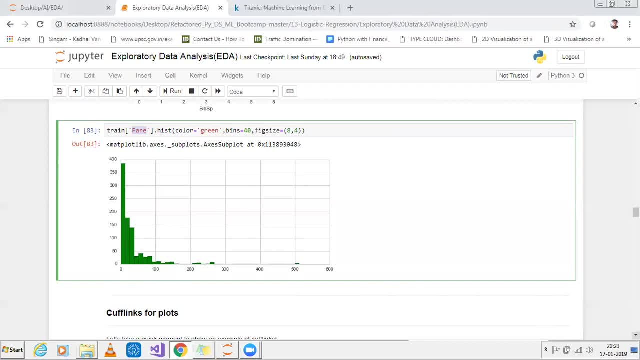 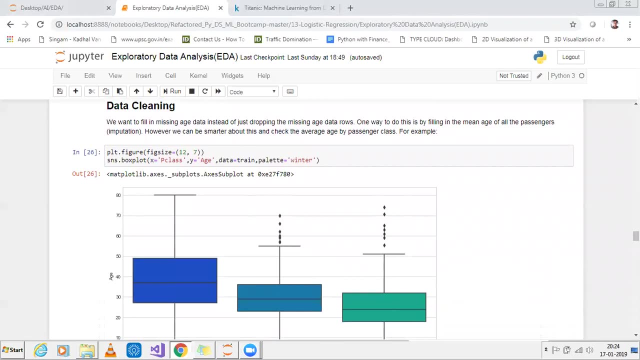 and how did they buy? okay, Now, when I go down guys, first step, as I told you that I'm going to remove the null values, Now see how do I remove the null values. Null values of. first of all, I'll go with the H column. 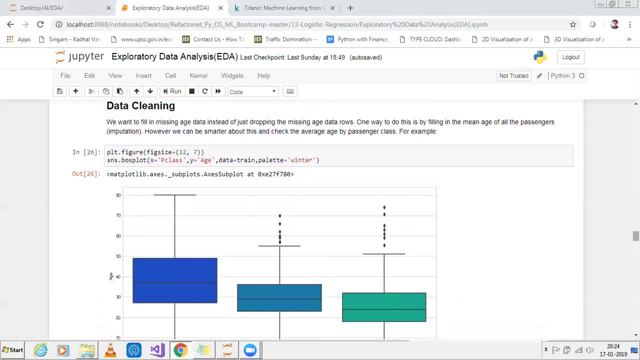 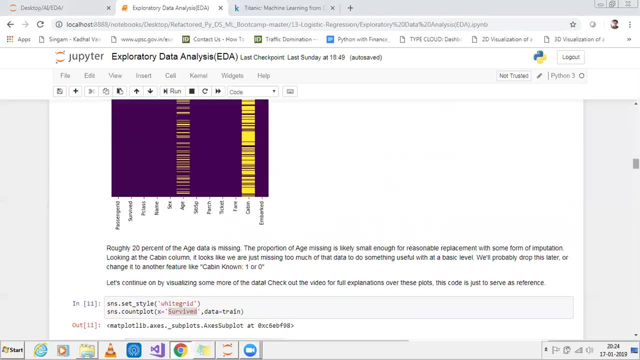 and then you saw that I'll be going to my next column over here, So you can see that which are columns basically had null values. one is H and one is cabin. So now H and cabin. first of all, we'll try to remove the H column. 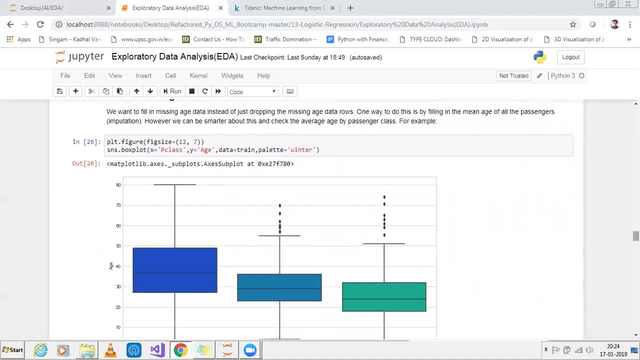 But before removing the H column, okay, I did some analysis and I found out that there was some relation with respect to the passenger class and H, okay, With respect to the passenger class, I tried to find out what is the average age of the people. 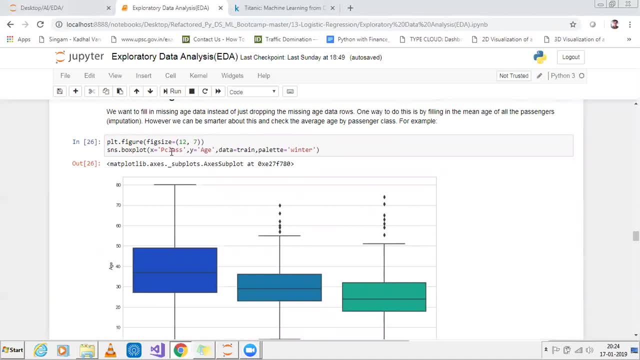 Whereas, suppose, if the passenger class is one, and what is the average age of this? So for that we'll be using something called a box plot. okay, In the blocks plot in the X axis I'll give passenger class. Now you can see that in my passenger class. 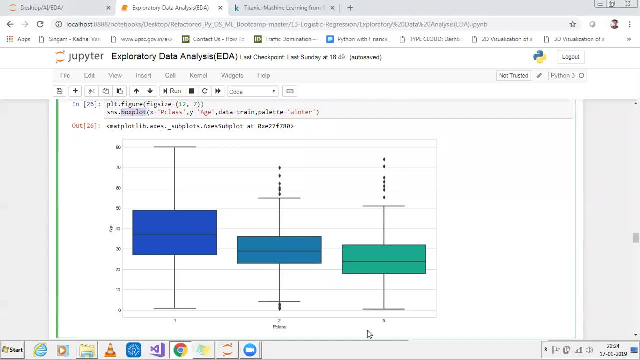 I have three values: one, two, three- because in my data set I have three passengers And in my Y axis I basically have H. okay, Now, based on these two information, I'm trying to find out. this is basically a box plot. 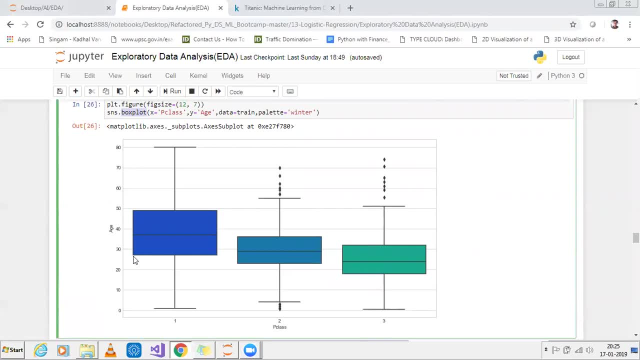 And this box plot gives us a lot of information. This line actually gives me 25 percentile value. This gives me the average 50th percentile value, Whereas this gives me the 75th percentile value. So if I see this box plot, 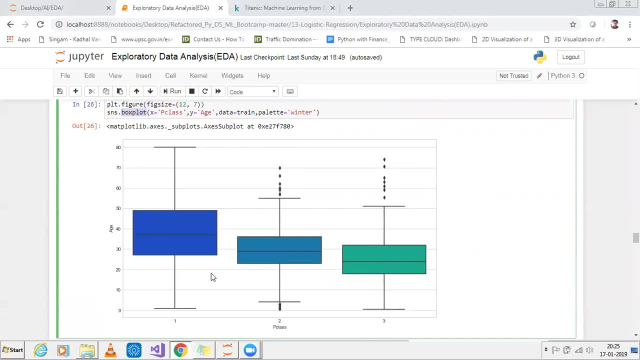 the average value is somewhere over here for passenger class as one And for box plot. for the second passenger class, my box plot and H has the average value over here, And similarly for passenger class three, my average value is three. okay. 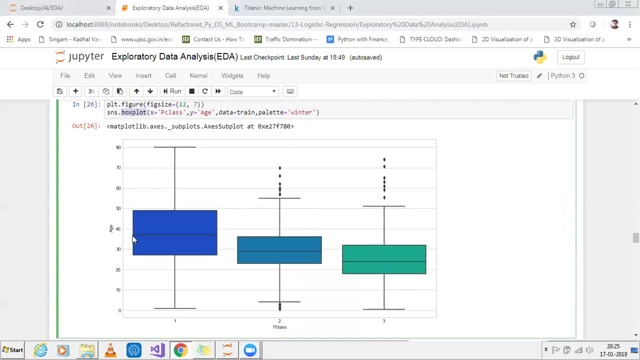 So this I'm considering somewhere around 37 or 38. This may be somewhere around 29. And this may be somewhere around 24, 25.. So let us see, based on this passenger class and H, I'm going to replace the nan value in the H column. 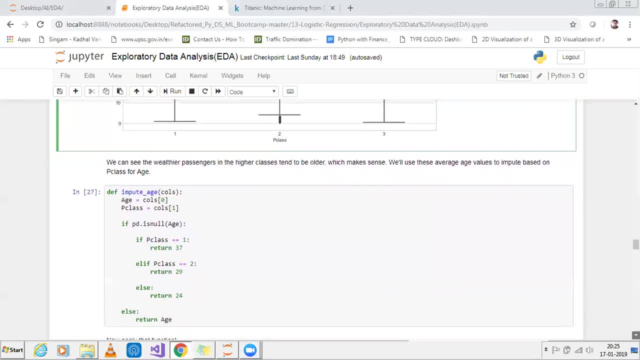 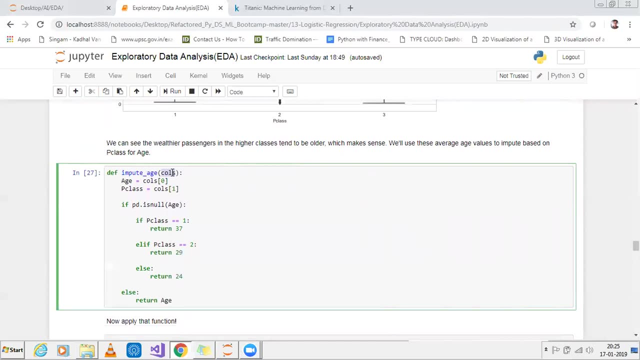 So I'll put a simple condition saying that I'll create a function where I'll be giving the columns- that is my H column, okay, Age and passenger column. sorry, Sorry, age and passenger class column. So first column will be my H. 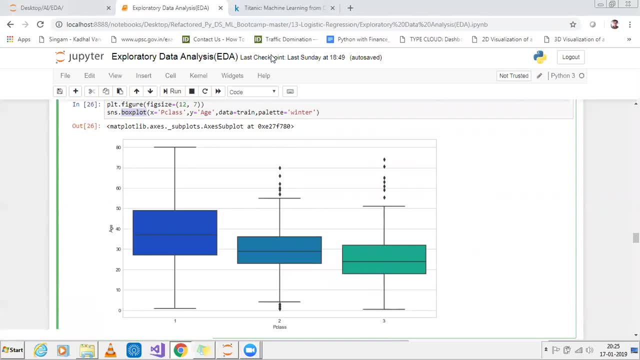 This is basically a box plot, And this box plot gives us a lot of information. This line actually gives me twenty five percentile value. This gives me the average percentile value, whereas this gives me the seventy five percentile value. So if I see this box plot, the average value somewhere over here for passenger class is one. 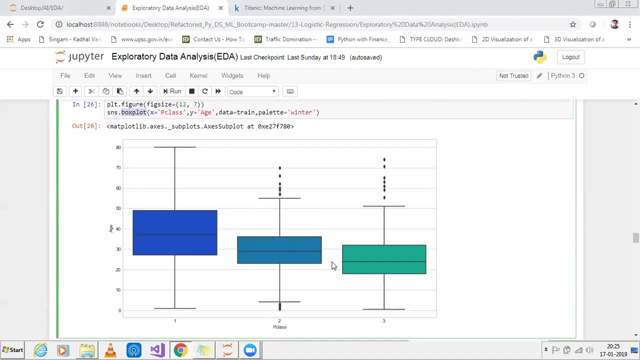 And for box plot. for the second passenger class, my box plot and age has the average value over here, and similarly for passenger class three, my average value OK. so this I'm considering somewhere around, you know, thirty seven or thirty eight. 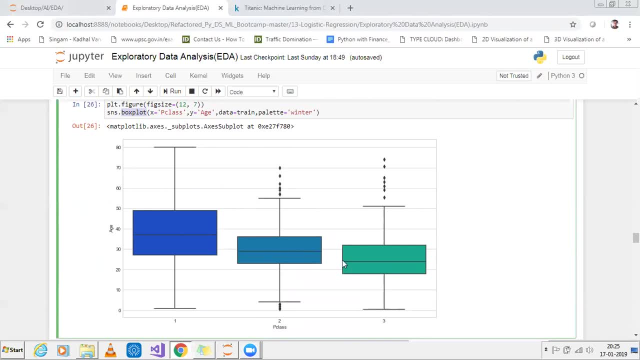 This may be somewhere around twenty nine. This may be somewhere around twenty four. So let us see. based on this passenger class and age, I'm going to replace the value in the age column. So I'll put a simple condition saying that I'll create a function. 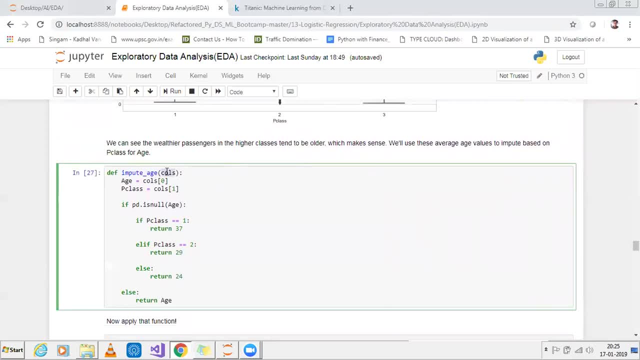 where I'll be giving the columns. that is my age column. OK, Age and passenger column. sorry, sorry. age and passenger class column. So first column will be my age, The second column will be my passenger. I'm putting a condition. 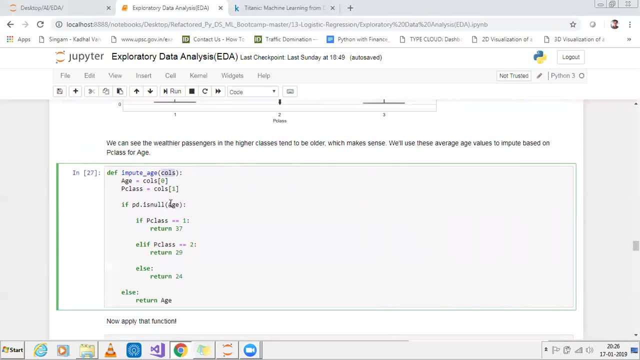 If PD is null age, OK. if this is true. if there is a null value in that age column, OK. at that time. if that passenger class which I'm getting from here is one, OK, I'm going to replace it with thirty seven. 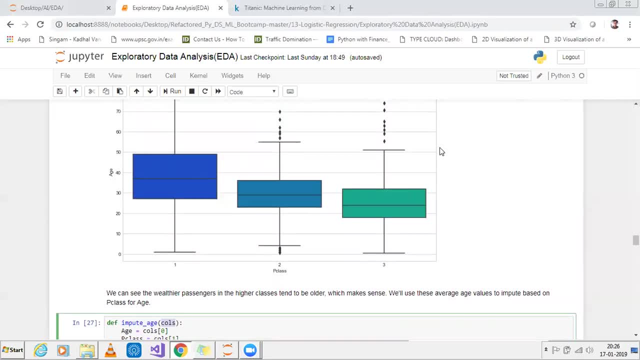 Why I'm replacing with thirty seven? Because over here you can see that my average value of the passenger of first class with age is thirty seven. OK, similarly with the passenger class of two is somewhere around twenty nine. So, similarly, I'm going to replace it. 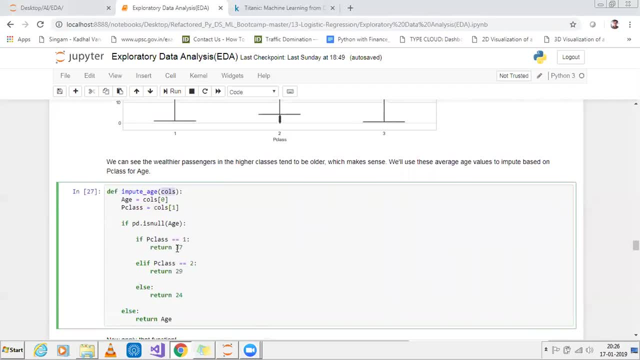 I'm saying: oh yeah, if my class is equal to one, I'm returning thirty seven. If my class is equal to two, I'm returning twenty nine, and I'm returning twenty four. OK, otherwise I'm just returning the age back. 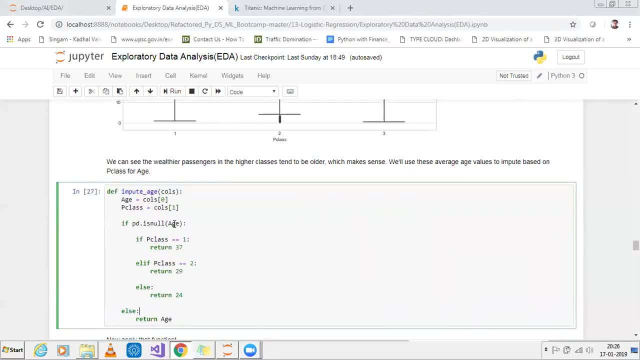 That's it When I'm returning the age back when the age is not OK. so After implementing this, you know, the first class with eight sub values will get replaced with thirty seven, twenty nine, twenty four. So here I'm replacing all these values. 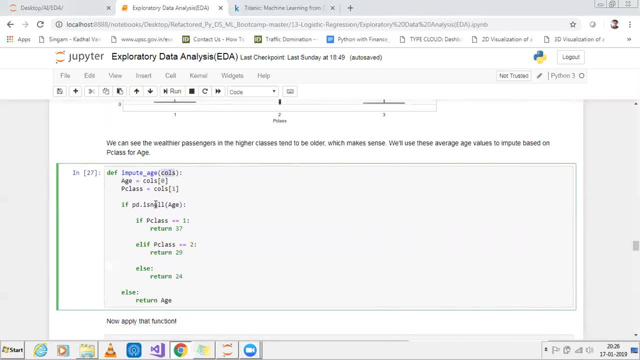 The second column will be my passenger column. I'm putting a condition: if PD dot is null H, okay. If this is true, if there is a null value in that, if there is a null value in that H column, okay. 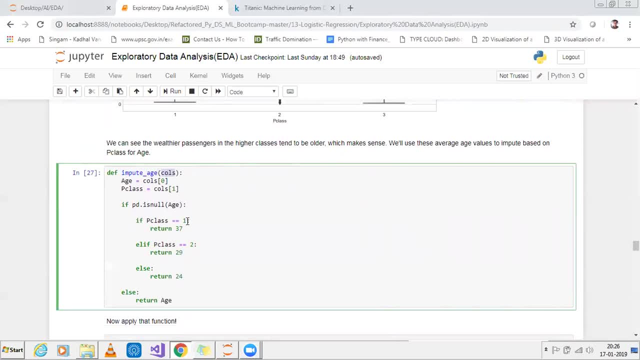 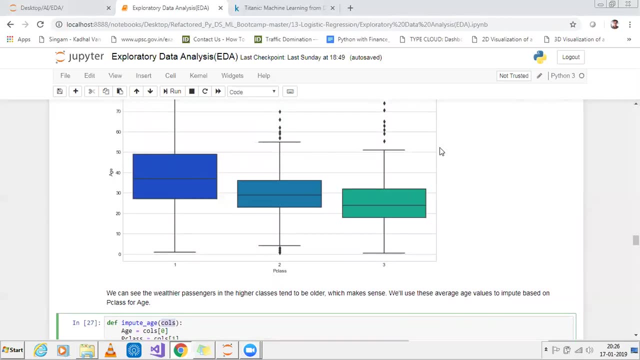 At that time. if that passenger class which I'm getting from here is one, okay, I'm going to replace it with 37.. Why I'm replacing with 37? Because over here you can see that my average value of the passenger of first class with age is 37, okay. 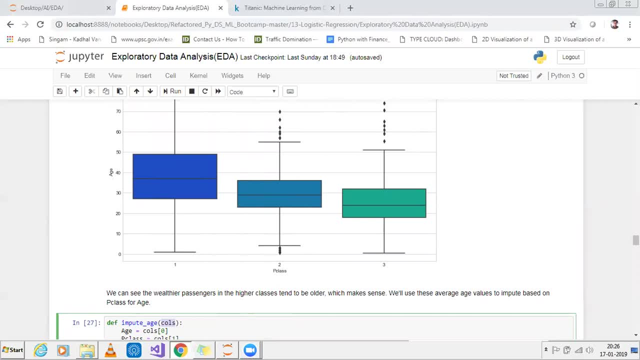 Similarly with the passenger, class of two is somewhere around, you know, 29.. So similarly I'm going to replace it. I'm saying over here, if my T class is equal to one, I'm returning 37. That is a. 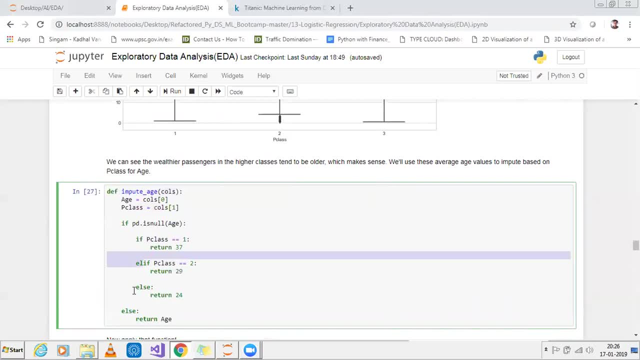 If my T class is equal to two, I'm returning 29.. Else, I'm returning 24, okay, Otherwise, I'm just returning the H back. that's it When I'm returning the H back when the age is not null, okay. 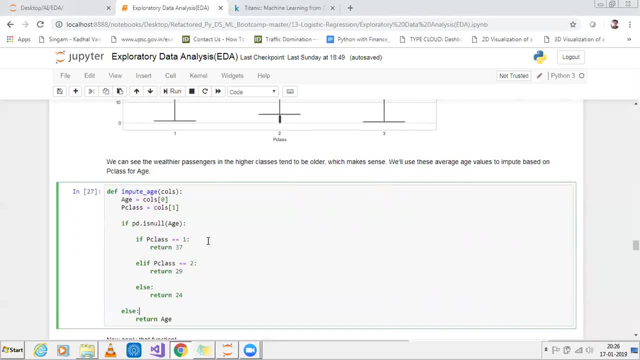 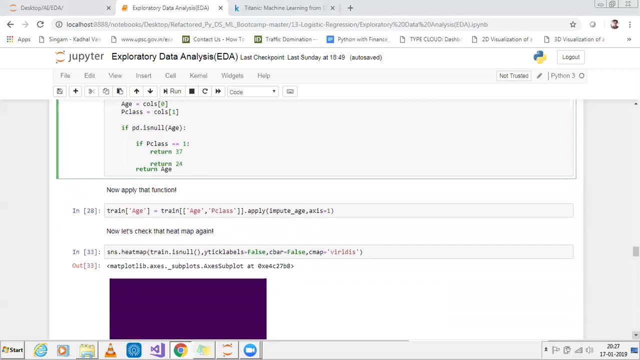 So after implementing this, you know, the first class with H sub values will get replaced with 37,, 29, and 24.. So here I'm replacing all these values. Now what I have to do is that I have to take train, okay. 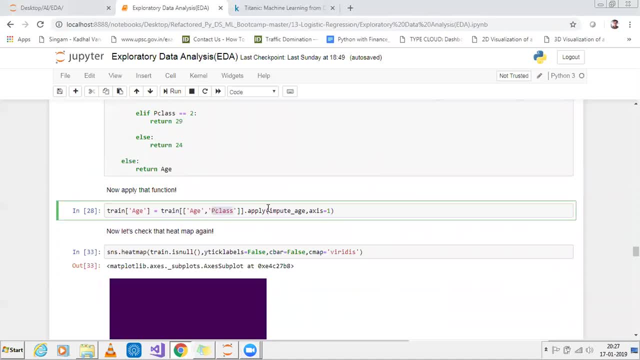 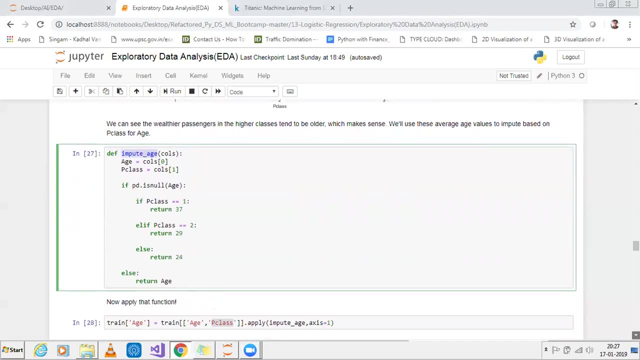 Train And I'm considering the age and P class. okay, Train, And I'm considering the age and P class and I will call this function that is impute age. okay, Impute age by using the function called as apply. 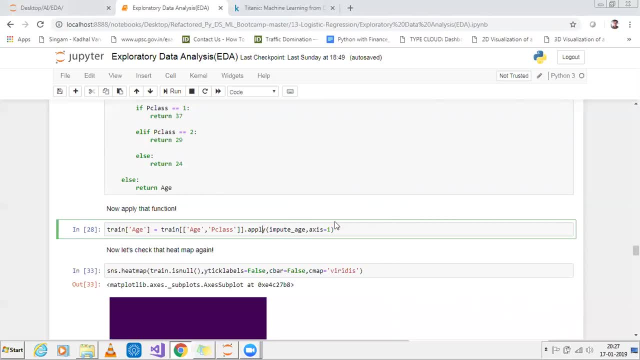 Now apply when I give the function name as impute underscore age and I'm going to set the axis for the one at that time- what this impute age is going to do for each and every record set of presenting age. 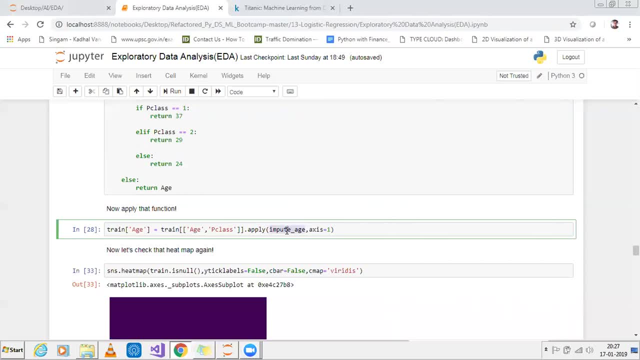 and passenger class is going to apply this particular impute underscore age function. Now, once we do this, and once again we when we check, and once again we when we check, and once again we when we check. 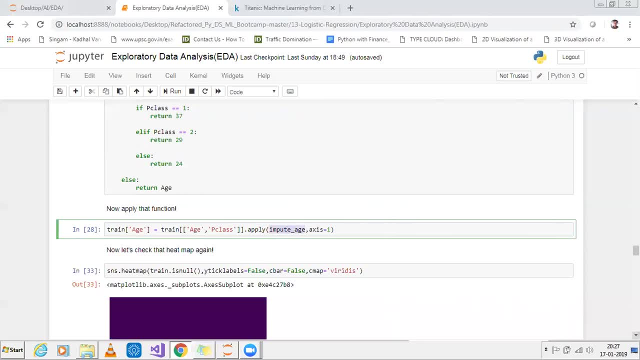 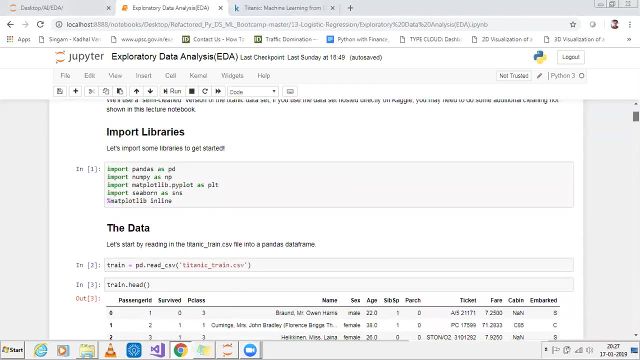 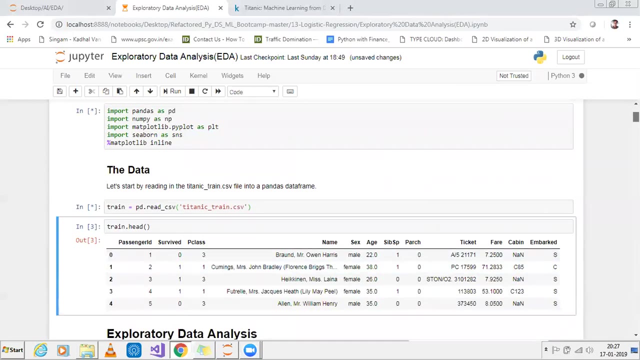 the same heat map that we checked initially. now you can see that my. okay, just a second. I'll just execute this. Just a second. okay, this is I have got executed. this is my data set. okay, So just give me a second. I'm just going to execute it. 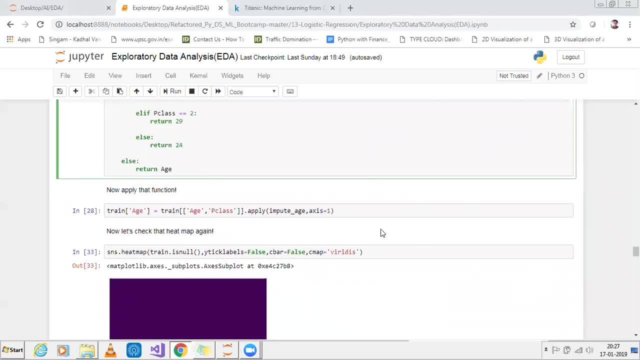 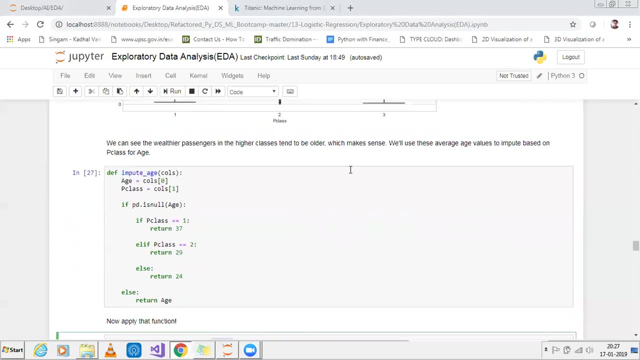 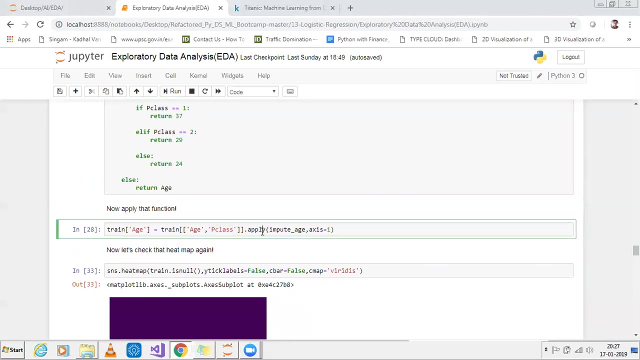 Now what I have to do is that I have to take train, train, and I'm considering the age and class And I will call this function that is imputed, imputed by using the function College dot apply, dot apply When I give the function name as impute. 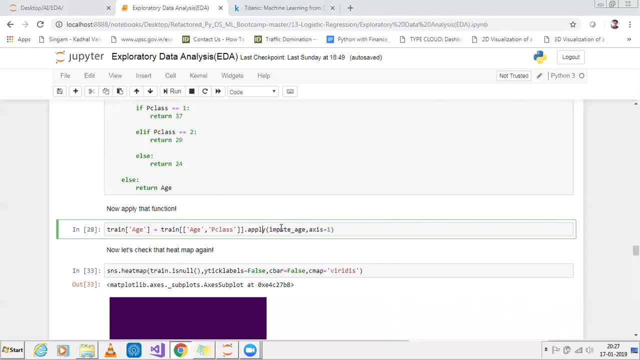 underscore age and I'm going to send taxes for the one at that time. what this impute age is going to do for each and every record that are present, in age and passenger class is going to apply this particular impute And this way. 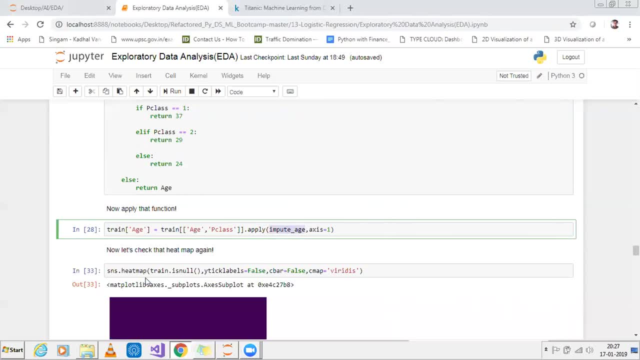 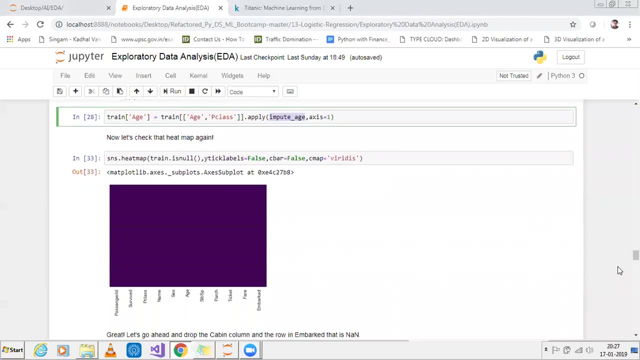 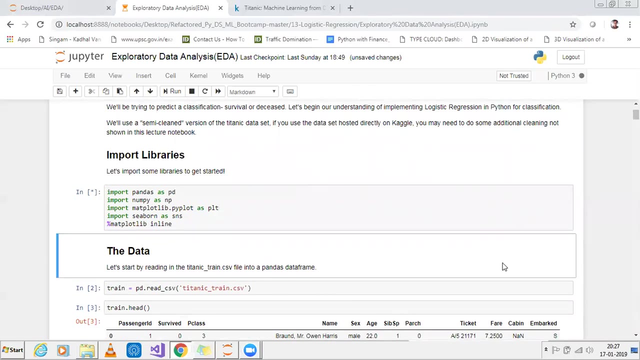 Now, once we do this, and once again we when we check the same heat map that we checked initially. Now you can see that my just a second. I'll just execute this, Just a second. This is I have got executed. This is my data set. 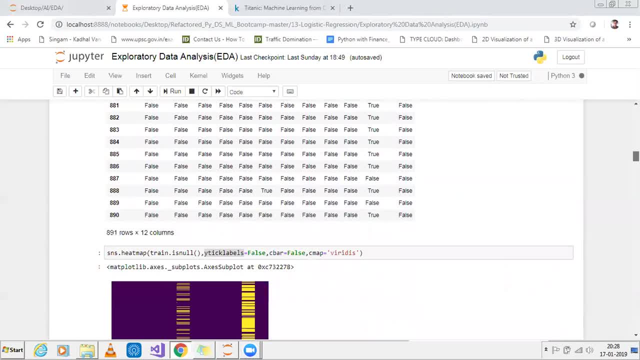 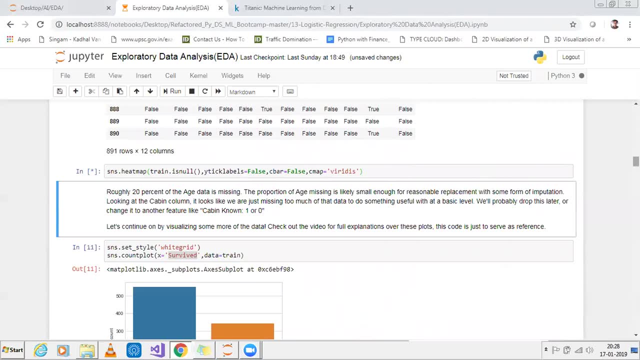 OK, so Just give me a second. I'm just going to look at it, because there I can actually see my heat map. because after replacing the H column, right at that time you'll be seeing that that each column will never be more. 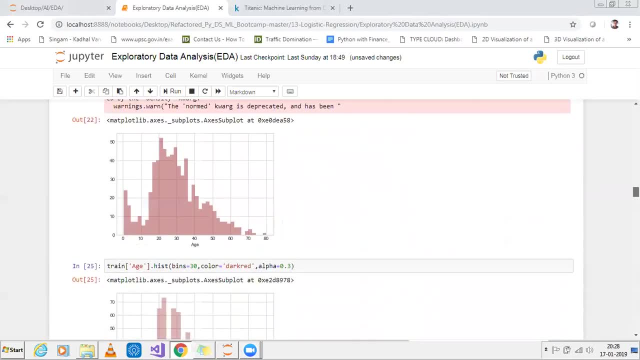 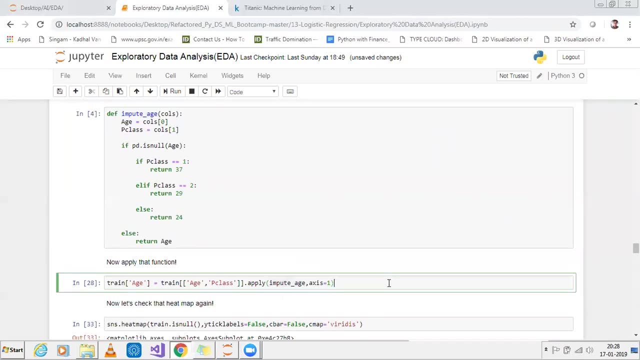 Now you can see that I'm having both this right. What I'm going to do is that I'll go down over here. you know, I'll go down here and create this function. I'll execute this. OK, my heat map is ready. 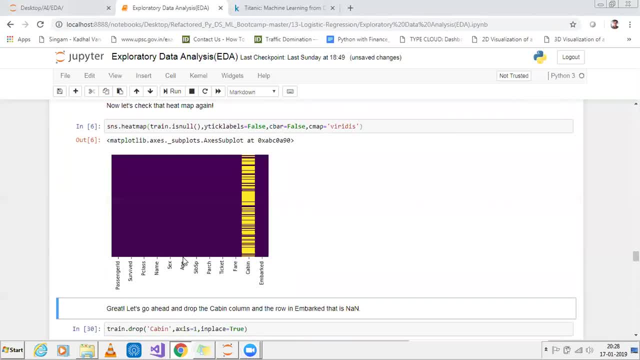 Now, if I go and check my heat map, you can see that my H column has got replaced with the with the values, that is, with respect to the passenger, So I don't get any yellow lines over here. Now I have to replace this cabin. 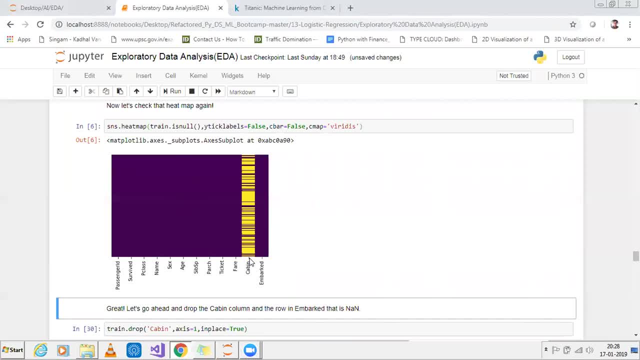 But the problem with this cabin is that there are many, many, many null values. Right, Sorry, there are many, many null values. Now, if I want to replace something instead of this null values, you know I have to apply some feature engineering, and feature engineering is altogether. 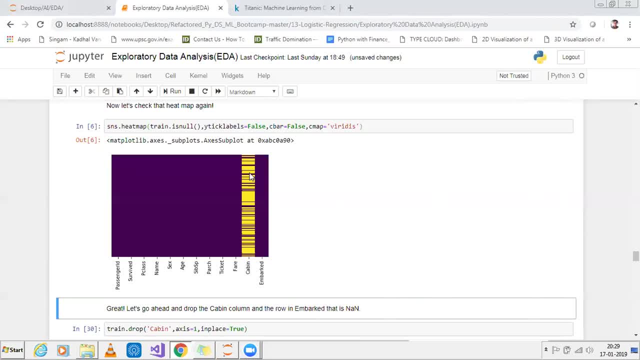 different concept because you know, we need to apply a lot of logic, But right now there are so many null values, I'm going to, I'm going to drop this particular column because, you know, when there is so many null values, you, we have to do a lot of you know. 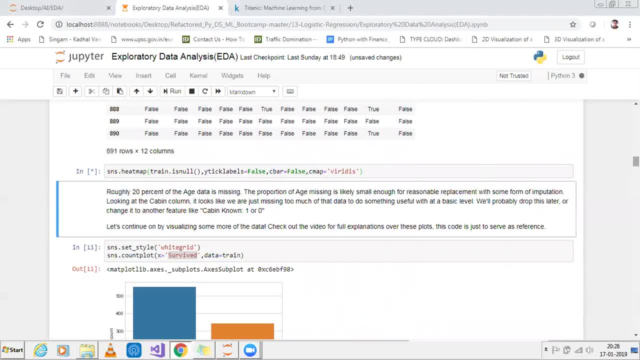 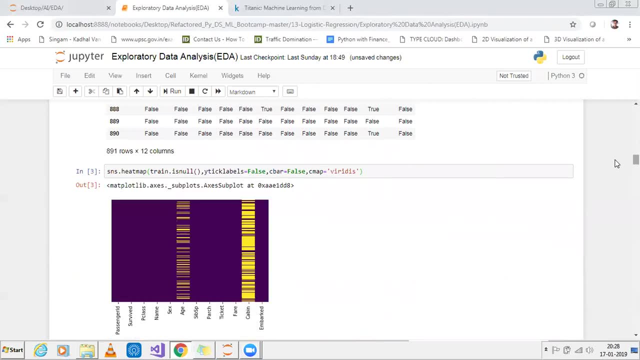 because there I can't actually see my heat map, because after replacing the age column, right At that time you can see that, okay, At that time you can see that you'll be seeing that that age column will never be more blank. 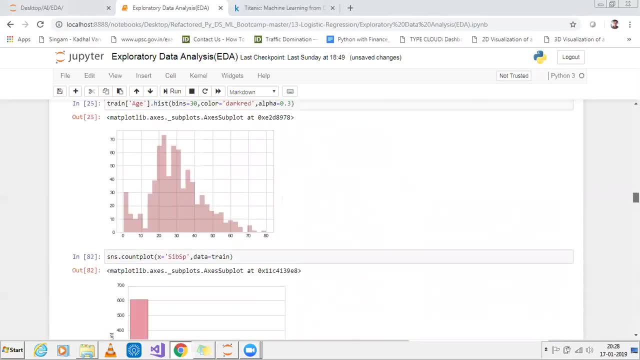 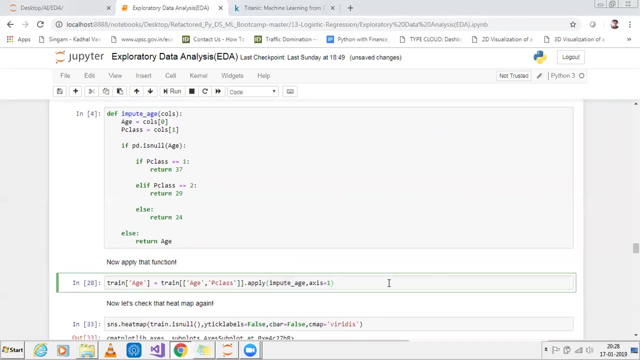 Now you can see that I'm having both this right, And what I'm going to do is that I'll go down over here. you know, I'll go down here. I'll create this function. I'll execute this. okay, my heat map is ready. 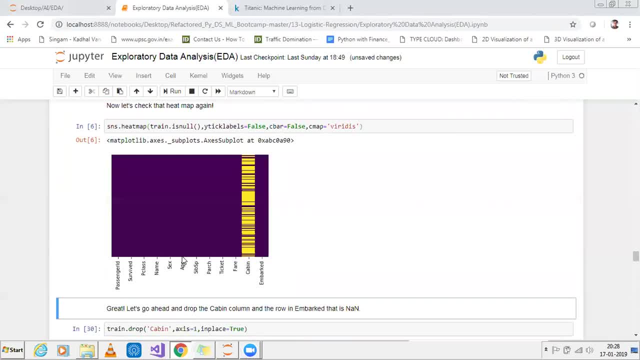 I can't go and check my heat map Now. you can see that my age column has got replaced with the with the values, that is, with respect to the passenger class, So I don't get any yellow lines over here. Now I have to replace this right. 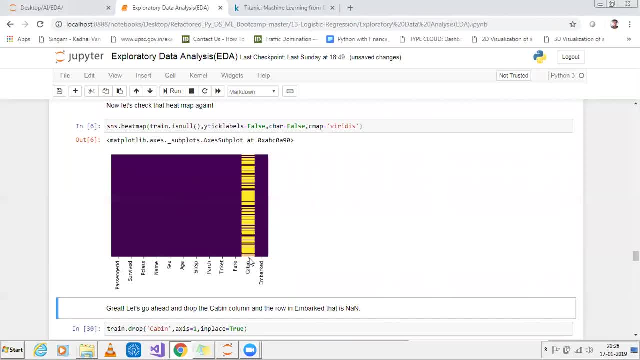 replace this cabin. but the problem with this cabin is that there are many, many, many null values. right, sorry, there are many, many null values. now, if i want to replace something instead of this null values, you know i have to apply some feature engineering, and feature engineering is an. 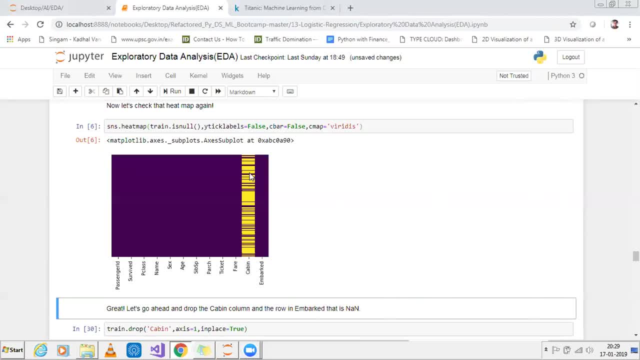 altogether different concept because, you know, we need to apply a lot of logic, but right now there are so many null values, so i'm going to drop this particular column because, uh, you know, when there is so many nan values, you we have to do a lot of- you know- feature engineering to fill. 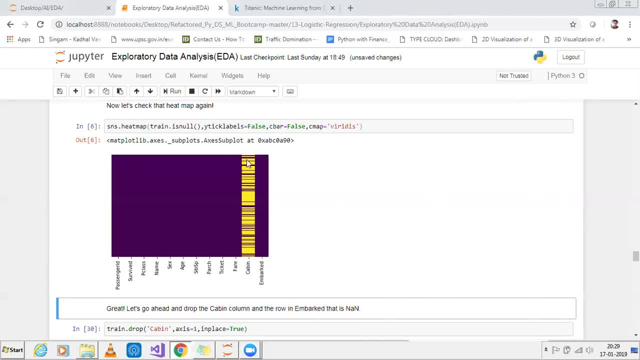 that nan values is something else. okay, this part i'll be taking up in the next video, because it will take more time to explain about this, how i'm going to do the various feature engineering. so what i'm going to do instead of this, i'm going to drop this particular column. 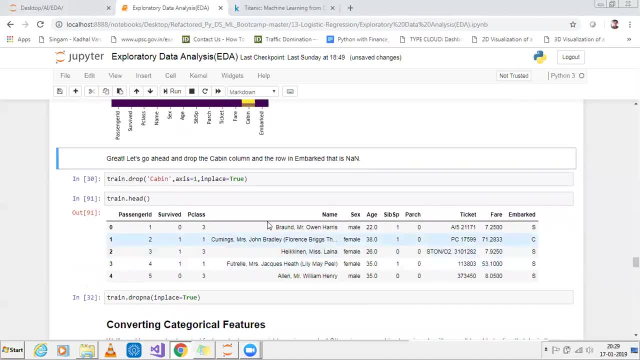 so in the cabin, so i can just use traindrop. cabin x is equal to one. in place is equal to that. so as soon as i drop it now, you can see that my, my column is not present, which is called as cabin. okay, so i'm going to drop this, so you see that. 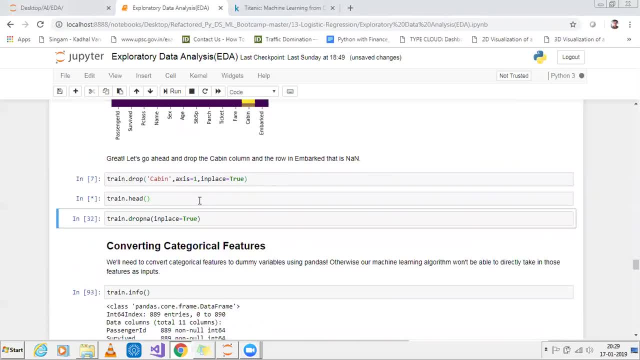 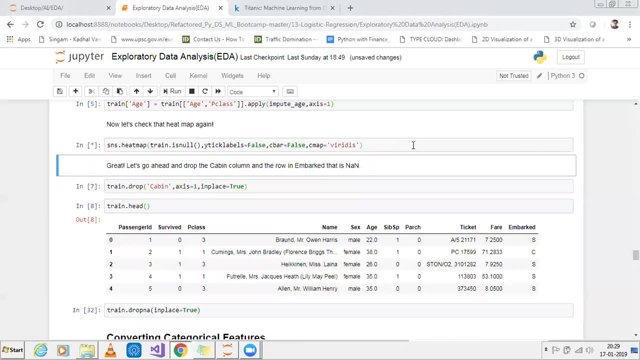 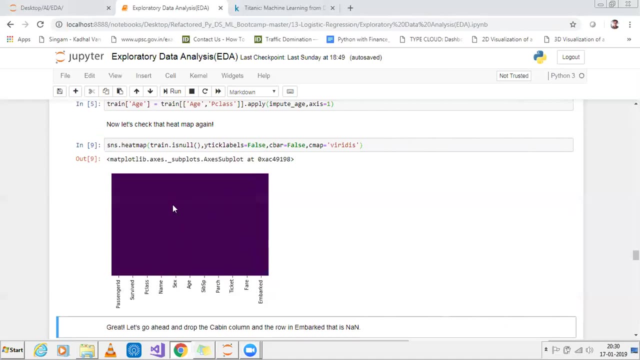 after executing this, and if i go and see my head, my head looks fine. now you see this. if i am again visualizing this particular column, i mean through this bitmap. now i don't have any man values, everything is blank. now, see this? that basically means that we have successfully handled all the 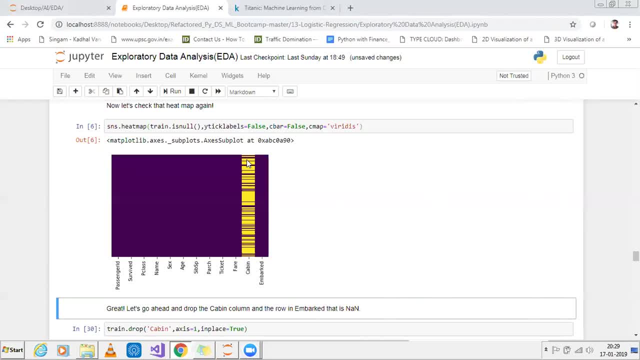 feature engineering to fill the null values with something. OK, this part I'll be taking up in the next video, because it will take more time to explain about this, how I'm going to do the feature engineering, So what I'm going to do instead of this, I'm going to drop this particular column. 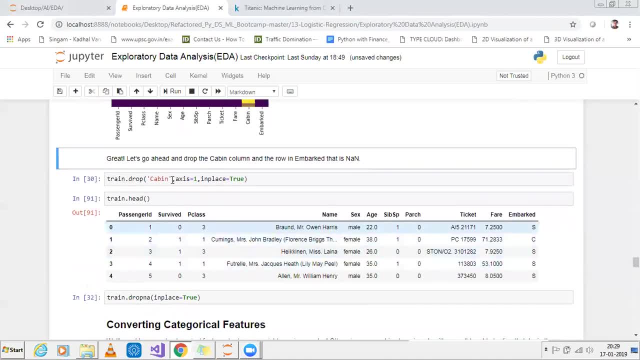 So in the cabin I can just use traindrop. cabin axis equal to one, in place is equal to two. So as soon as I drop it now you can see that my column is not present. It is called a cabin. OK, so I'm going to drop this. 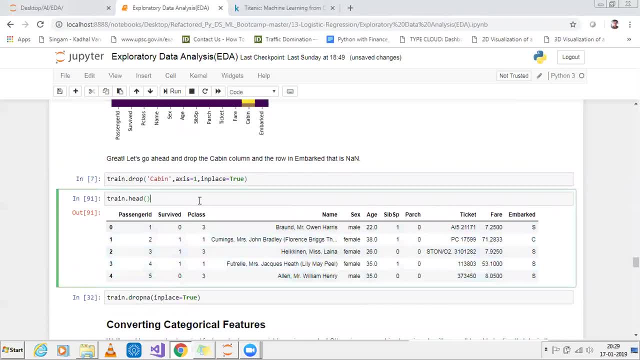 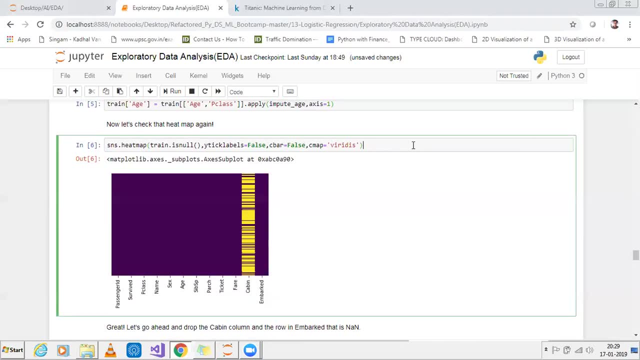 So you see that after executing this, and if I go and see my head, my head looks fine. Now you see this. If I'm again visualizing this particular column, I mean through this bitmap. now I don't have any null values, everything is blank. 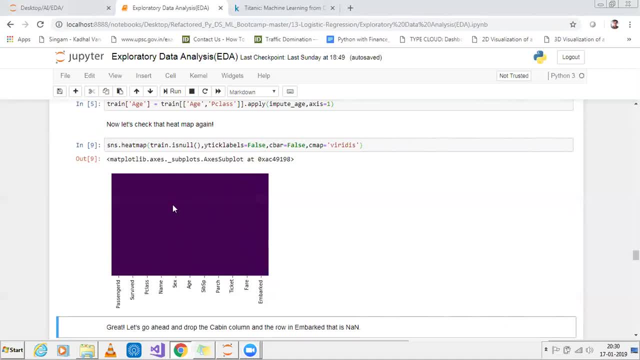 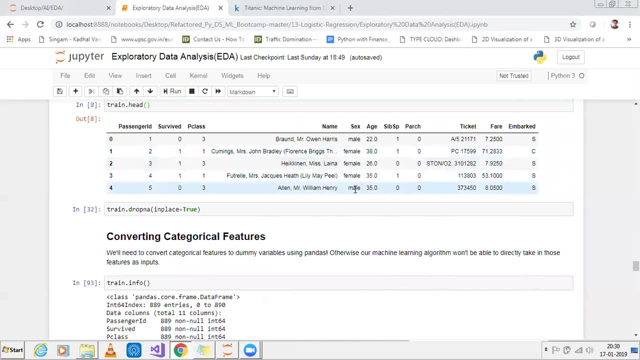 Now I see this. That basically means that we have successfully handled all the null values. OK, now, with respect to this, you can see that this is my complete data. Now, when I see, when I'm seeing this particular data, you know. 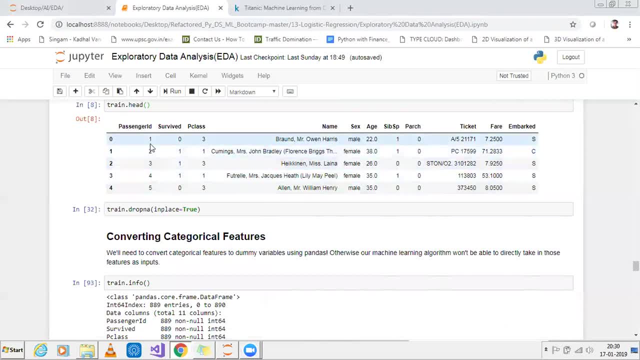 there's some information like passenger ID. because passenger ID is not required because there's just a unique ID name is not required, OK. Similarly, a ticket is also not required because ticket does not play a very big role in this, OK. so what we are going to do is that, first of all, 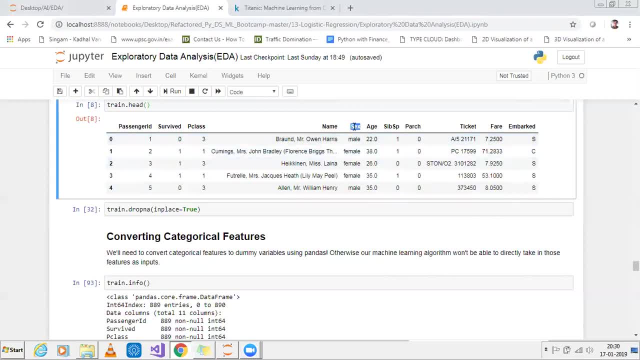 you know we are going to consider some of the categorical features like sex. OK, in this sex you can see that I have two categories, So this has to be represented in some integer format before I pass to the model. OK, so I'm going to handle this particular. 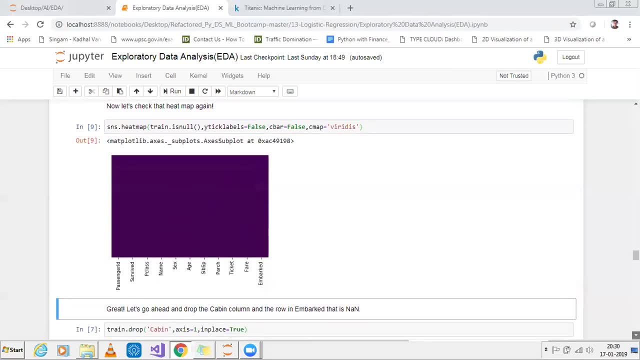 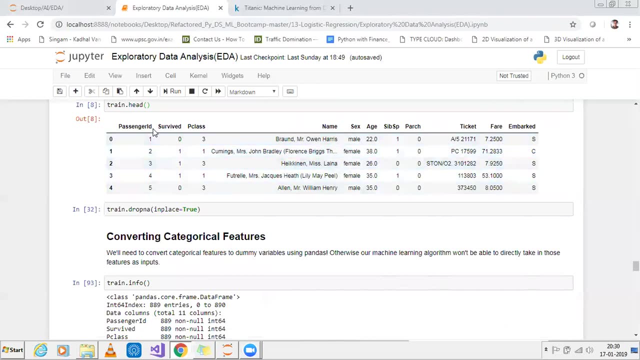 man values. okay, now, with respect to this, you can see that this is my complete data. now, when i seen, when i'm seeing this particular data, you know there's some information like passenger id, because passenger id is not required because there's just a unique id name is not required, okay. similarly, a ticket is also not required, because ticket does not play a. 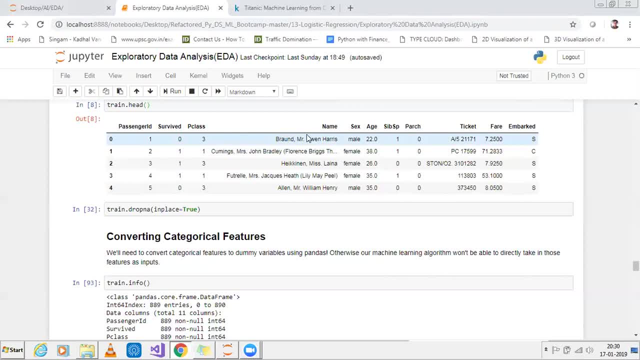 very great role in this. okay, so what we are going to do is that, first of all, you know we are going to consider some of the categorical features like sex. okay, in this sex you can see that i have two categories, so this has to represent it in some integer format before i pass to the model. okay, so i'm going to handle this particular. 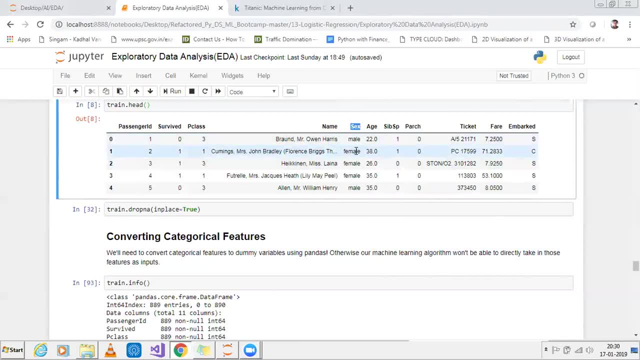 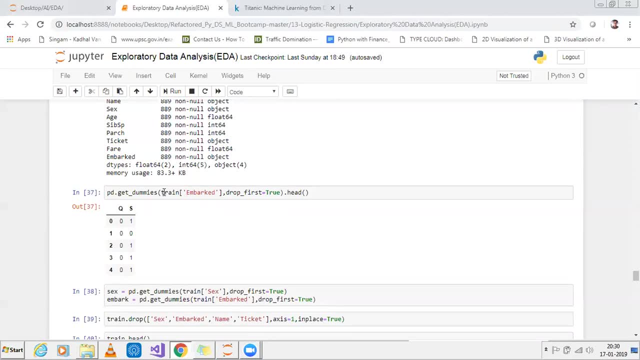 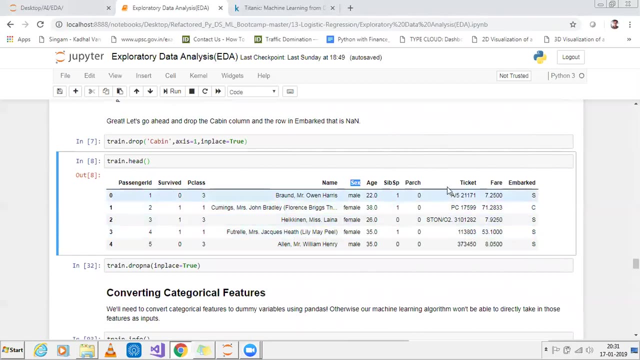 category features by using pandas, by using an inbuilt function called as get dummy. so if you go down and see this, i'm using pdget underscore dummies and okay, i'm also going to apply this get dummies to mbac column- also mbac column. so there are three categories in mbac and two categories. 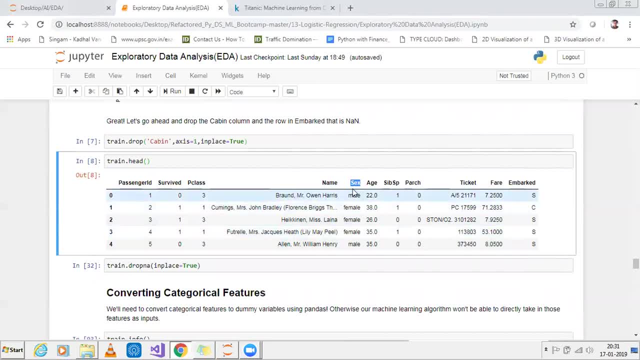 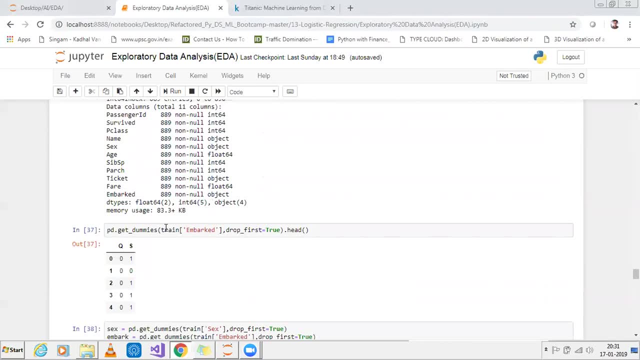 in text. so i'm going to apply the category dummy variable to both the sex and mbac column. so for this, what i'm going to do is that i'm going to go down, i'm going to apply pdget dummies and i'm going to convert. i'm going to take the column which is called as mbac and i'm going to 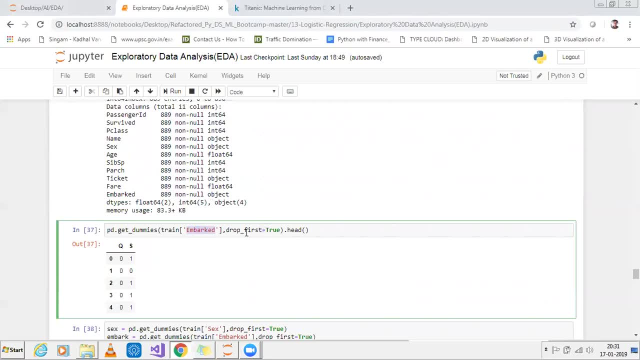 remove the first row. and what does get dummies do is that it converts that many number of categories, that many number of columns. so if i have three dummies, it converts into three categories or three columns. okay, and i can remove the first column because the other two columns can represent. 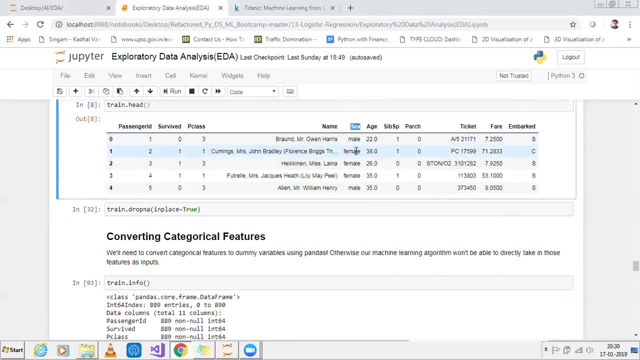 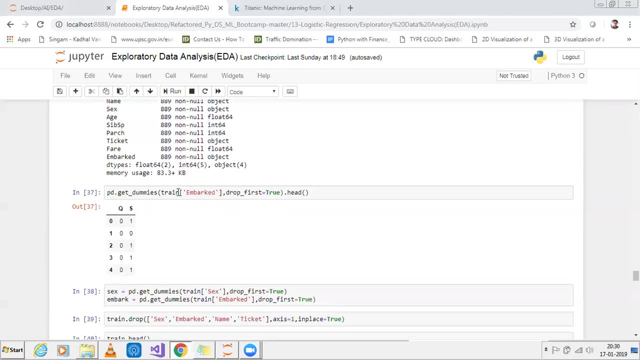 category features by using Pandas, by using an inbuilt function called GetDummies. So if you go down and see this, I'm using pdgetDummies And I'm also going to apply this GetDummies to mbac column- also mbac column. 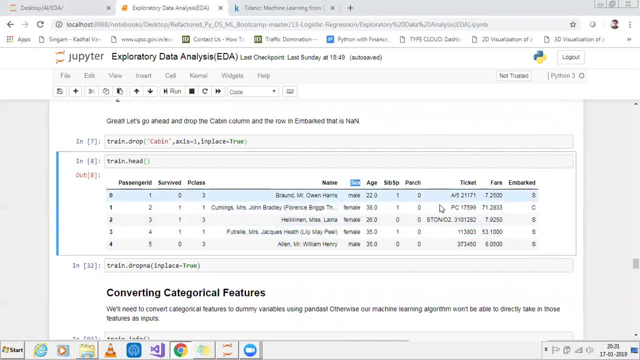 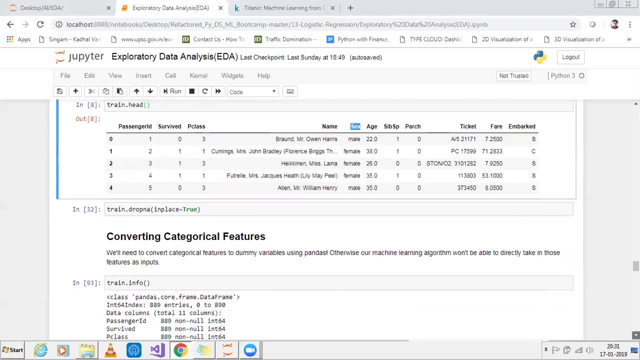 So there are three categories in mbac and two categories in text. So I'm going to apply the category variables to both the sex and mbac column. So for this, what I'm going to do is that I'm going to go down. 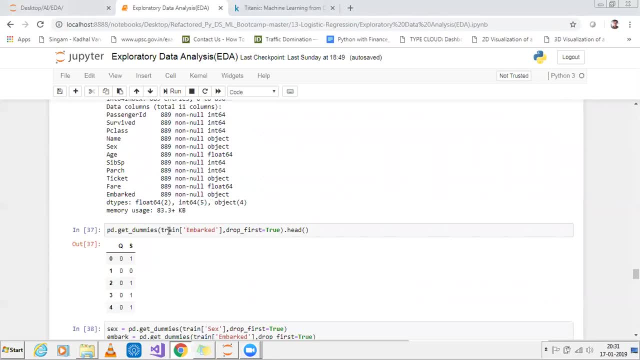 I'm going to apply pdgetDummies and I'm going to convert. I'm going to take the column which is called as mbac and I'm going to remove the first row. And what does getDummies do is that it converts that many number of categories. 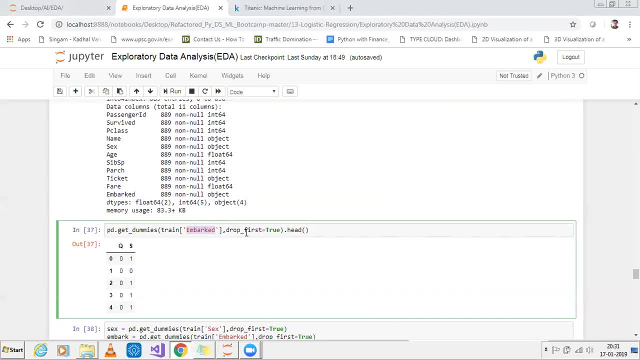 that many number of columns. So if I have three dummies it converts into three categories or three columns, OK, and I can remove the first column because the other two columns can represent the first column. So what I'm doing is that suppose I had three columns like p, q, s. 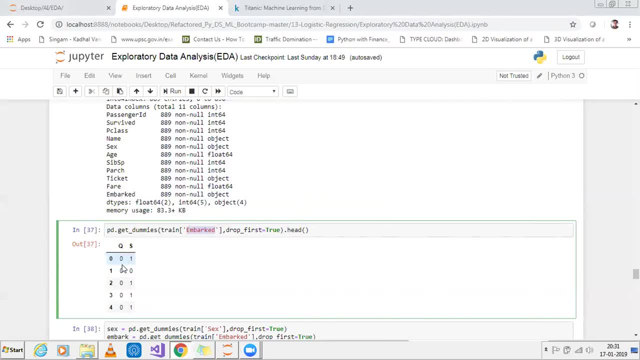 OK, now you know that each and every category gets a unique value, like 0, 1.. 0, 1 is basically for s. OK. 1, 0 is basically for q. 0, 0 will be basically for p. 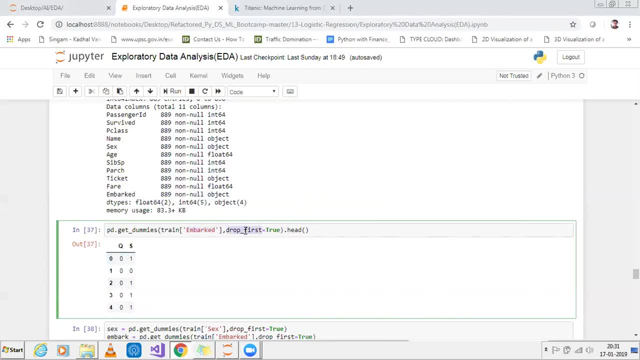 So for that case, what I'm doing is that I'm dropping the first column. I don't require it, And this is basically called as dummy variable trap. OK, so I'm just taking the two columns Similarly, with the help of sex. what I'm doing is that I'll try to convert. 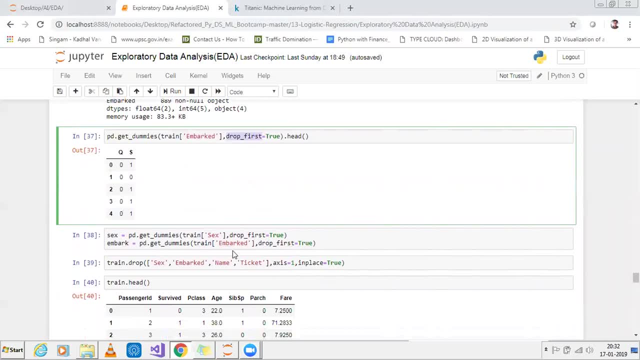 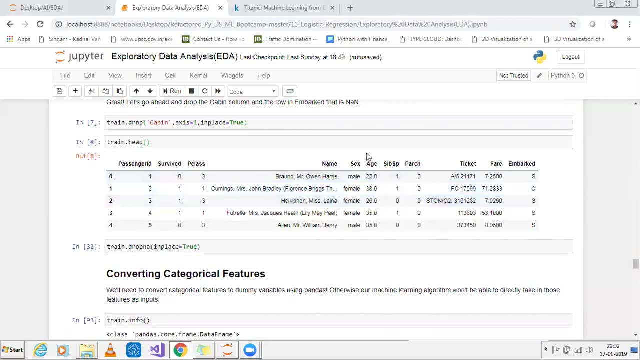 the sex also into dummy variables And drop first is equal to 2.. So, finally, I'm going to drop all the columns that are not required, Like I'll not require the passenger ID, I'll not require name, I'll not require the sex, because I've converted this into category features. 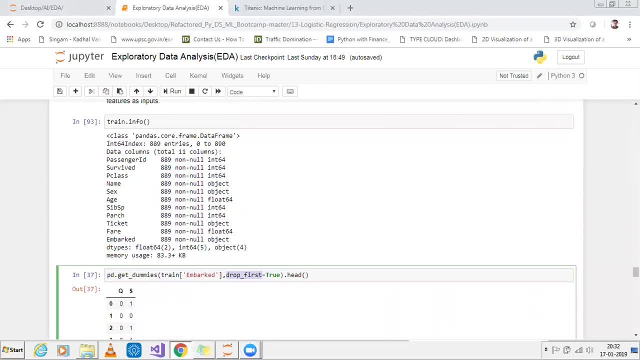 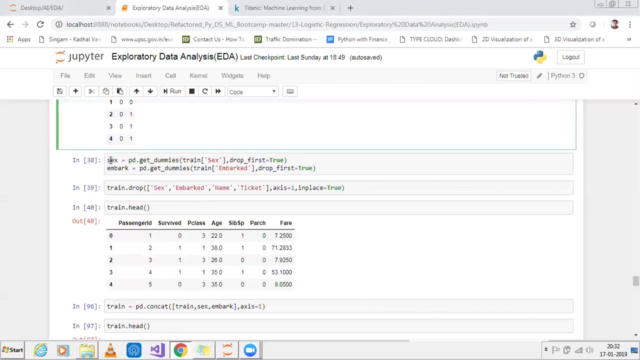 I'll not require mbox also. So here it is. I will go and drop all the columns. I'm dropping sex mbox name ticket because I have created two more columns which is called as sex and mbox in category features. So what I'm going to do. 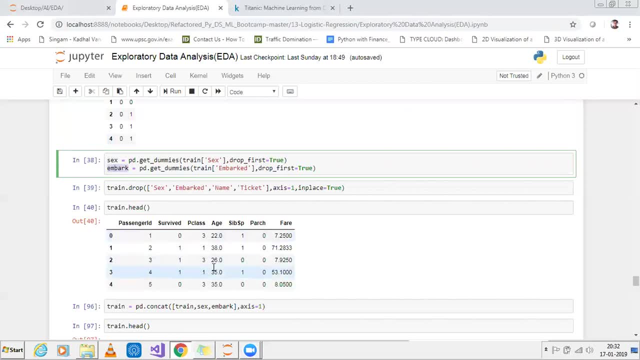 First of all, I'm going to drop it. after dropping it, I'll just see the head part, my head part. You can see that I'm not having sex, mbox name ticket Right, But I have to append the sex column and mbox column because these are the category. 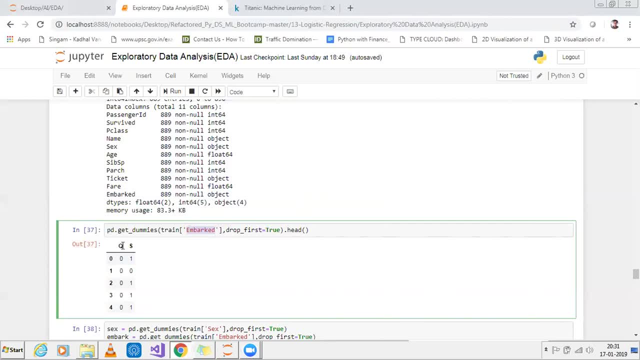 the first column. how i'm saying is that suppose i had three columns like pp, s, okay. now you know that each and every categories gets a unique value, like zero. one zero one is basically for s. okay. one zero is basically for q. zero zero will be basically for p. so for that case, 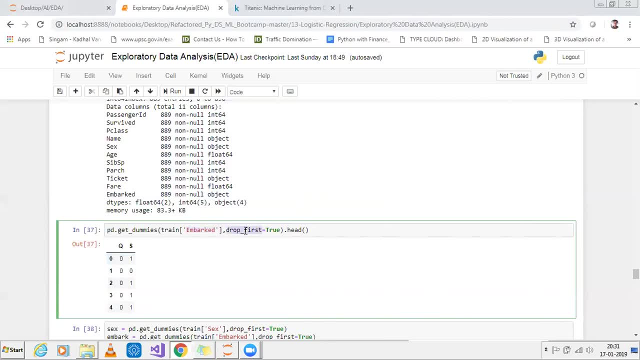 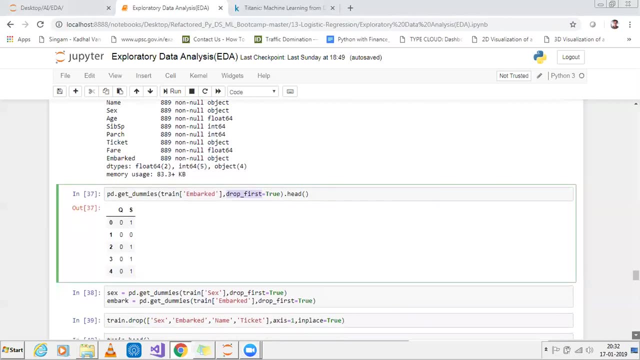 what i'm doing is that i'm dropping the first column. i don't require it and this is basically called as dummy variable track. okay, so i'm just taking the two columns similarly with the help of sex. uh, what i'm doing is that i'll try to convert the sex also into dummy variables and drop first. 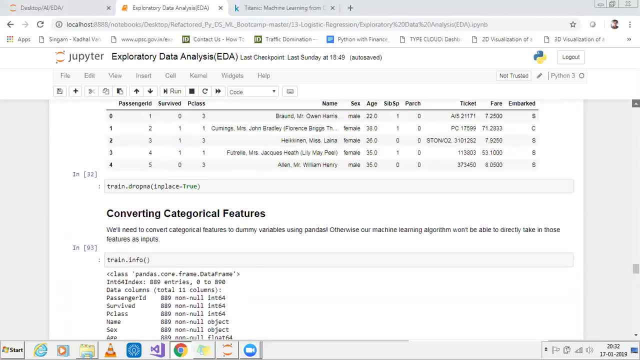 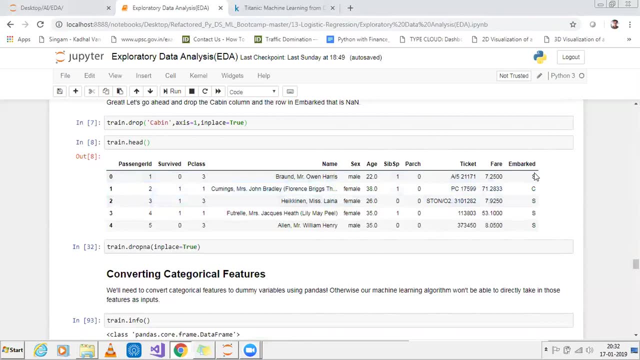 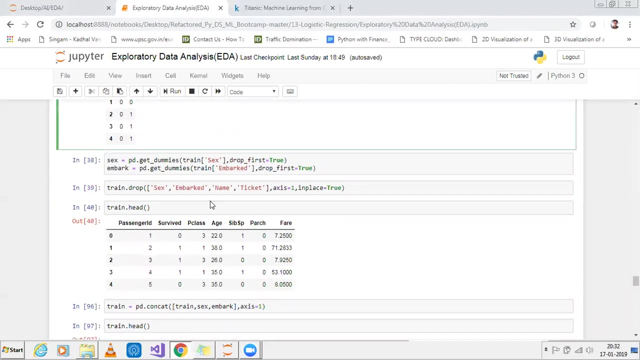 of all, i'm going to drop all the columns that are not required, like i'll not require the passenger id, i'll not require name, i'll not require the sex, because i have converted this into category features. i'll not require mbox also. so here it is. i will go and drop all the columns. 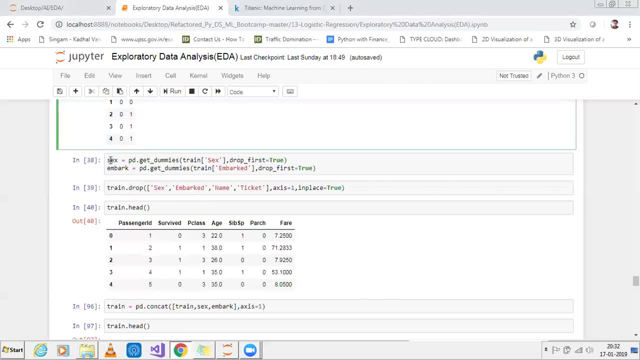 i'm dropping sex and about name ticket because i have created two more columns, which is called in category. so what i'm going to do? first of all, i'm going to drop it. after dropping it, i'll just- you can see that i'm not having sex, mbox, name ticket, right, but i have to append this sex column. 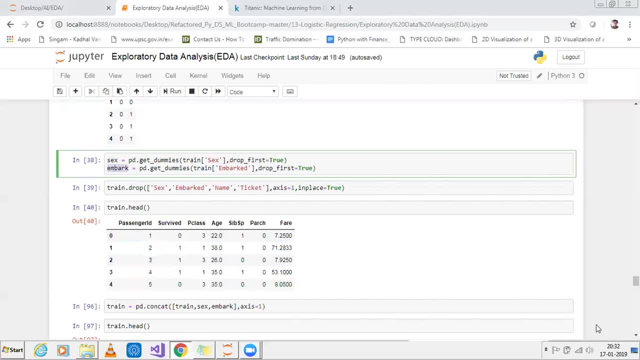 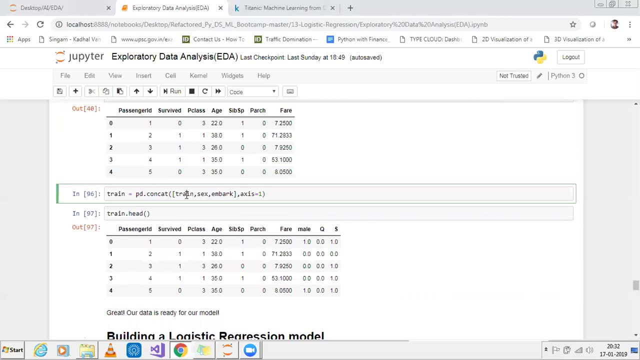 and embark column because these are the category features. so for that i'll be using pdconcat, okay, pdcom, train sex m bar for training data or sex data or which is in my categories features. so you here. you can see that my all my data has got added in the last and i have us. 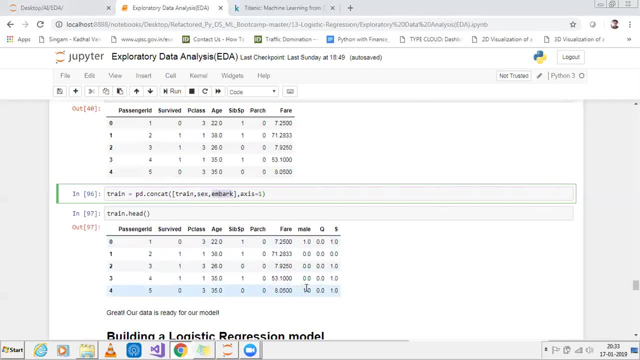 for embed and mail. as for sex data, now my data is ready. this is my whole data. now, from this data, I have to divide this data into dependent and independent features. now you know, survive column is basically my dependent feature, whereas all the remaining columns are my independent. so I'll I'll be applying a logistic regression model first of all. 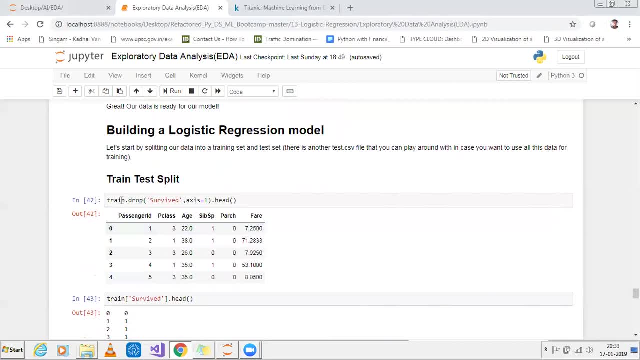 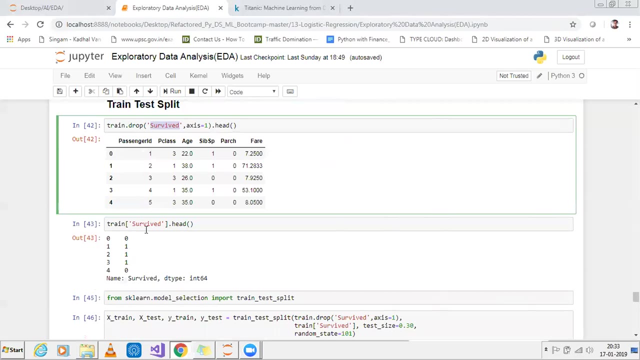 I'll be doing a train test it. but before doing a train test it, I am going to create a train data where I'm dropping the survive column, for survive column is basically my dependent feature. now, this is the complete training data set. okay, and this is my output data set. that is train survive dot head. train of survive is. 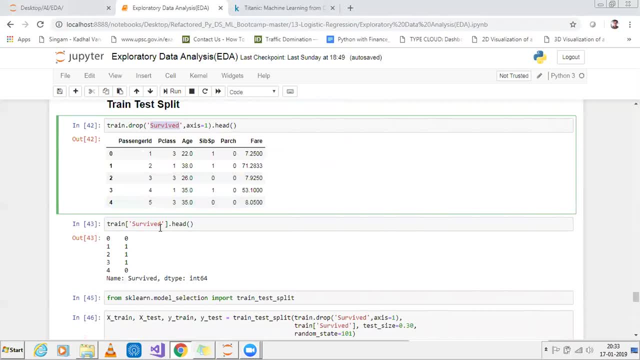 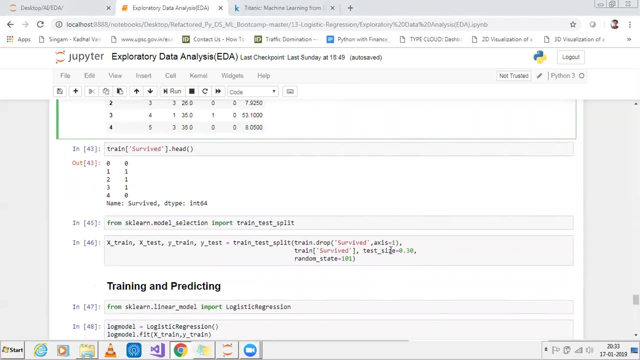 basically my output data set. so considering these two data I am going to do the train test split. so for that I am using sklearn dot model collection and train test split. here in my test size I am taking it as 0.3, that is, 30% will be my test, and here 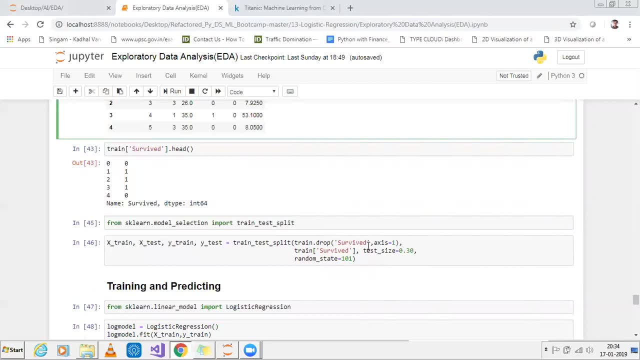 I am just giving my X and Y value. X value is basically train dot drop survive. this X is equal to 1 and my Y value is basically my survive column. after this, I am going to import my logistic regression model if you have not seen the logistic regression. 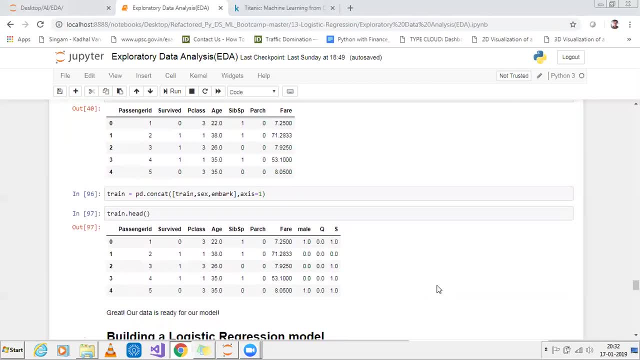 features. So for that I'll be using pdconcat. OK, pdconcat train- sex mbox for training data or sex data, which is in my category features and mbox data. OK, so here you can see that all my data got added in the last and I have UAS for. 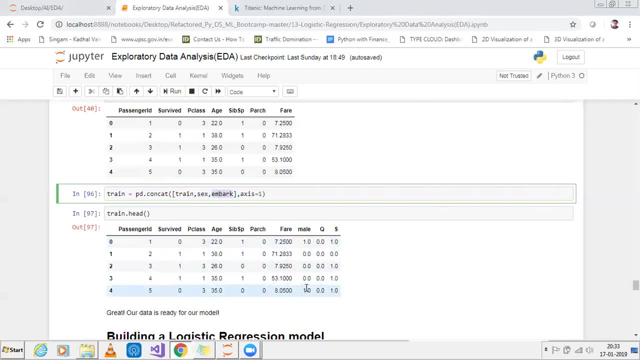 sex mbox and male. as for sex data, Now my data is ready. This is my whole data. from this data, I have to divide this data into dependent and independent features. Now you know, survive column is basically my dependent feature, whereas all the remaining columns are my independent. 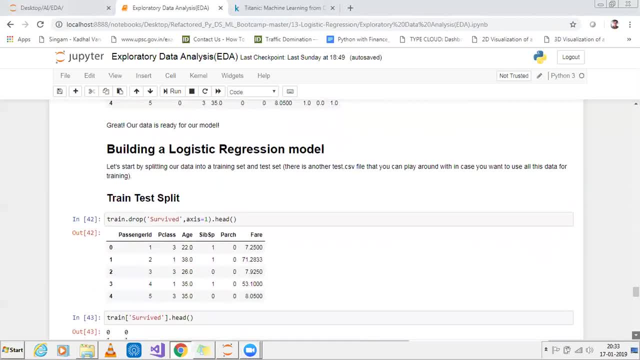 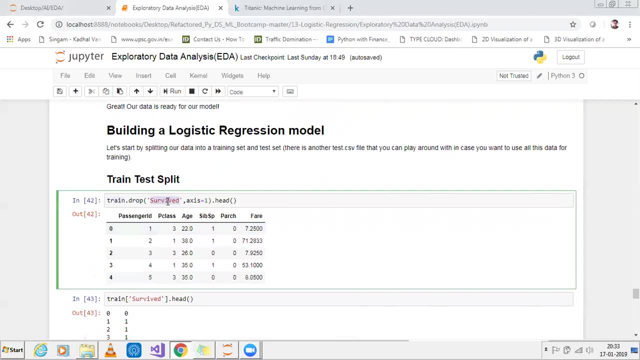 So I'll be applying a logistic regression model. First of all, I'll be doing a train test, But before doing a train test I'm going to create a train data where I'm dropping the survive column. So the survive column is basically my dependent feature. 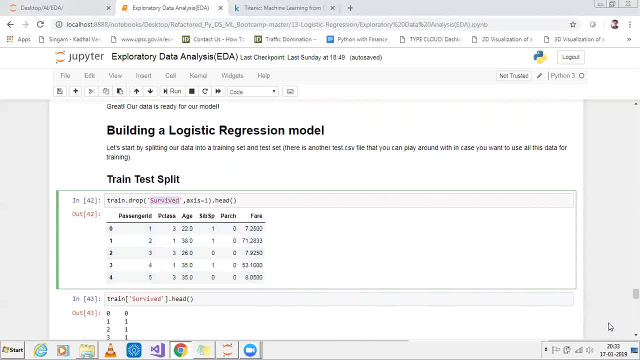 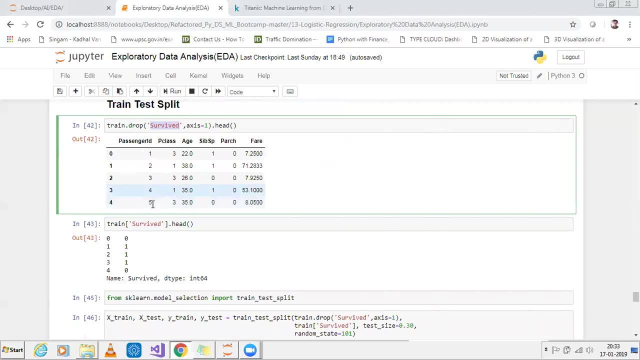 Now this is the complete training data set. OK, and this is my output data set. that is, train survive. Train of survive is basically my output data set. So, considering these two data, I'm going to do the train test split. So for that I'm using sklearnmodel collection and train test split. 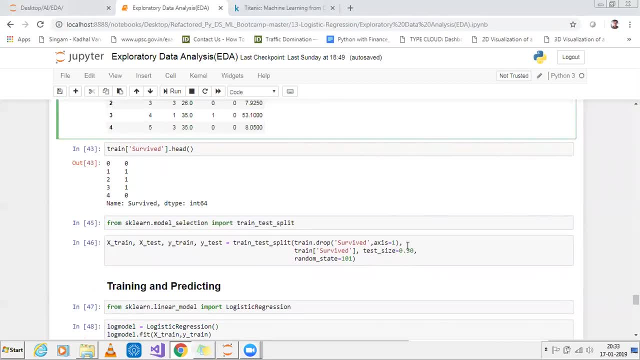 Here in my test size I'm taking it as 0.3, that is, 30 percent will be my test. And here I'm just giving x and y value. X value is basically traindrop survive And my y value is basically my survive column. 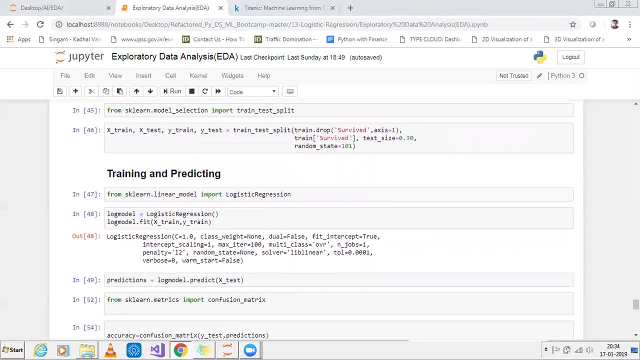 After this, I'm going to import my logistic regression model. If you have not seen the logistic regression explanation, please go and see my video in my playlist in machine learning. There I've actually explained everything about logistic regression for theoretical and practical parts. 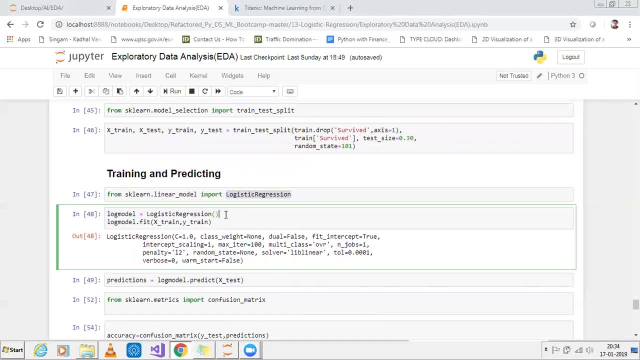 So I'm going to import my logistic regression, I'm going to initialize my logistic regression And then I'm going to apply my fit method where I'm going to pass my x, y, And as soon as I do this, you know, my object will be created. 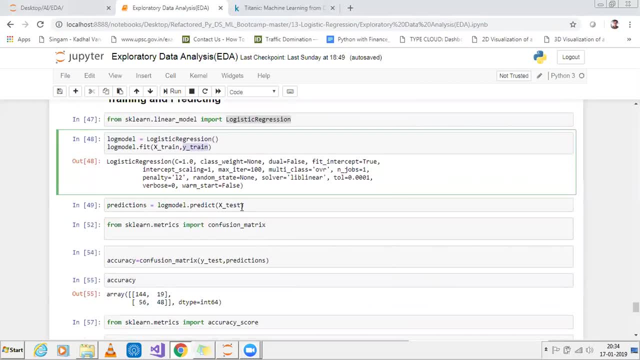 I have to just apply my predict for my x test data. I'll get my prediction. I'll import confusion matrix. If you don't know confusion matrix, please. I've already created videos in confusion matrix about confusion matrix. Again, you just have to go to my playlist there. 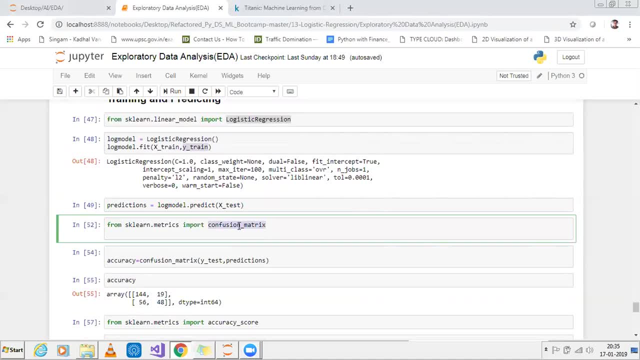 I think this is in data science questions. I've actually put up this video about confusion matrix. Confusion matrix helps you to get the accuracy with respect to your model. Now, based on this, I'm getting you know a 2x2 matrix. the diagonal elements will be your right. 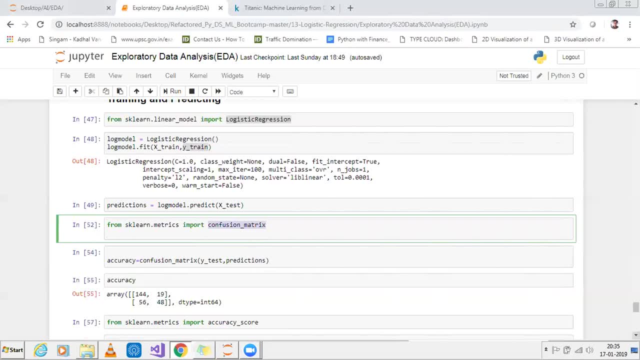 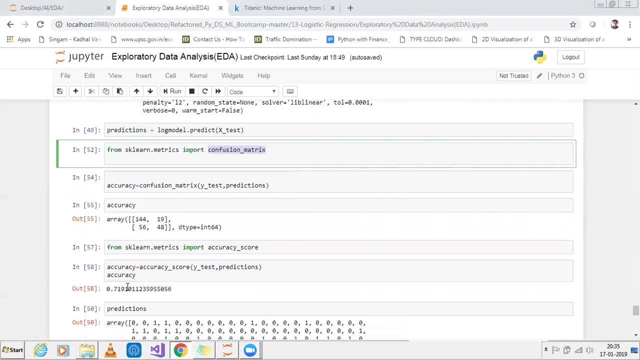 elements and remaining elements will all be your wrong elements. If I go and see my accuracy score, there is somewhere around seventy one point nine percent. So seventy one point nine percent is just by applying a simple logistic regression. If I go and apply some more complex, 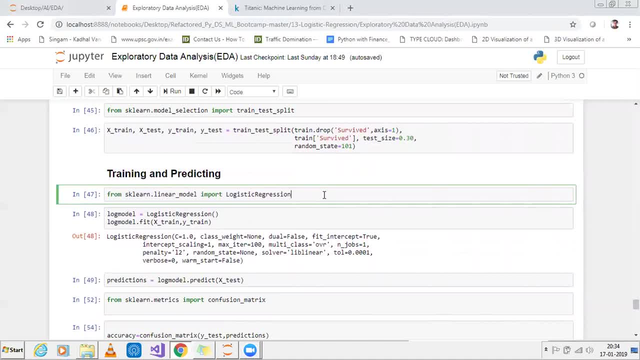 explanation. guys, please go and see my video and log in my playlist in machine learning. there I have actually explained everything about logistic regression for theoretical and practical part. okay, so I am going to import my logistic regression, I am going to initialize my logistic regression and then I am going. 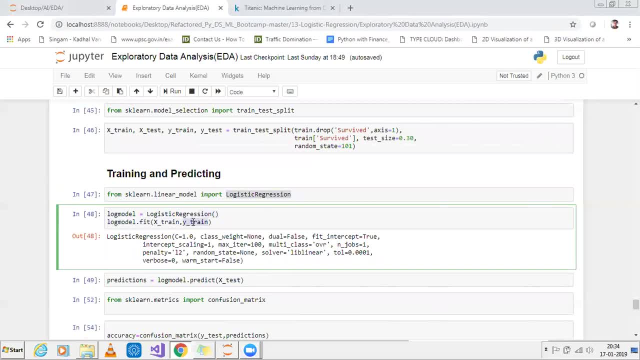 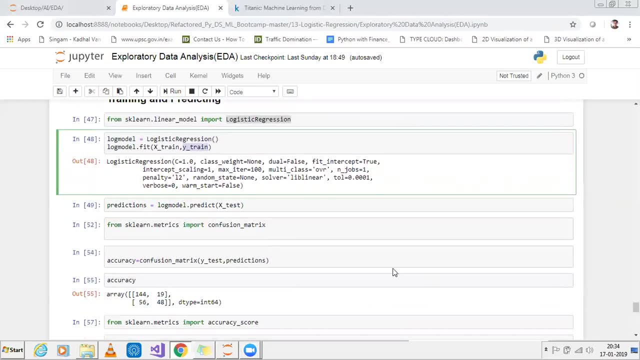 to apply my fit method where I am going to pass my X train and Y train. so as soon as I do this, you know my object will be created. I have to just apply my predict for my X test data. I will get my prediction. I will import confusion matrix if you don't know confusion. 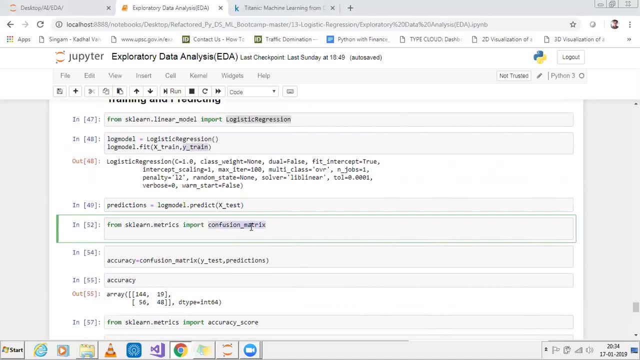 matrix, please, guys. I have already created videos in confusion matrix about confusion matrix again. you just have to go to my playlist there. I think this is in data science in questions. I have actually put up this video about confusion matrix. confusion matrix helps you to get the accuracy with respect to a classification model, so I am going to import my logistic regression. 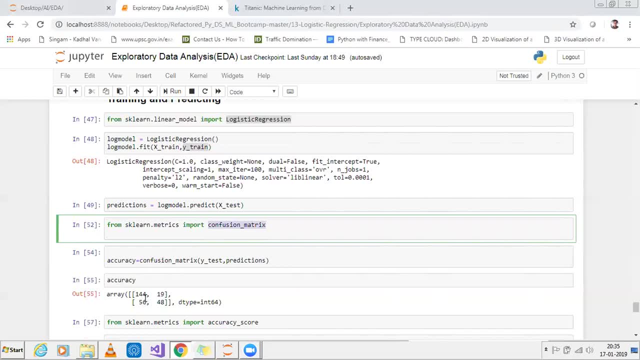 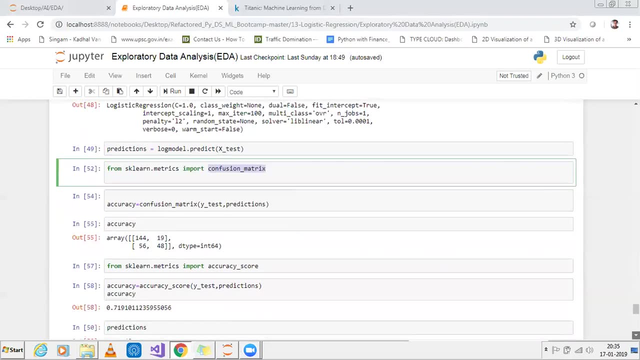 now, based on this I am getting you know, or to the 2 cross 2 matrix, the diagonal elements will be your right element and remaining elements will all be your wrong element. if I go and see my accuracy score, there is somewhere around 71.9%. 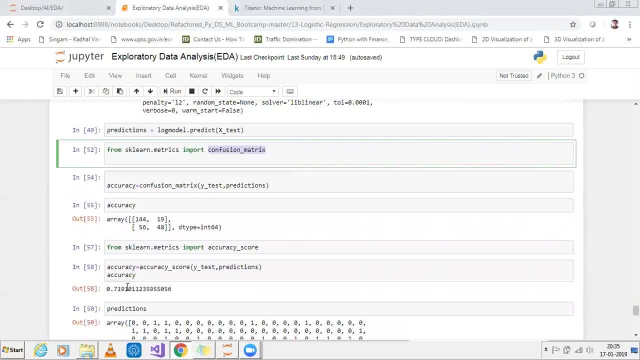 okay, so 71.9% is just by applying a simple logistic regression. if I go and apply some more complex algorithms like random forestization or gboost, I will be getting a very good accuracy now with logistic regression. also I can fine tune this model again. fine tuning part will be displayed in another video where 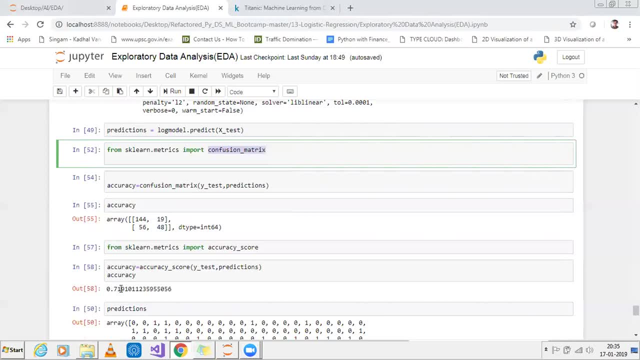 I can improve. I have tried it already and I can improve this 71.9% to somewhere around 87 to 88% by using the same technique. okay, instead of logistic regression, I had tried it with execution. so this is how you can do an exploratory data analysis. you actually 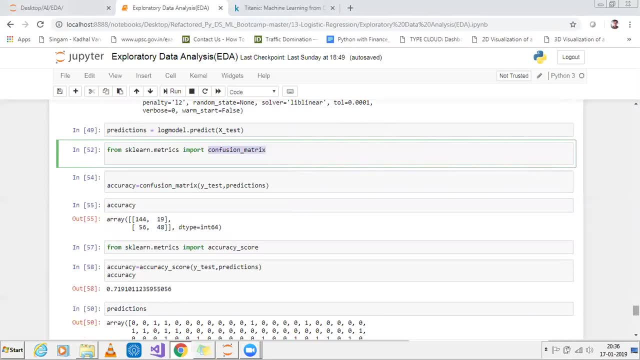 have become a detective. you are able to understand the information from the data even though you don't have a domain knowledge, where you just have some basic knowledge about that particular data. so this is how you can do an exploratory data analysis. you actually can do it for a particular data set. I hope you like the videos. guys, give a thumbs up. 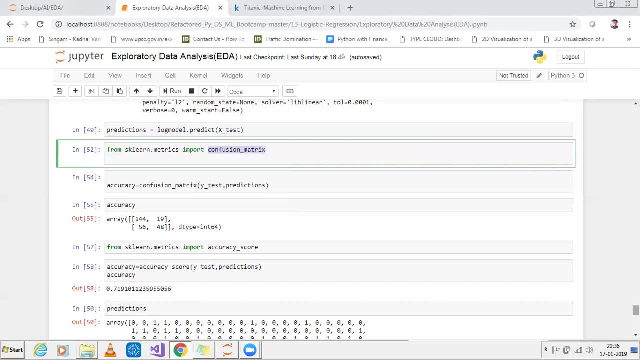 like this video. share with your friends. if you liked this video, comment down with any type of videos that you read you need regarding machine learning and deep learning and please subscribe the channel. share with all your friends who require this kind of help. and one more good news is that in my upcoming videos, I'm going to create a deep learning.